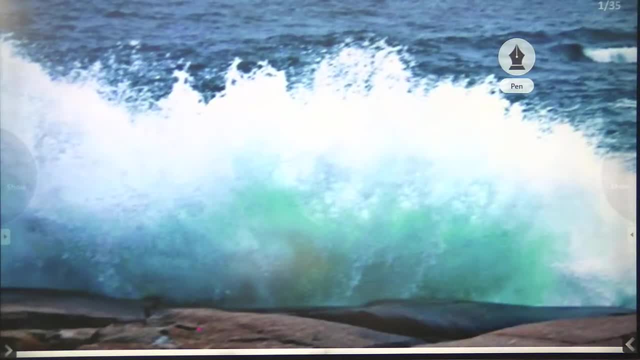 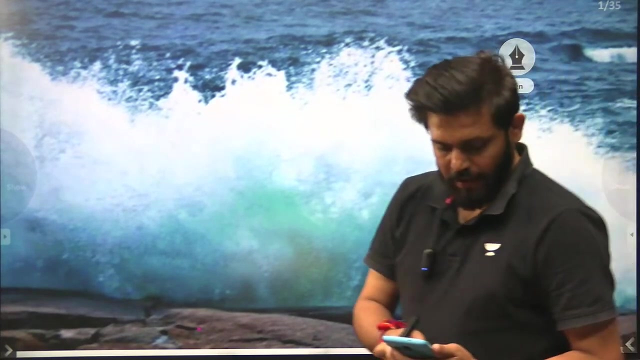 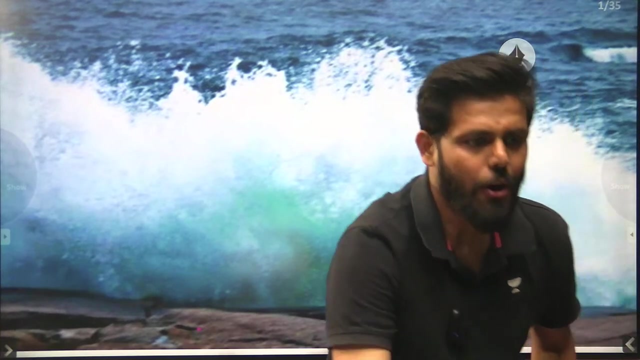 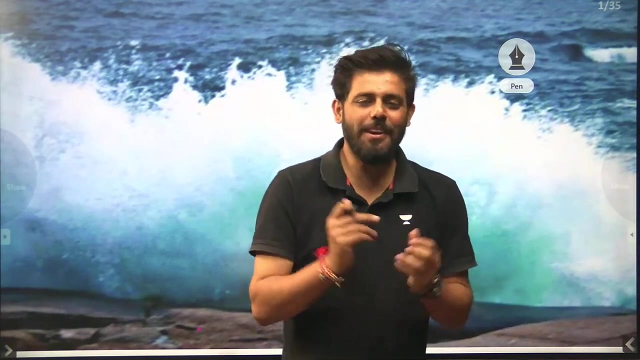 Hello guys, Hello everyone, Hello everyone. So, hello guys, Very, very good evening to all of you. Good evening everyone. How are you all All good? So, guys, today we are going to discuss one of the most 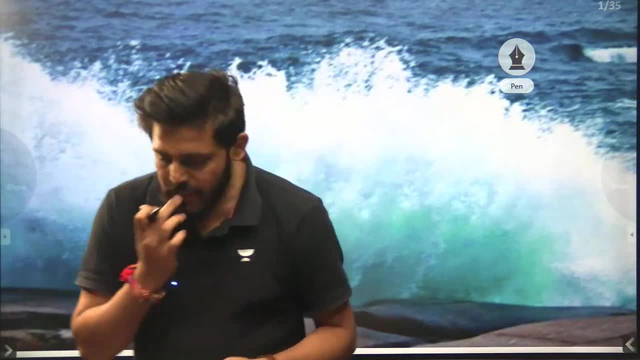 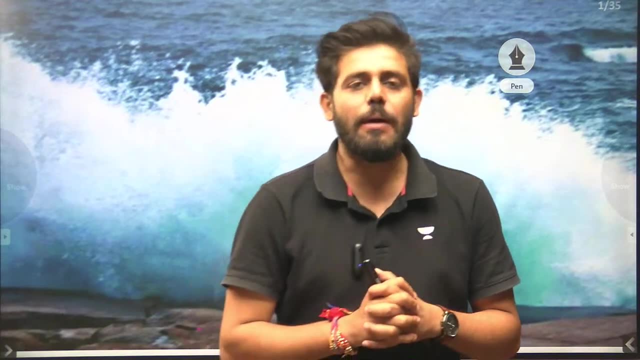 most important topic of oceanography. Today, we are going to talk about tides. What are tides? How do tides come? We will talk about all those aspects. Today we will talk about what is diurnal tides, What are diurnal tides, What are diurnal tides? What are diurnal? 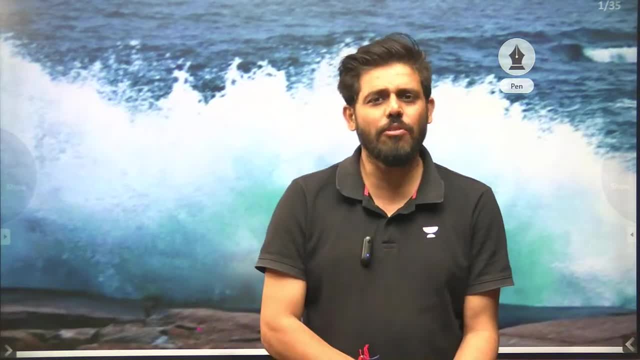 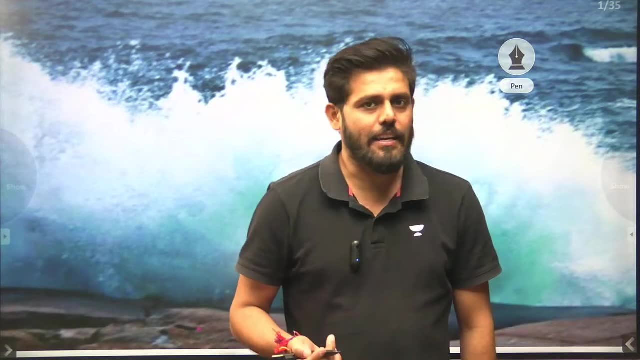 tides. Today, we will talk about what are semi-diurnal tides. Along with that, we will discuss what is spring tide and neap tide. How do tides come And what is the basic difference between tides and waves? What is the difference between these two? How does the movement of 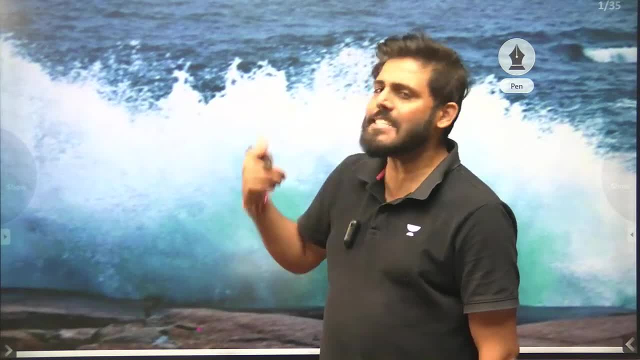 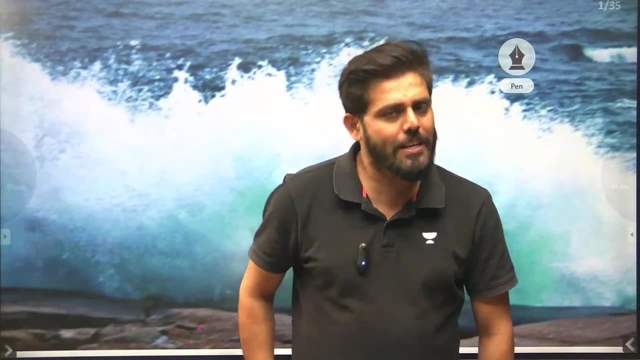 water in our oceans happen. What is the role of the gravitational force of the sun and moon, of these tides? This topic is very important, if I talk from the UPSC point of view. Here there are a lot of tides, There are a lot of tides, There are a lot of tides There. 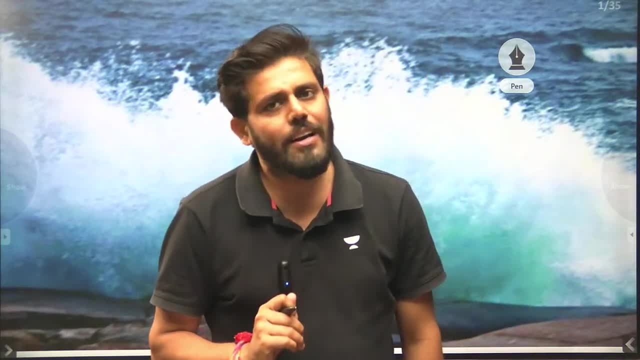 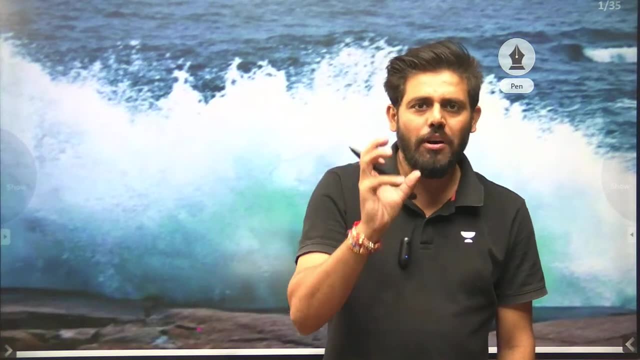 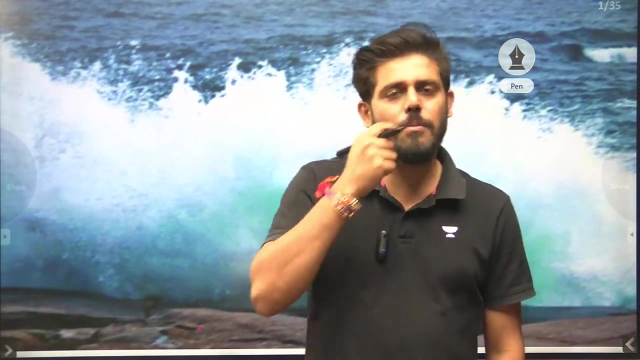 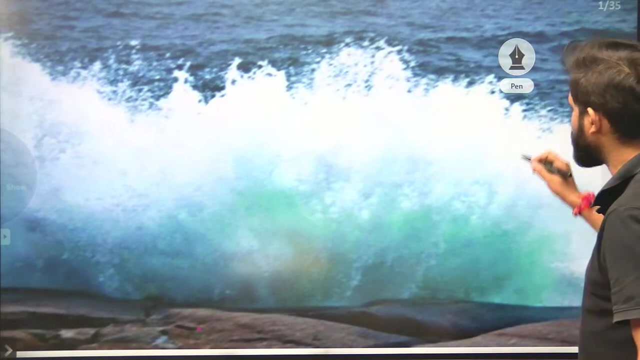 are a lot of swaps in the parameter ANYär, which are generally mathematically Undert坯s. So today we will discuss this topic. Today we will discuss this topic thoroughly, Because our per vie students talk very much about this topic, So we want to keep this topic. 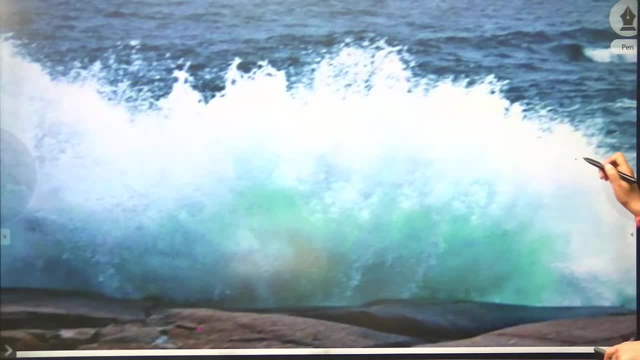 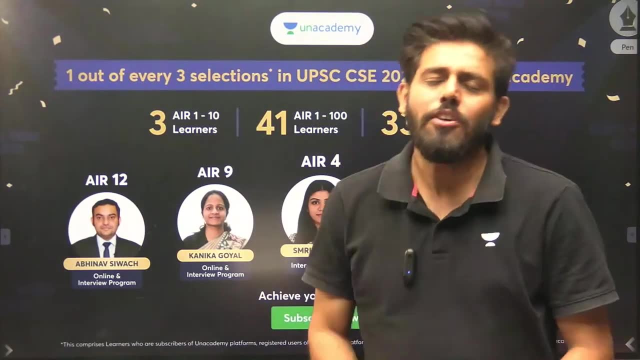 in detail. Okay, so me owe So before starting a session. if I talk about myself, this is Anirudh Malik. I have a teaching experience of more than 6 years. I taught and mentored more than 30,000s of offline. 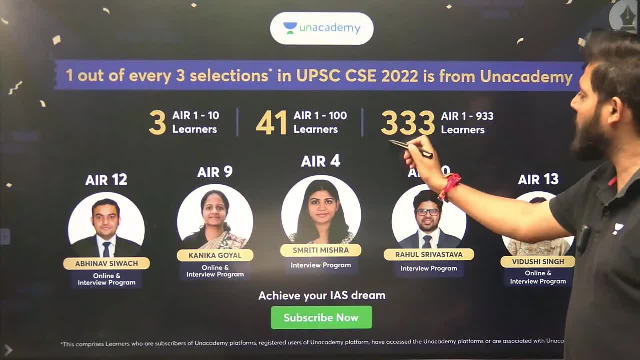 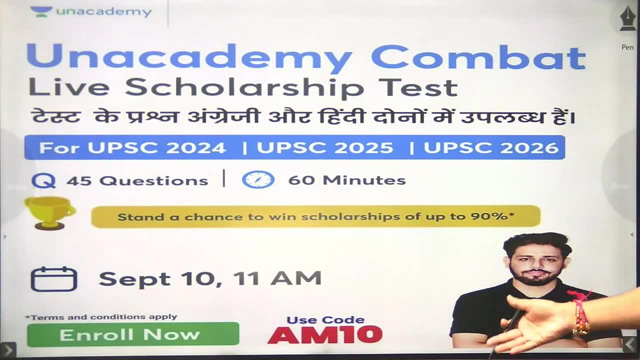 and lakhs and crores of online students. Guys, if we talk about last year, 333 selections were done. there is a reason. everything is in prelims. there is complete coverage. there is an academy scholarship test on 10th of. 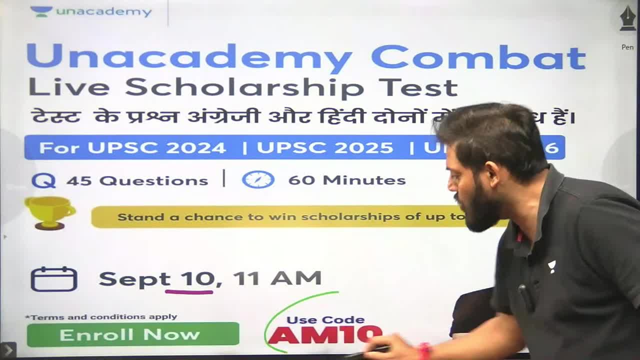 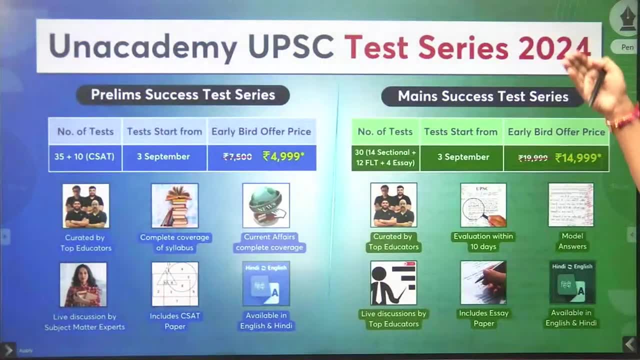 September at 11 am in the morning you can enroll and win a scholarship here for free. You will get a lot of quality questions here. Along with that guys, there is a test series in here of prelims and mains. You will get a prelims in 5,000 and a mains in 15,000. 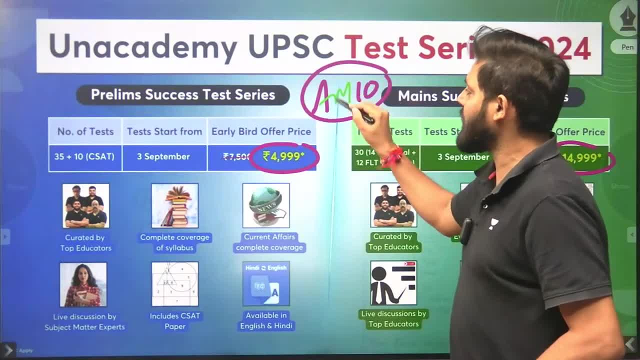 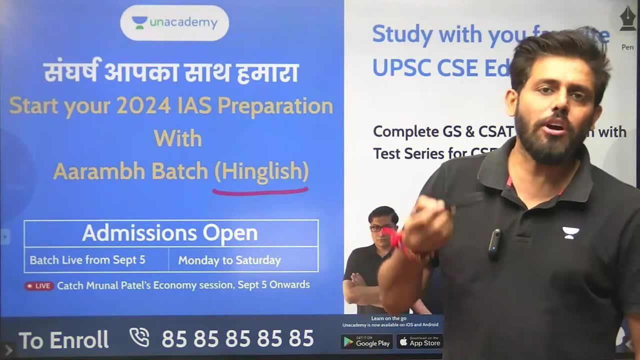 So you can enroll in this test series using AM10 code. you will get a discount here. Along with that, there is an RM batch in English medium. there is a physical geography batch in Mera Plus at 8 am in the morning. if you want to join, then you can do it, and whoever. is a plus student And along with that guys, the test series will be available in English medium. but you can do it in English medium So you can enroll in the test series. So you can enroll in the test series. 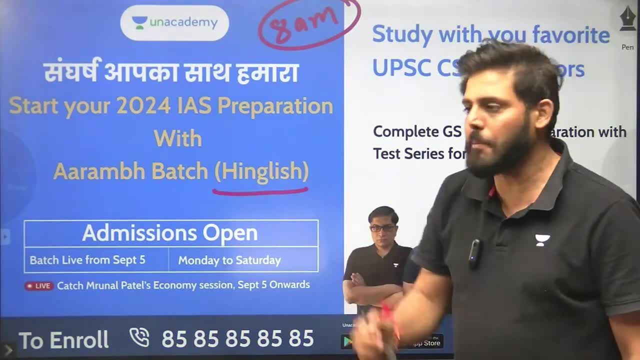 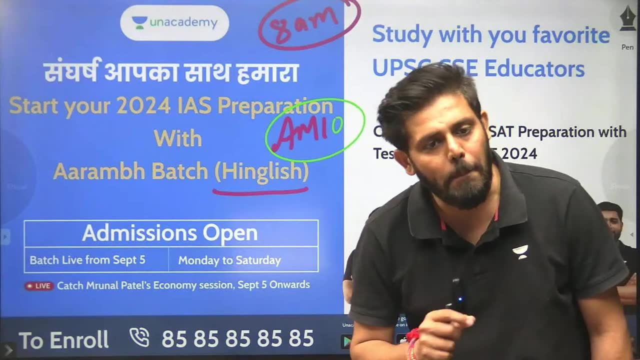 So you can enroll in the test series. I am bringing Indian Geography next month, plus the RM batch, And if you want to take the subscription, then use that code: capital, AM10, discount and mentorship. you will get everything with complete coverage. 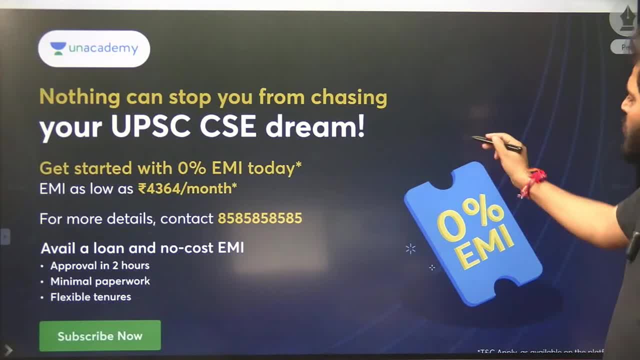 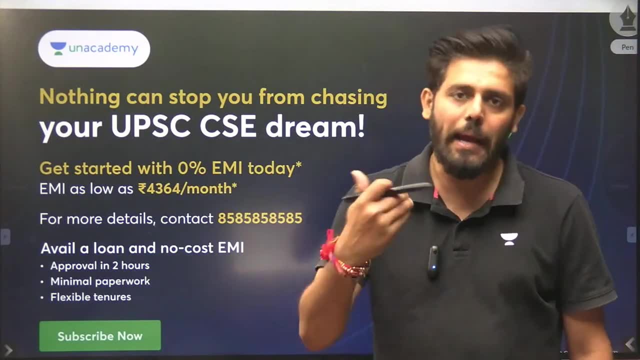 Along with that. guys, if you want to take through loan, then the sales team call comes. just told them that use code AM10, only then you will get mentorship, guidance: what to study, how to study, in which approach to study. 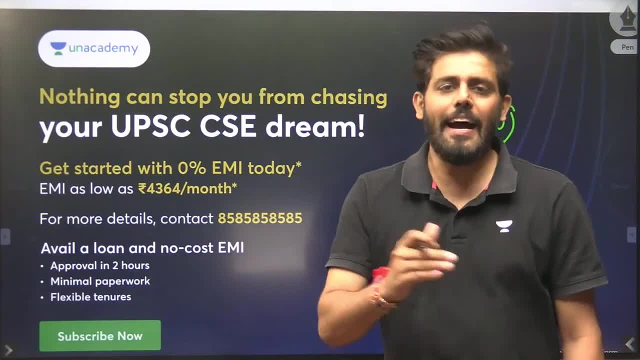 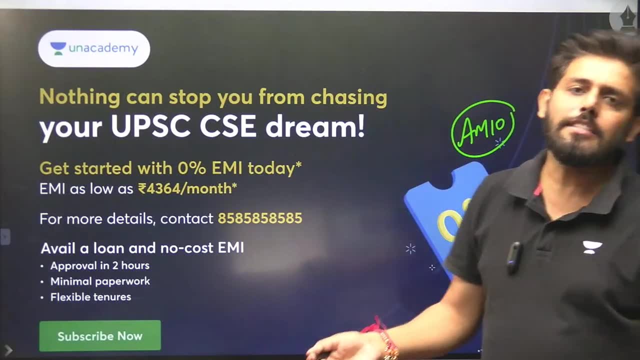 in all those things. you will get help from me. What are the things? how are they? what will happen? you will get complete coverage in all things. Okay, So if you have any doubt regarding subscription, unacademy underscore: Anurudh Malik. 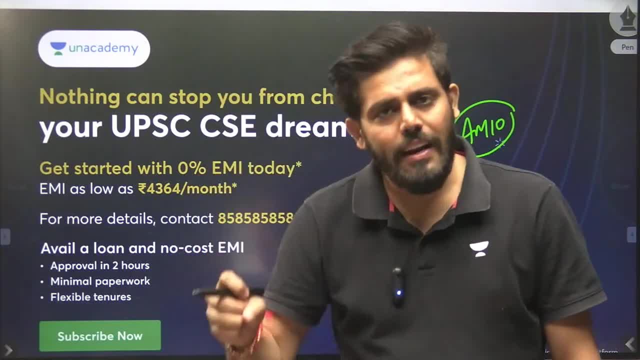 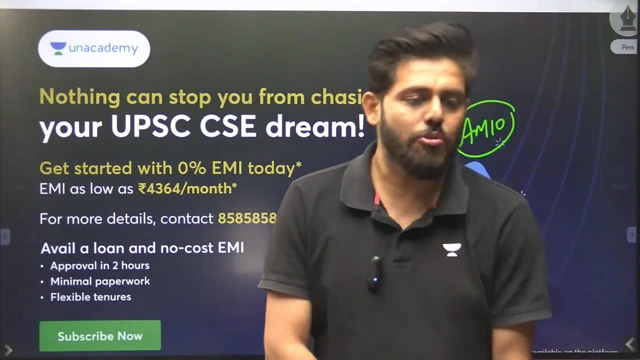 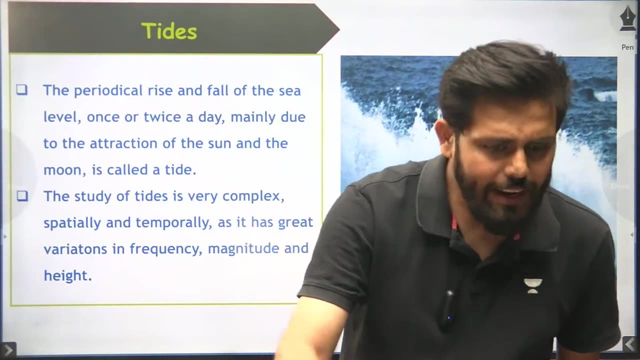 There you will get all doubts contact number plus all my updates class notification on that telegram channel. That is unacademy underscore: Anurudh Malik. Okay, Okay, Let's come quickly about tides. What are tides? How do tides come? 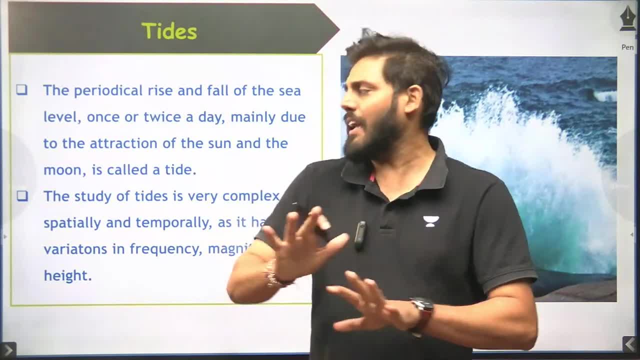 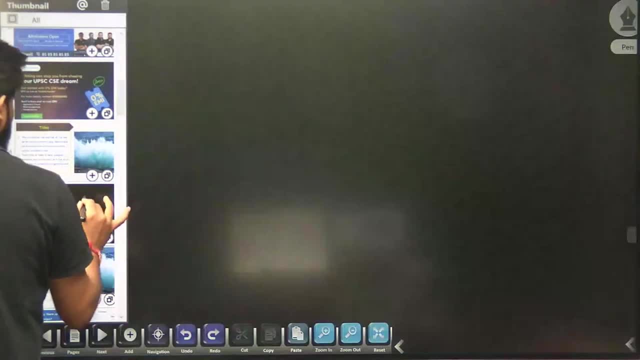 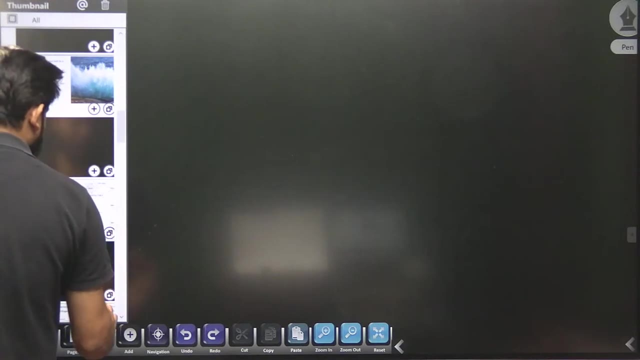 What is the impact of tides? So come quickly. I will leave all these things here and try to explain things in the same old way And I hope so that you stay engaged with things a little bit. You try to understand things, try to understand the concept. 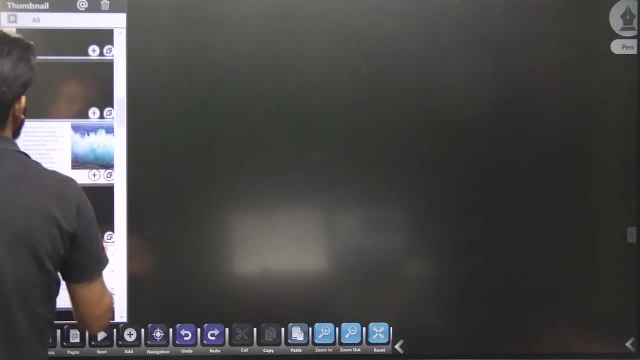 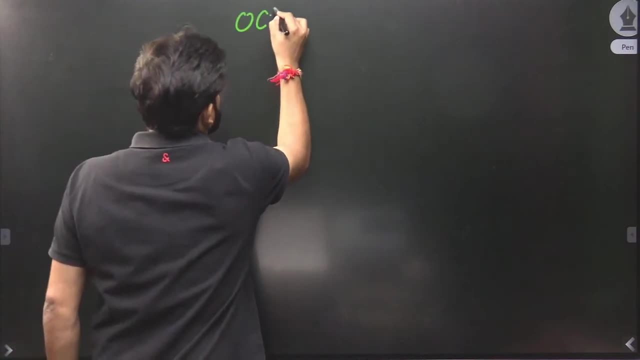 then things will automatically become clear to you. So, without wasting any time, let's start things quickly and we will talk about your first ocean movements: The water in the ocean, the movement of the water in the ocean, how it happens. it is very important to understand that. 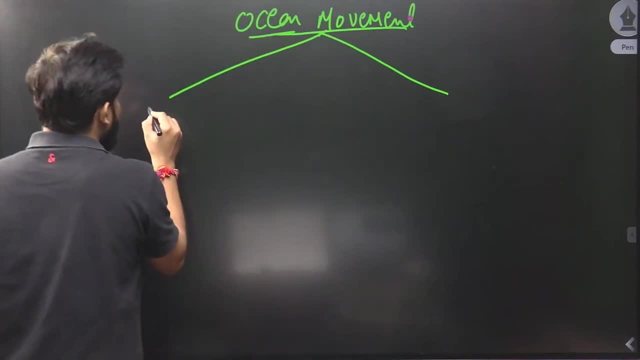 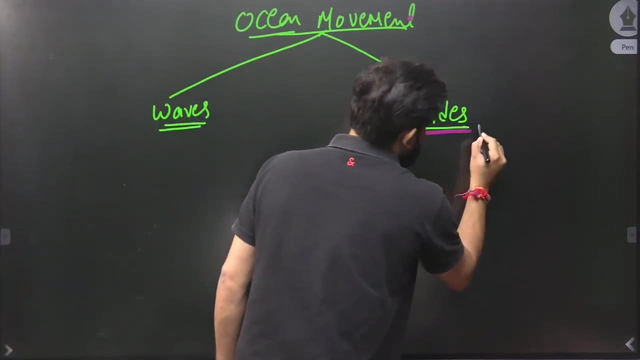 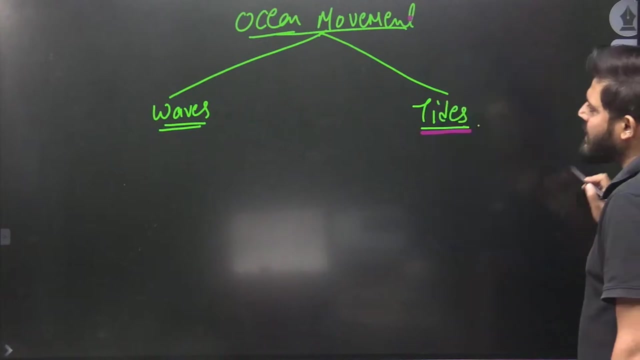 So let's quickly cover it. The first one is waves And the second one is tides. In yesterday's session we will cover ocean waves. Today I will tell you about tides. So what is the difference between the two? What is the basic difference between waves and tides? 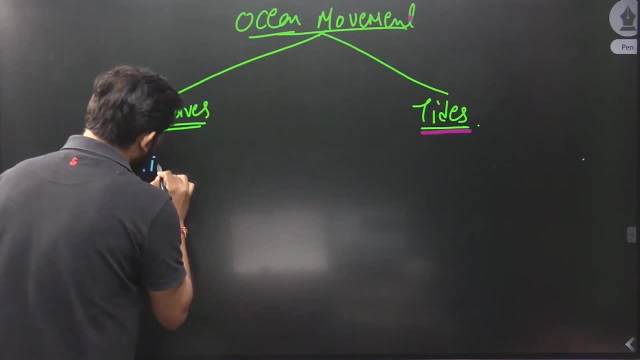 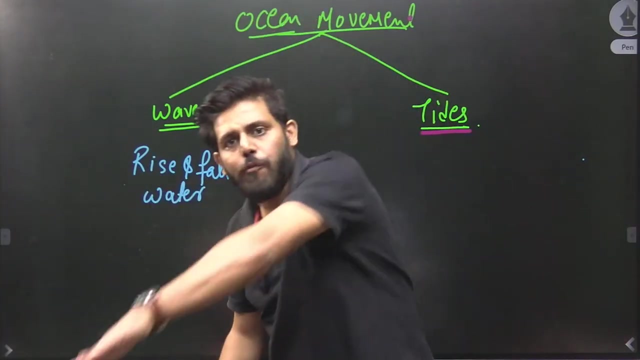 So you have to know that the waves are the rise and fall of sea water. The rise and fall of sea water- The rise and fall of sea water- is the rise and fall of the water in the ocean. The rise and fall of the water is called waves. 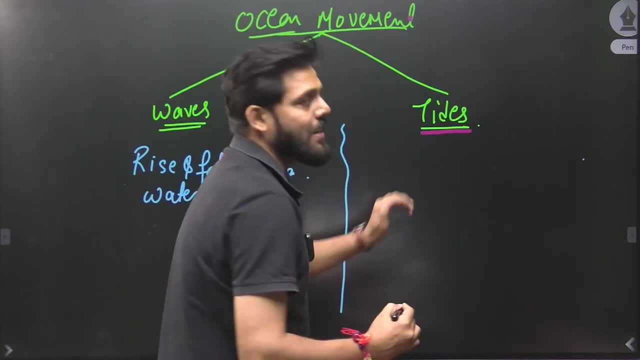 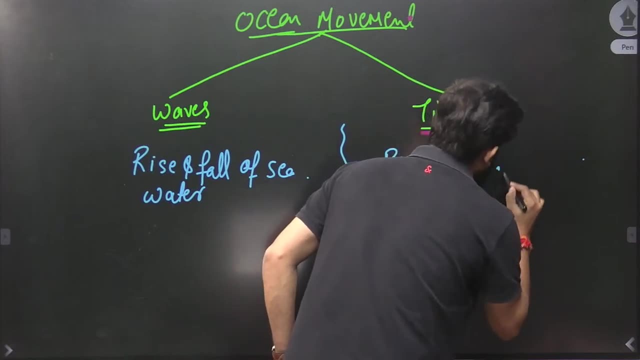 With that, the tides. so, sir, its definition will be different. No, Tides are also called rise and fall of sea water. Here, tides are also rise and fall of sea water, Sir, there is no difference between the two. there will be a little difference, but the point is that because of whom it has happened? 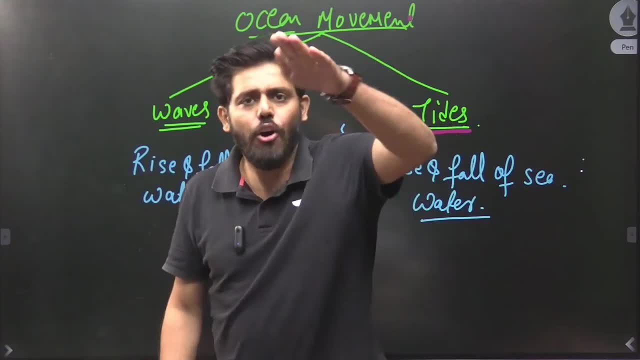 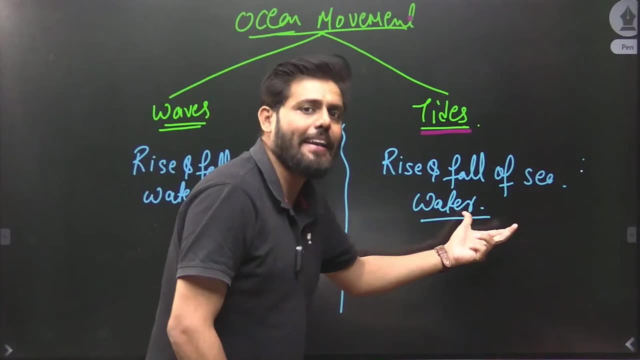 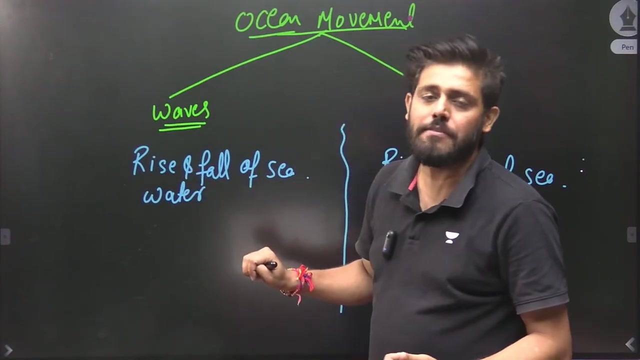 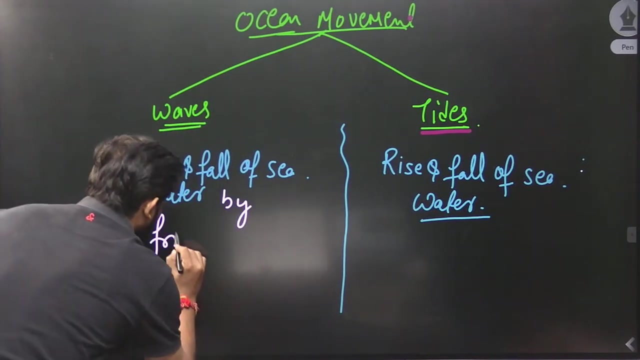 The waves are rising and falling here too. the water is rising and falling in the tides too, but the rise and fall here is due to different reasons, and the rise and fall here is due to different reasons. If I ask you why the waves are rising and falling, you will find rise and falling of sea water is called tides due to the frictional force of the winds. 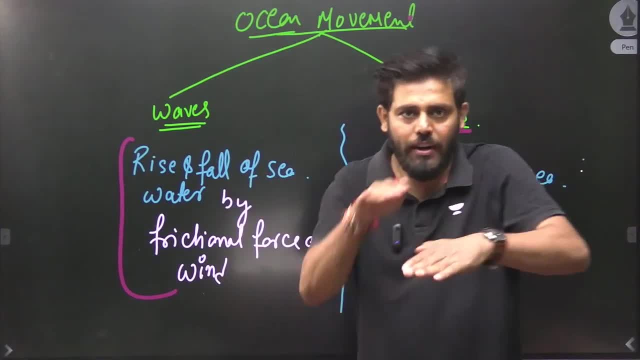 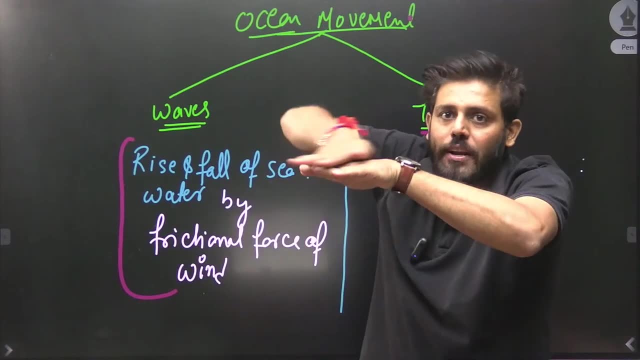 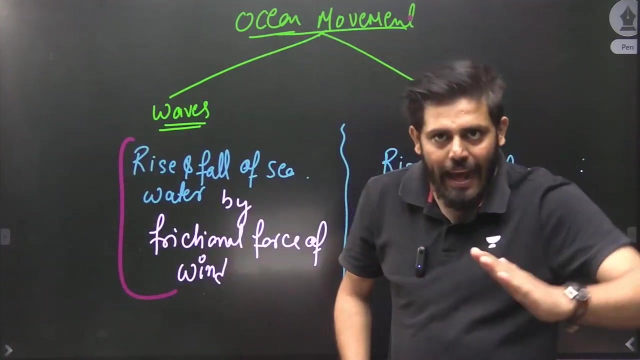 Try to understand. here it is the ocean water, Here is the wind. So when the wind is there, It will apply its force on the water, due to which the water will rise and then fall. This is called waves: Rise and fall of sea water due to the frictional force of wind. 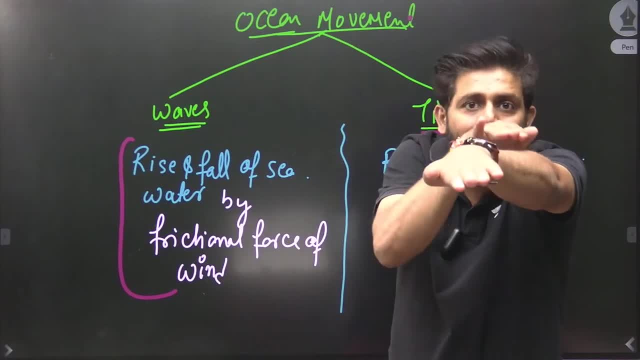 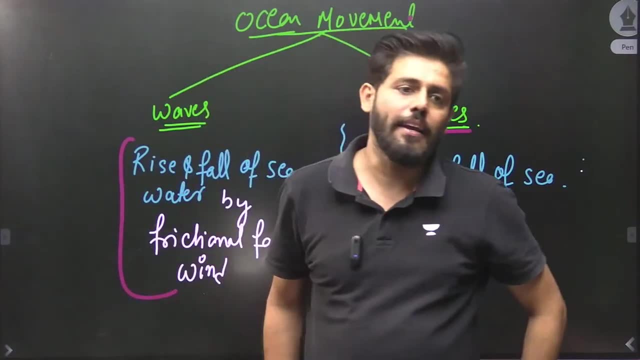 When the wind moves on the water, it will apply a force on the water And due to that force, due to that frictional force, when the water rises and falls, it will be called waves. Did you understand The rise and fall of sea water? due to the gravitational force? 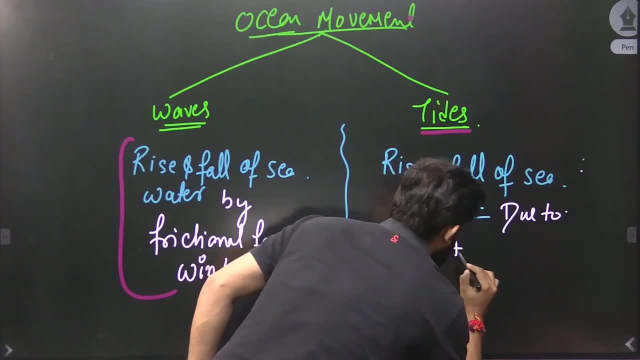 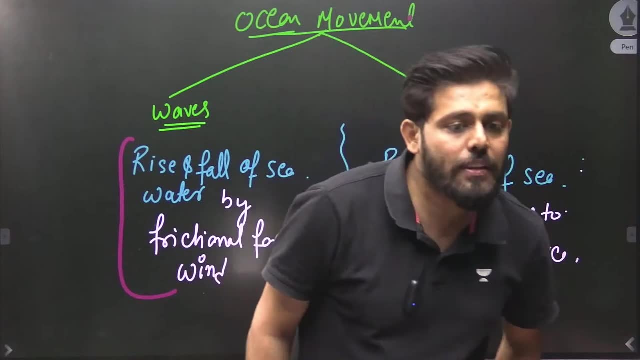 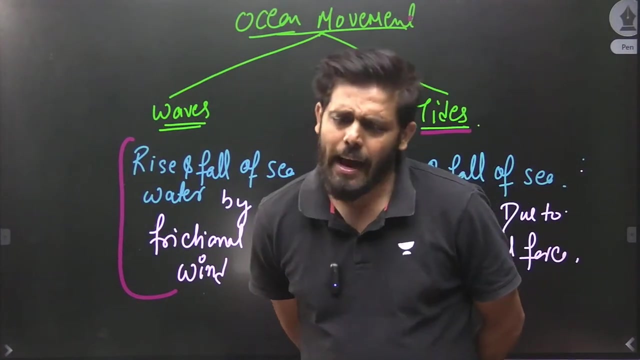 Due to the gravitational force. When there is a rise and fall of sea water due to the gravitational force, it is called tides. It is called tides. I will try to explain to you how this gravitational force is. Okay, Now I will explain everything to you very well. 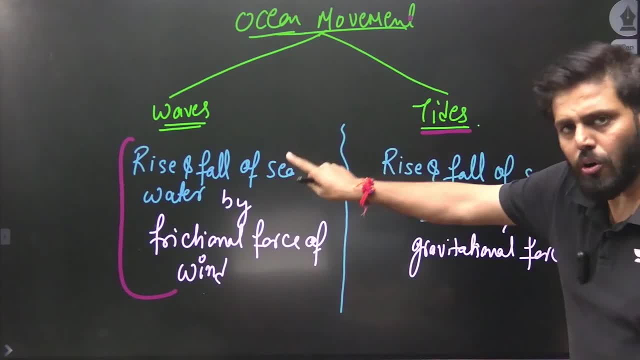 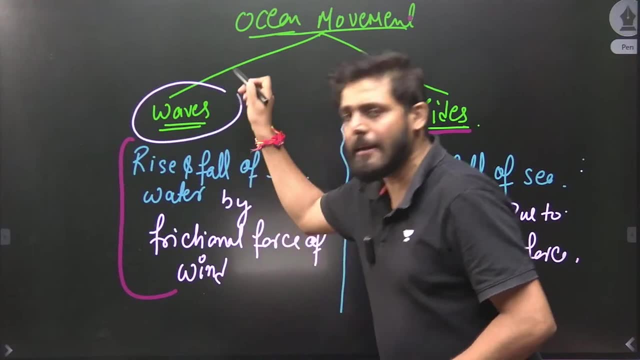 Rise and fall of sea water. both are called waves and tides, But rise and fall of sea water, if it is due to the frictional force of wind, it is called waves, Which we will study in tomorrow's class. How do the ocean waves come? How do they generate? 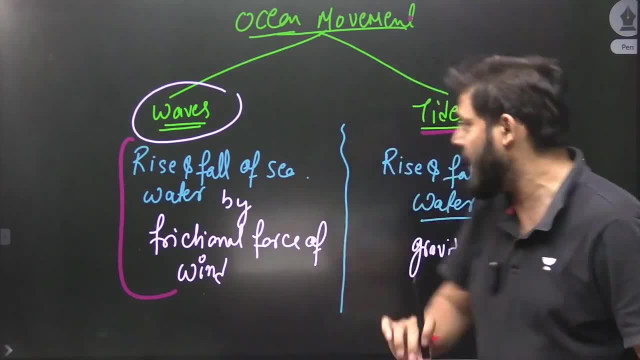 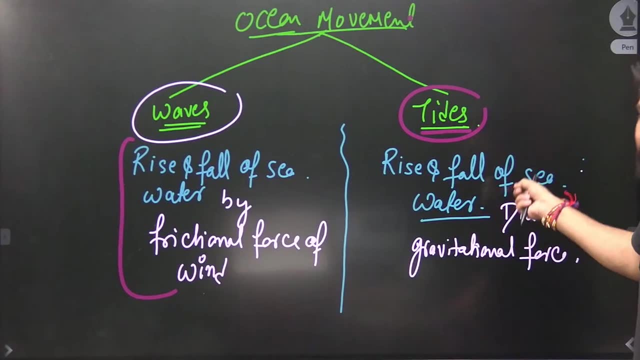 How does the tsunami come? We will talk about those things Today. we will talk about tides, That the rise and fall of sea water due to the gravitational pull, due to the gravitational force. how is it happening? Now, let's move ahead. How many types of tides do we have? First of all, we have two types of tides. That is high tide. The second type is low tide. After that comes one more thing, which is called tidal range. Try to understand tidal range. 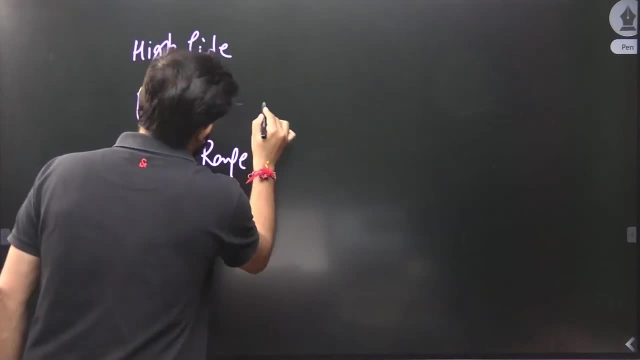 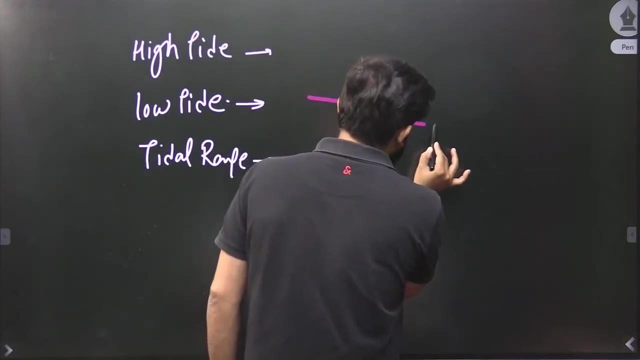 So these are the three things which we have to understand very well. Let's assume we have to understand very well. I have this coastal area here. This whole coastal area is this point Here. you will understand that this whole coastal area is up to here. 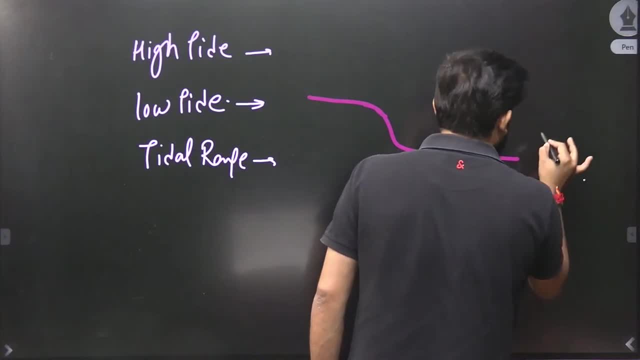 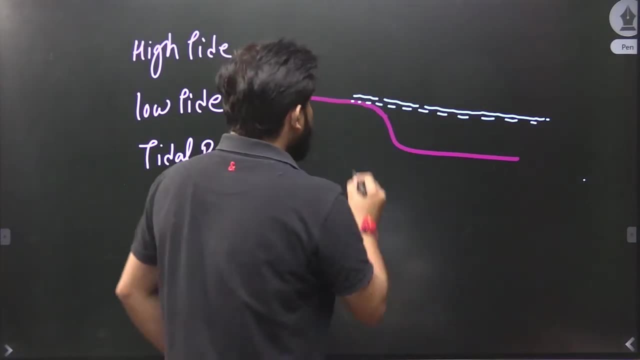 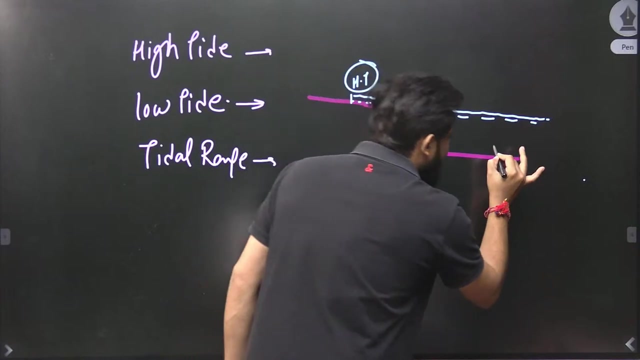 If my water level is up to here- Up to here, At this point, At the very top- Then this will be my high tide. What will happen? HT means high tide, And when my water level comes to this level, When my water level comes to this level, 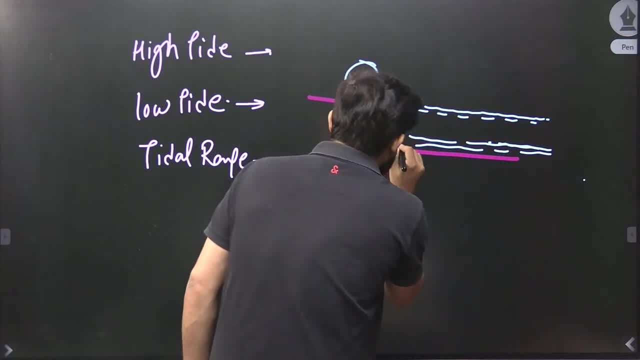 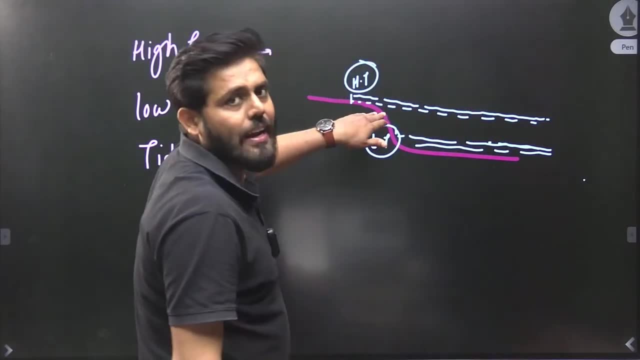 This will be my low tide. What condition will I have here? Low tide. Now I will also explain how this water level is going up and down. If this is a coastal area, You must have seen that once the water comes up to the very top of the coastal area. 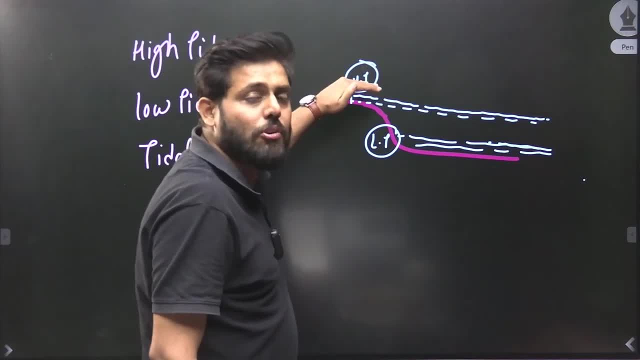 And once it comes down. So when the water comes up- That is known as the high tide At the coastal area- And when the water level stays at the back, You must have seen that the water is at the back of the coast. 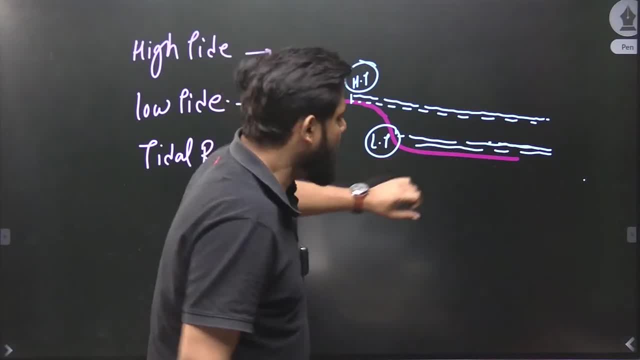 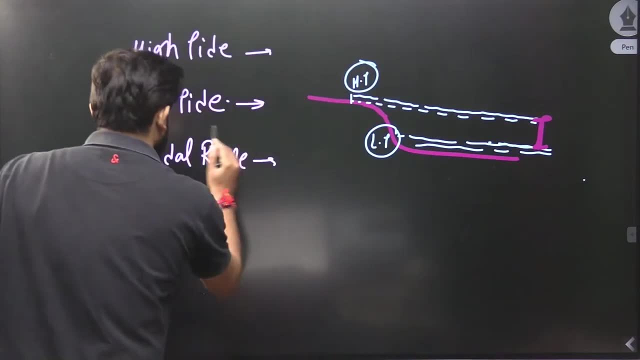 It is at the bottom, So it is called low tide. And the distance between high tide and low tide, The difference, The range. This is called tidal range, The difference between the high tide and the low tide, The difference between this. 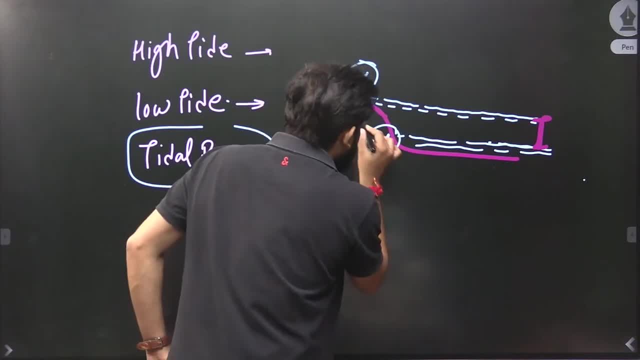 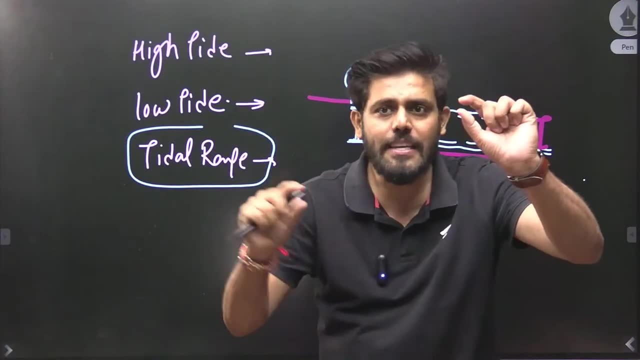 Means how high is it here And how low it is The difference between this. This is called tidal range. That means the range. What is the difference between this? In high and low? That is known as the tidal range. You will have to understand these things. 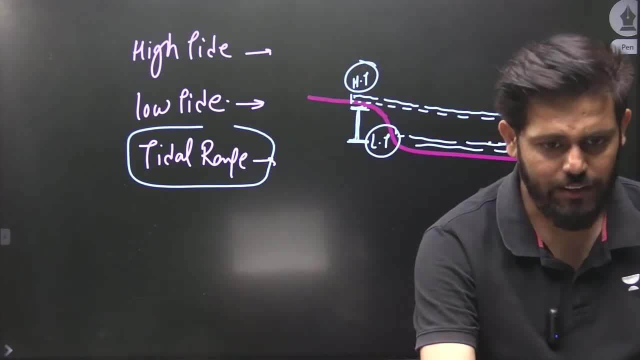 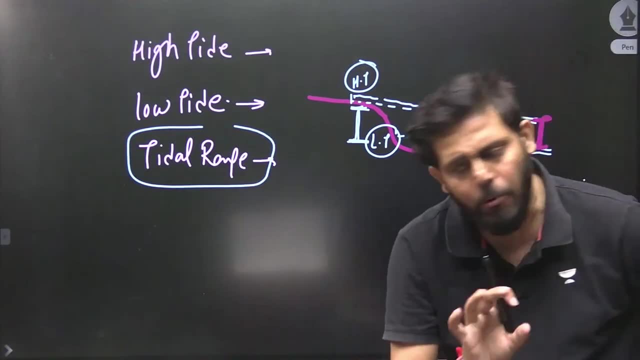 Now, as I will move forward And I will cover you. well, Ok, You will experience all the things. You are going to experience, each and every thing in the class. Very well, Ok, So before that, I will put Identify the bands. 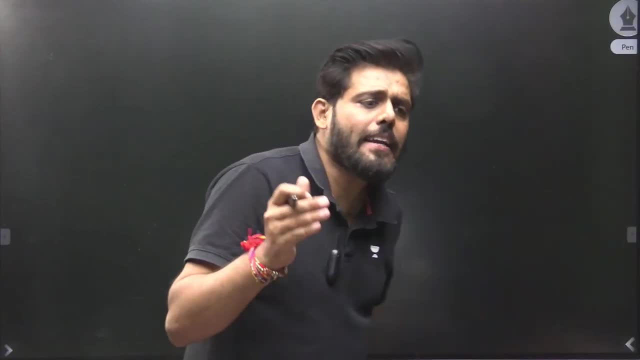 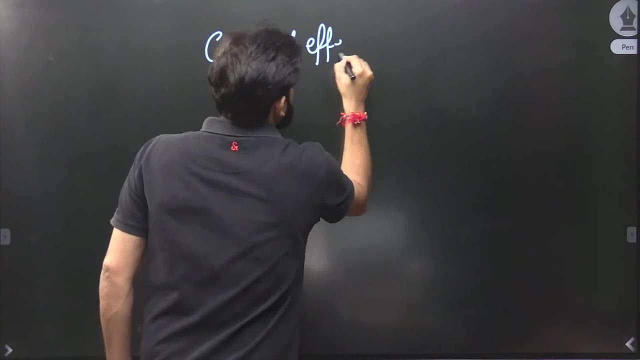 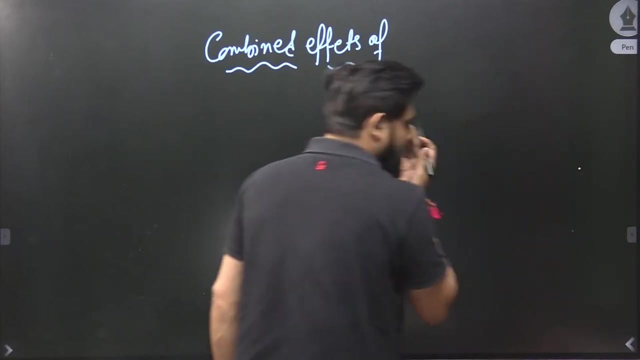 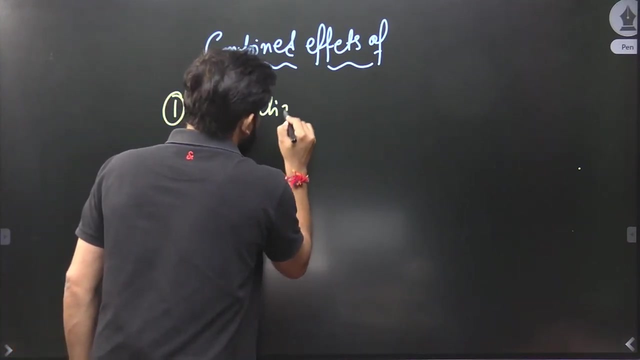 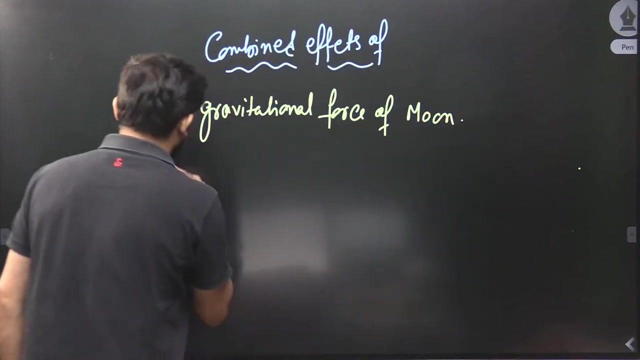 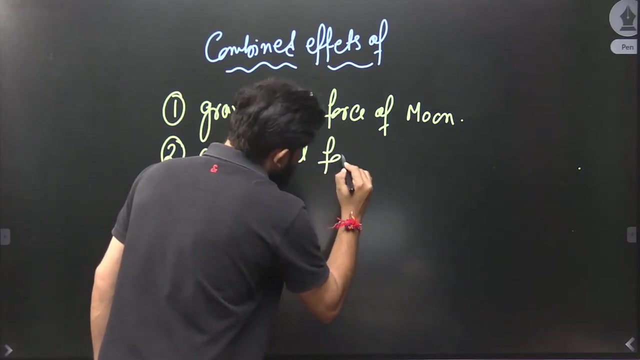 You will also find the pieces 類. It is almost about the same. It is the importance force of moon. moon ki gravitational force ke karan doosra hota hai. gravitational force of sun. sun ki jo gravitational force hoti hai uske. 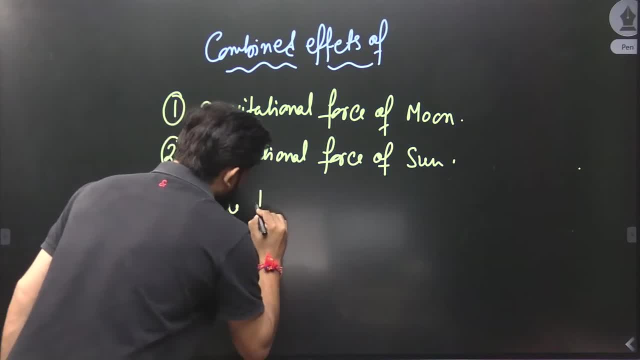 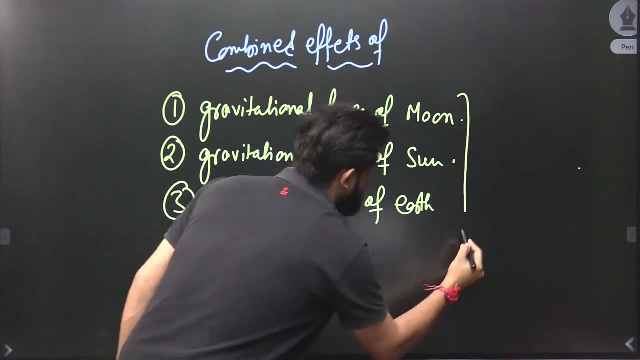 karan aur teesra hota hai due to the rotation of earth, jo earth, apne axis, par rotation of earth aur karan pe Tod hai tyak taro hai boh kaya hoon course, karan ke, uske karan bhi humarir tides ke upar impact hota hai. ye teen factor hai, agar aapne teen ho factors. 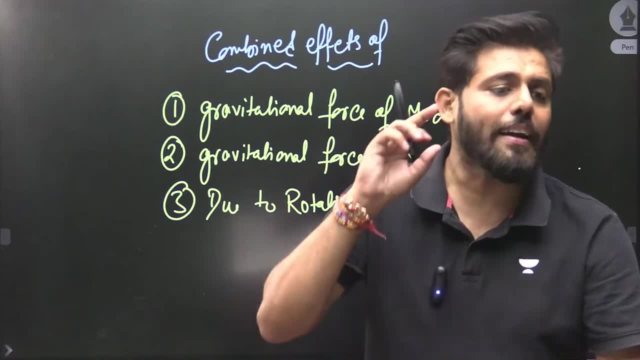 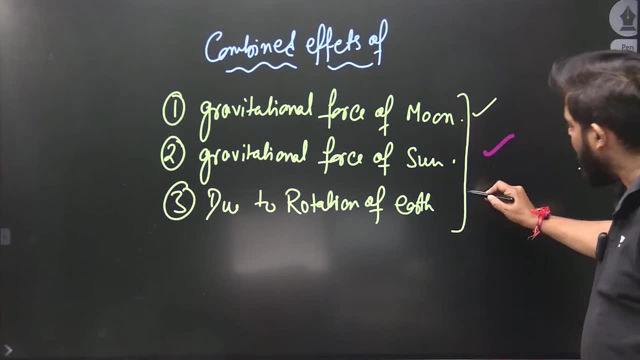 samaj liye, toh aapko cheeje samajhne aad jayenge ki toh ye teen ho factor ek saath role play karte hai, yad raha: gravitational force of moon, gravitational force of sun and gravitational force of ya sorry- due to the rotation of earth, aur may apko bata thoon. 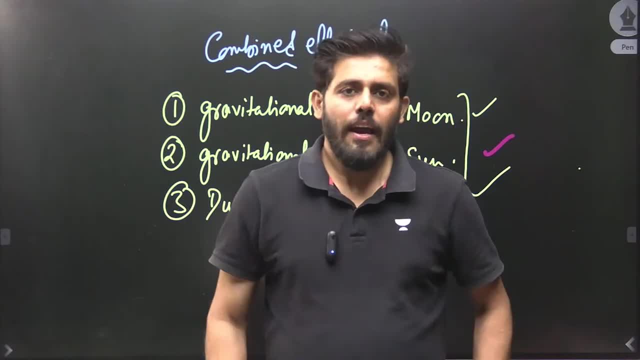 dikhe, guys, bahut aram se suna, bahut hi acche se humari jo bhi bodies hoti hai, jahi humara koi planeet hai, is aapko ke bheakhtar. bahut bhi body, jo bhi bodies k 의� chcia hai kya. 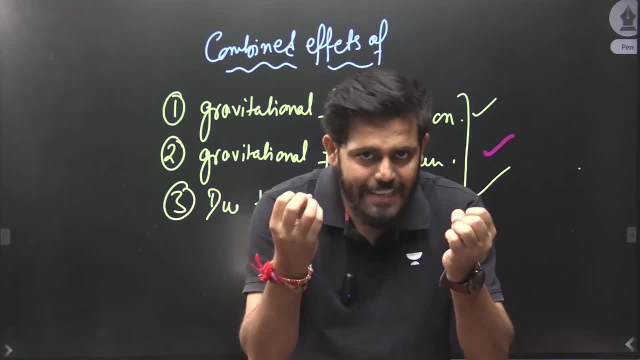 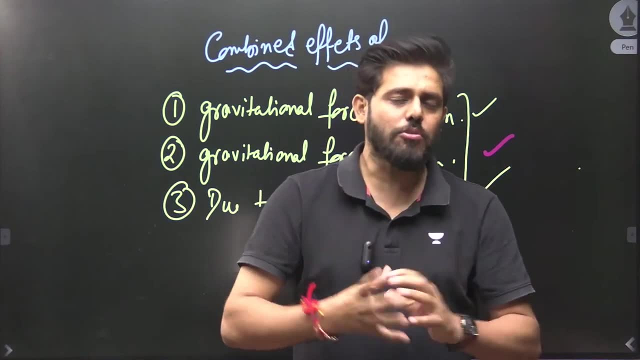 homi body hai inn aparte hai aur the other body may be very, very bad because of the work planet or a star or a satellite. these big bodies which have a lot of mass, they have their own force and that force is called gravitational force. 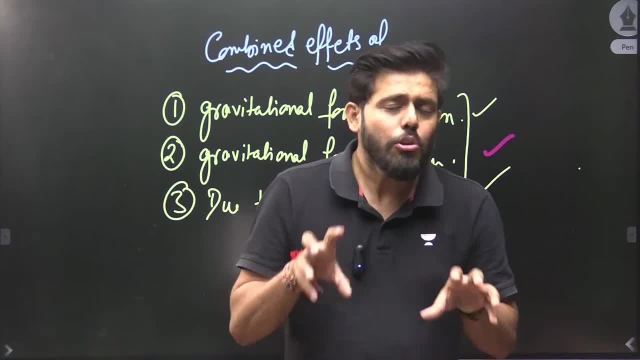 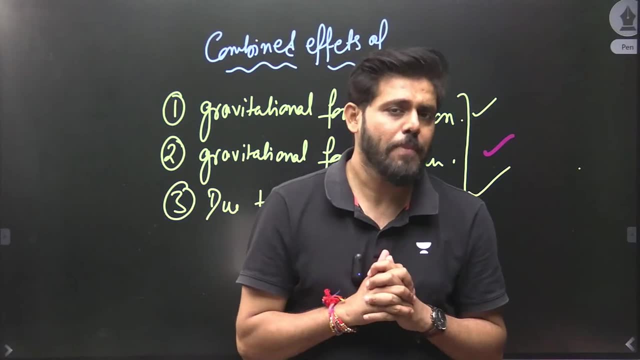 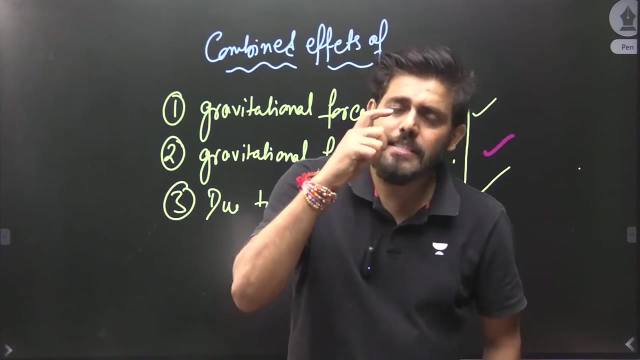 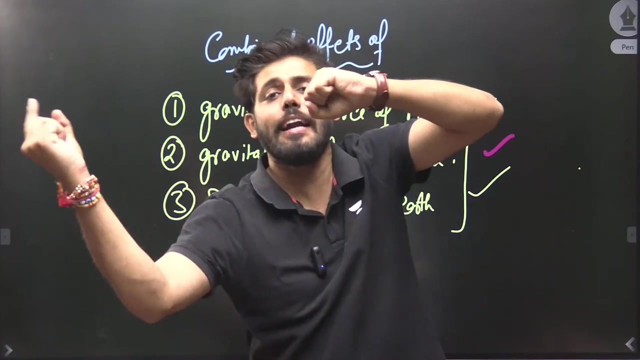 If you are standing on earth today, then it has its own force, that is, the gravitational force which is pulling us towards itself. Just like today earth is holding us because of its gravitational force. just like if there is earth in the centre, then around the earth its satellite moon is revolving. 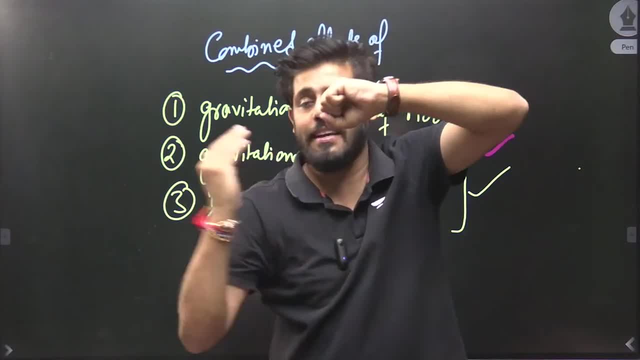 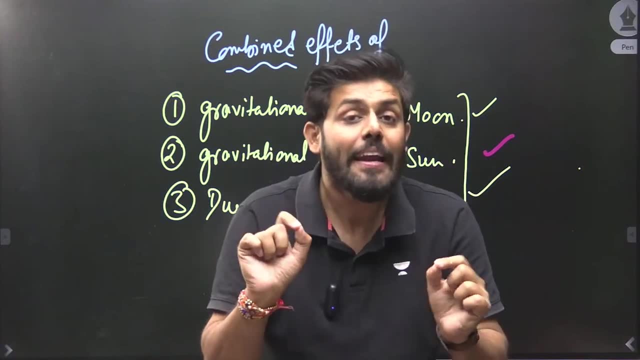 Moon is revolving the earth in all directions. This is how the moon is revolving And the moon is revolving in a particular elliptical path. it is due to the gravitational force of earth. Earth has gravitational force. It is due to the gravitational force of earth. 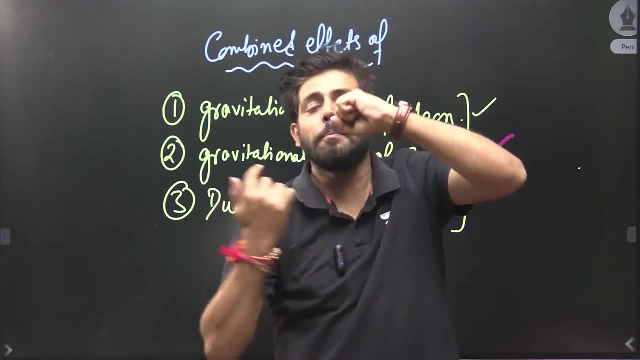 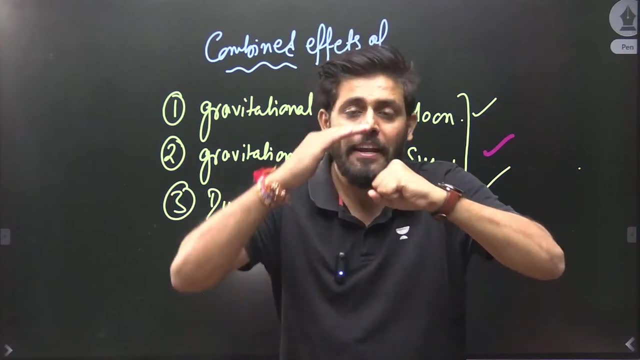 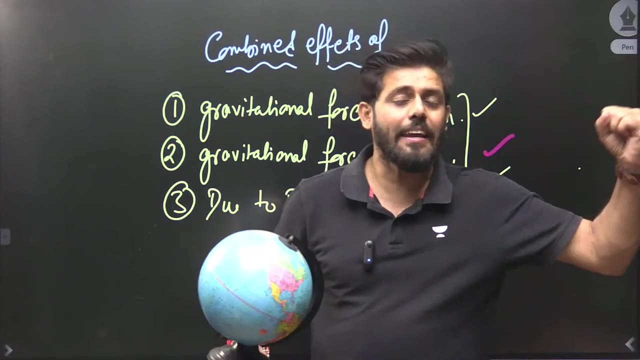 Sun revolves all around the earth in an elliptical path, which is forcing it to revolve in an elliptical path, Just like here on earth. the moon revolves around the earth in elliptical path due to the gravitational force of earth. when we talk here, in an elliptical path, the sun revolves. 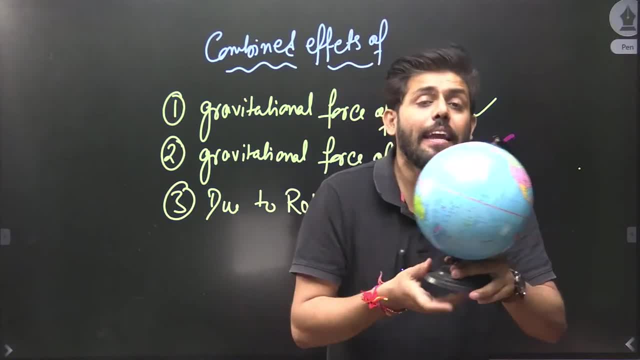 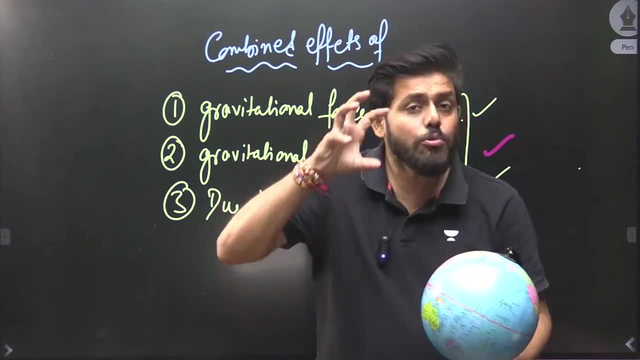 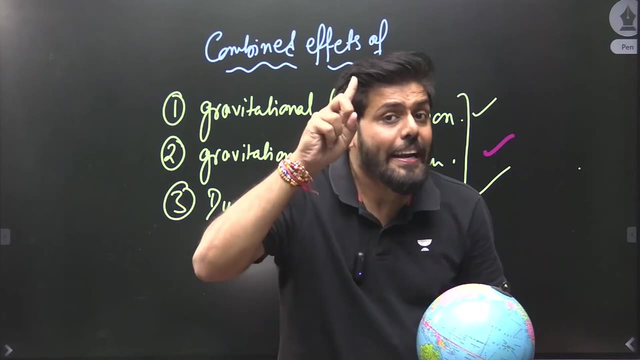 around the sun as well, and this is why the moon is revolving around the sun, And the Sun is very massive and because of this its gravitational force is very strong. But note one point: Gravitational force is inversely proportional to the distance. 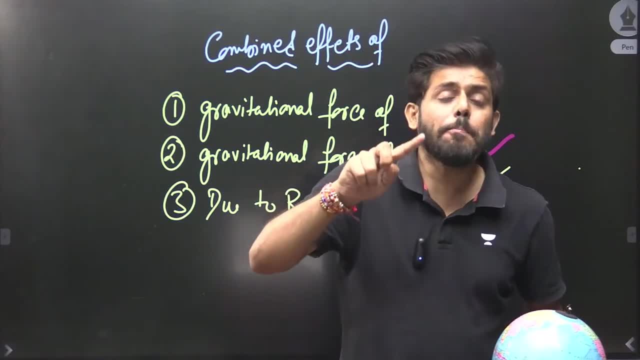 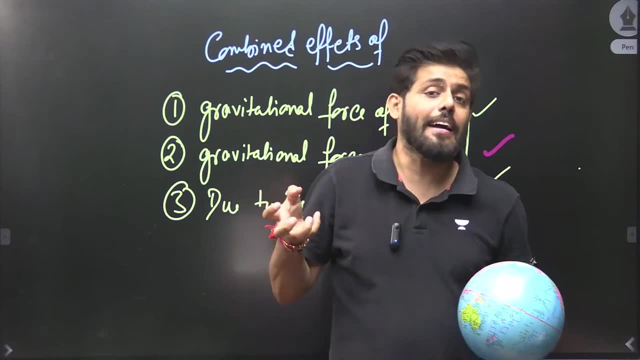 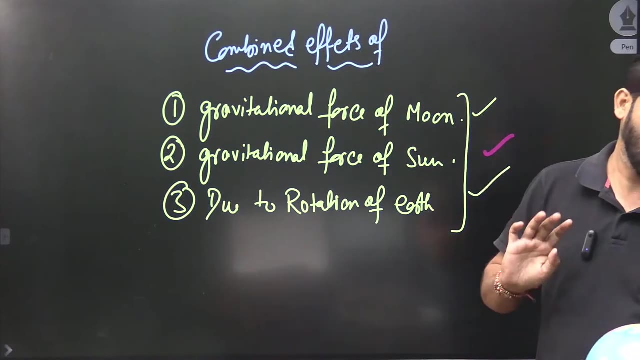 Always remember. gravitational force is inversely proportional to the distance. It means that if the distance is more, then the gravitational force will be less. remember. And because of that gravitational force the tides occur. Now I will explain you very well how all these concepts occur. 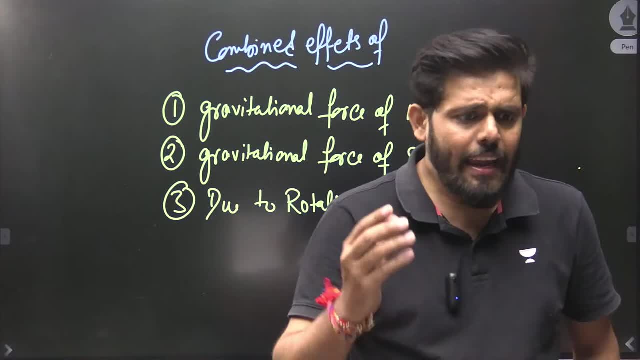 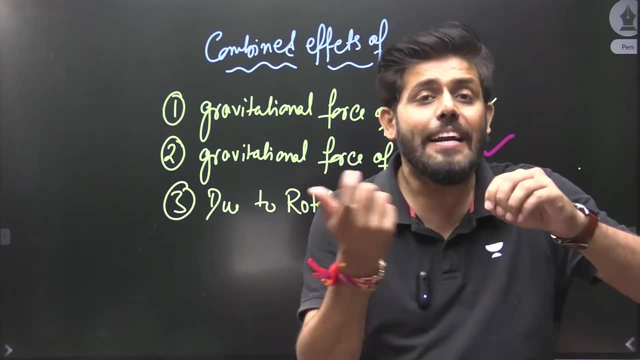 Are you understanding the things till here? Is it clear? Okay, absolutely correct. G1, G2 upon R square. that means inversely proportional to R square. R- what is radius? radius means distance, so it is inversely proportional to it. remember these things. 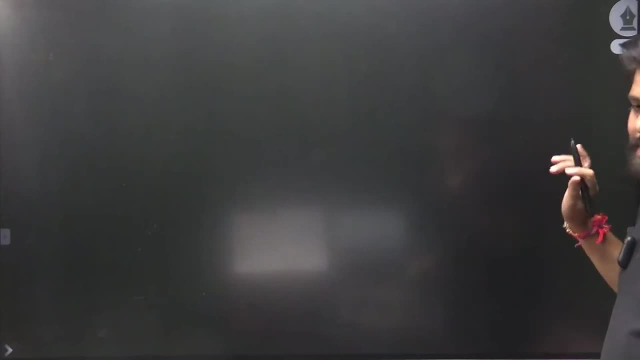 Come now I will explain you more nicely How all these things are happening. Look guys, here this is our earth. Okay, here, what is earth? Now, what is same? Here is our Sun. Here is our Sun. Here is the Sun. 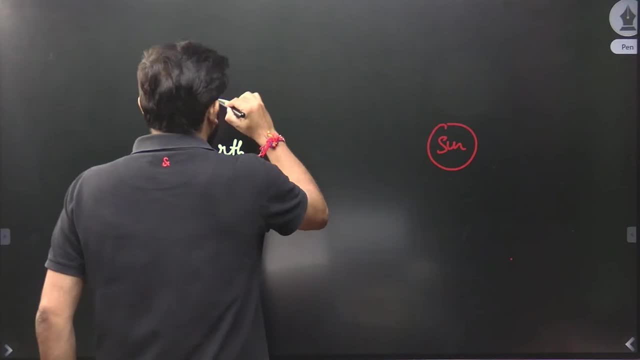 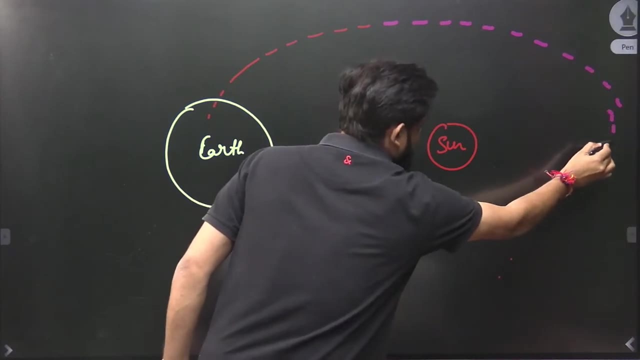 Here is the Sun, So you can say that our earth is revolving around the Sun, in an elliptical path, Around the earth. what is our earth doing? It is revolving in an elliptical path. It is revolving in an elliptical path. 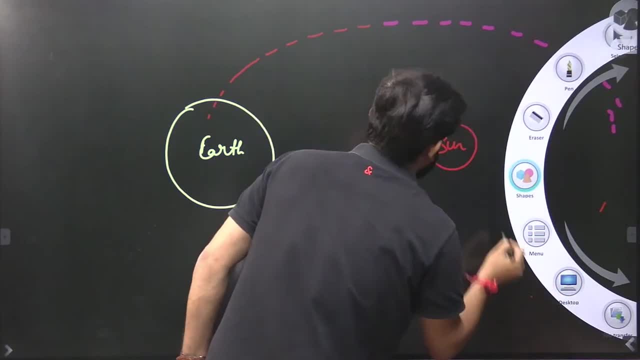 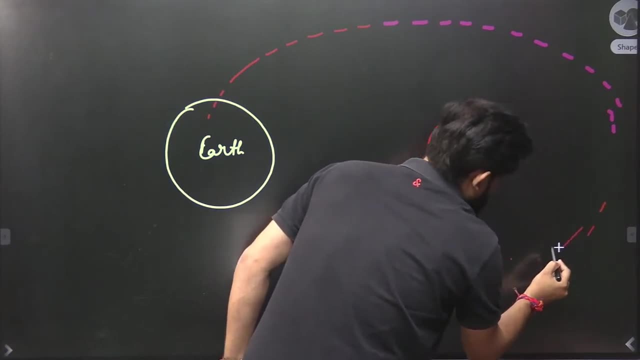 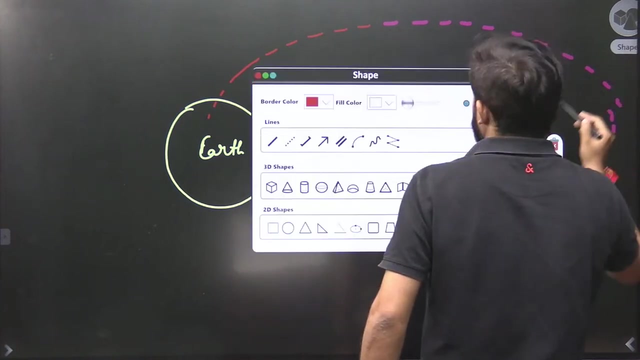 So we can talk like this: just give me, just give me one minute, okay, Here, let's take it from here, from here. oh man, what have I drawn? what have I selected? Let's remove the shape. Where has the shape been selected from me? 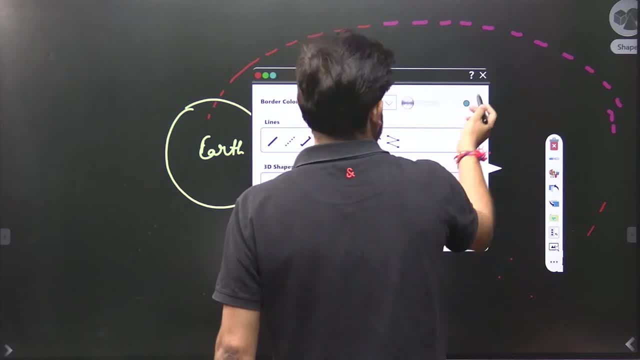 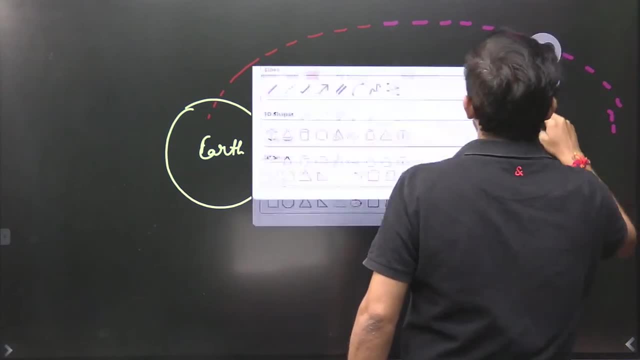 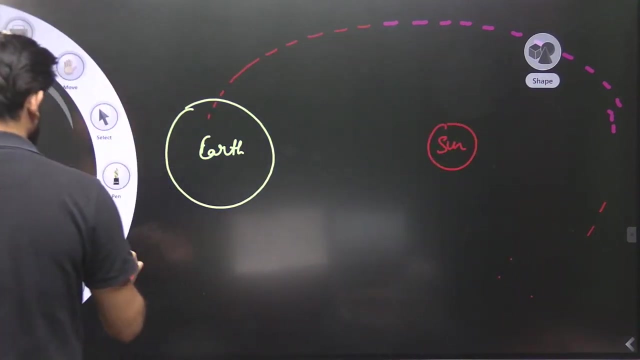 Where has the shape been selected from me, majors? What have I chosen? All of a sudden, we started yawning. Is that how the other set ofenciapline is doing Now? dancing, Dancing. Did we go dancing? Yes, we did. 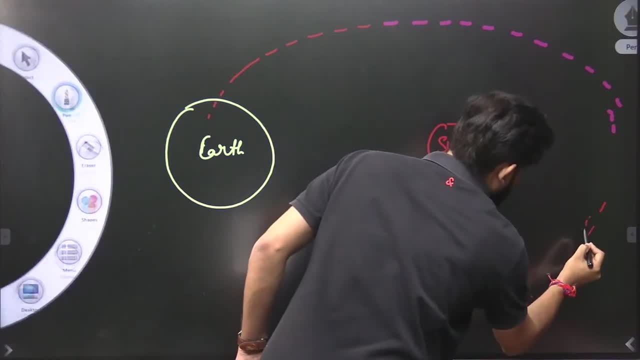 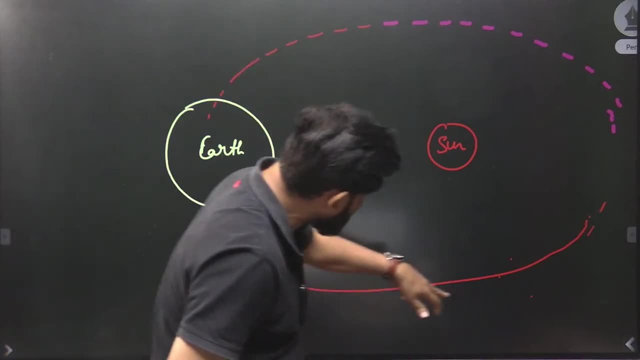 Is anyone here? has put down the dance. Is anyone here? how about dancing? Is everyone here? how is everyone dancing? Now the lights has people dancing. Your are dancing like a child dance. is what Does anyone here? or you live in standing position. 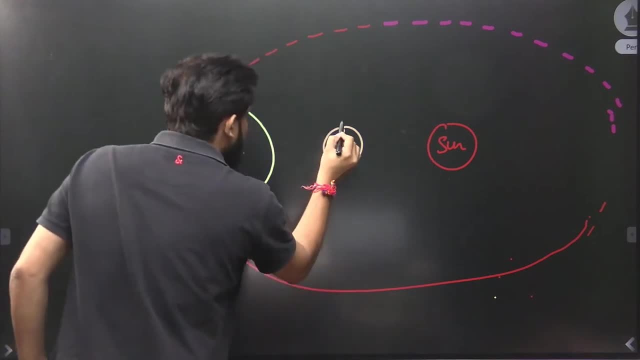 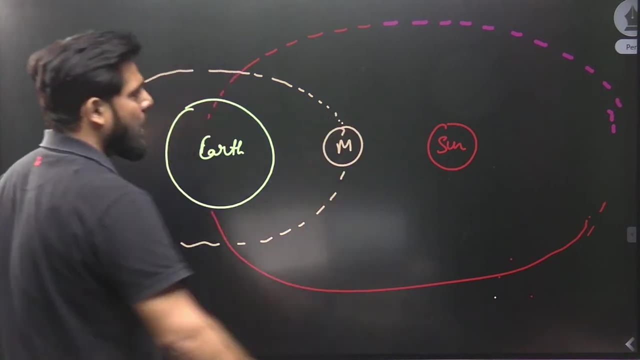 Yes, we are there. Yes, I am there. Yes, we are there. Yes, we are there, We are there. Yes, we are there. Would anyone dance? The moon is also revolving around the earth in an elliptical path. Remember these things. 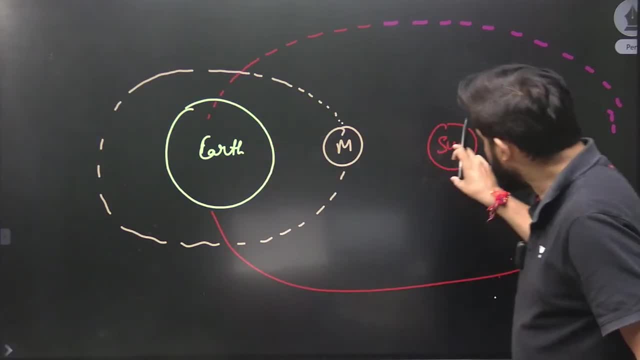 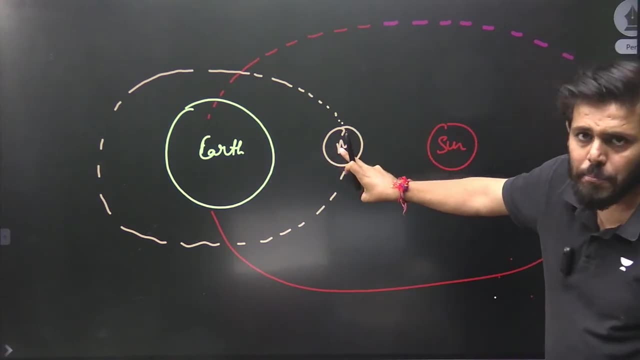 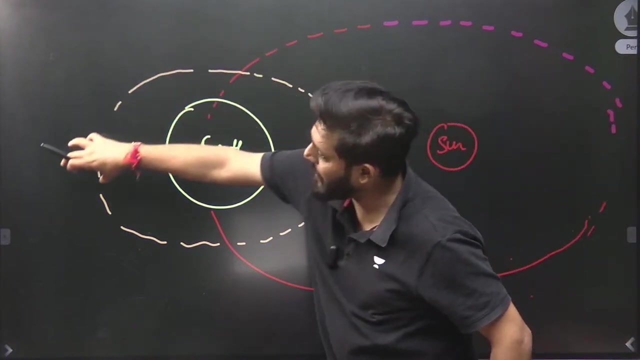 You all must be aware that the earth revolves around the sun. The moon is the only natural satellite of the earth. The moon is revolving around the earth in an elliptical path. Its position will be here, here, here and here, Because when it is revolving, its position will change. 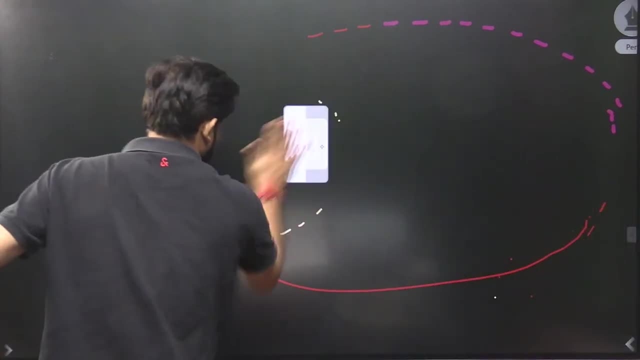 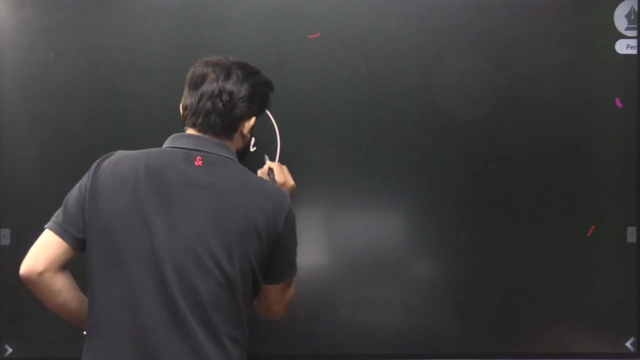 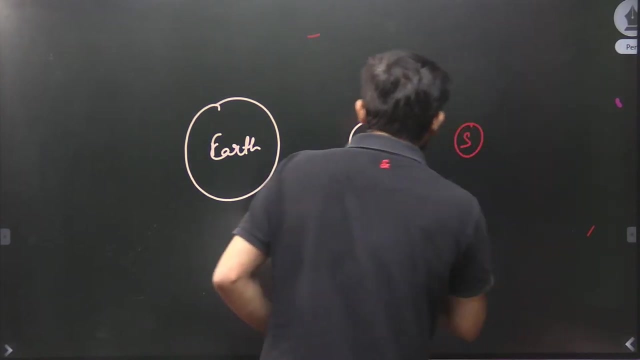 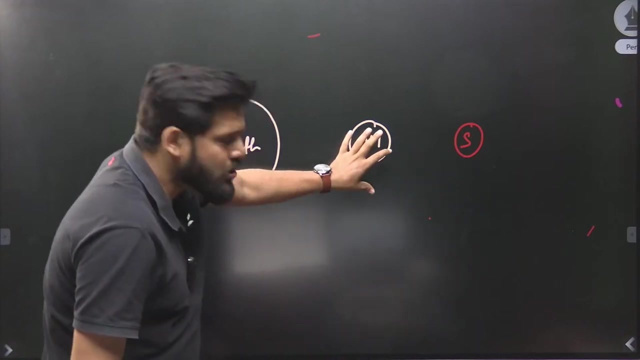 Now, what is the condition? I have already explained this to you. Now, what will be the condition? If this is our earth and this is our moon, then this is our sun. Now what is happening? Earth, moon and sun. Here, the gravitational force is of the sun and the gravitational force is of the moon. 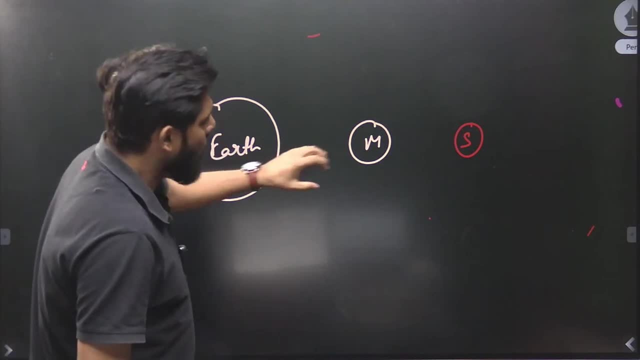 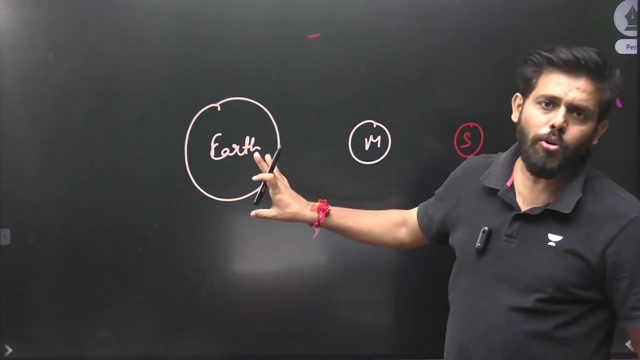 The gravitational force of the moon is revolving around the earth And the gravitational force of the sun is also revolving around the earth. But the point is that where is that gravitational force? You all know that our earth has water present in the two-thirds area of our earth. 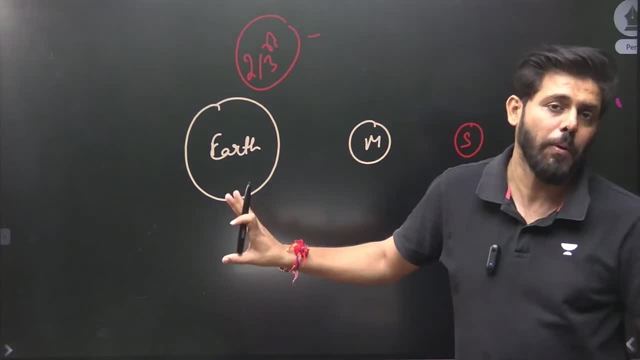 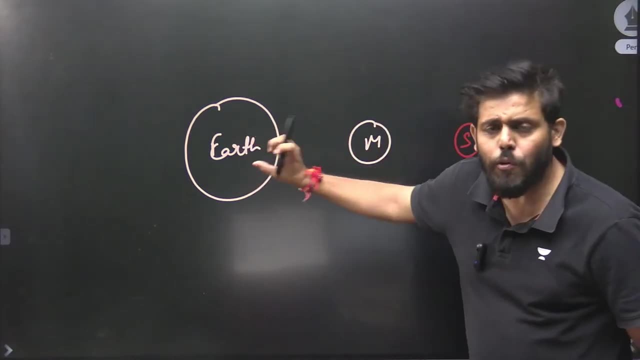 That means there is a huge amount of water present on the earth. Now, what will happen When the gravitational pull of the moon will be on the earth? then what will it do? It will pull the water. What will it do? It will pull the water towards itself. 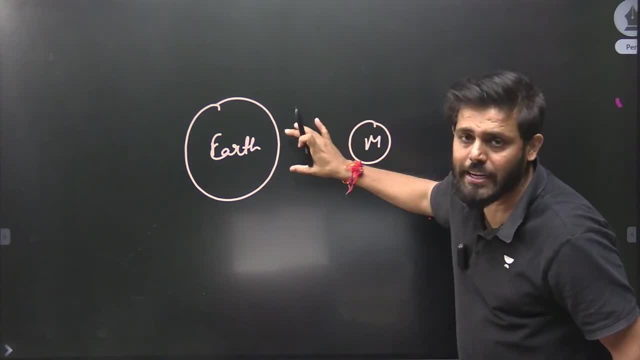 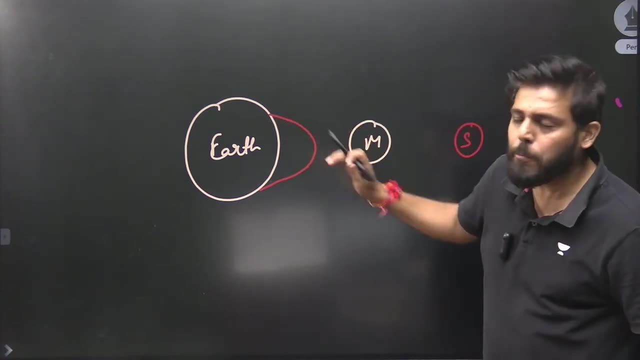 So when it will pull the water, then the direction in which the moon is applying the gravitational force, the water will pull from here in this way, This area here, And when the water will pull from here, then the high tide will come in this area. 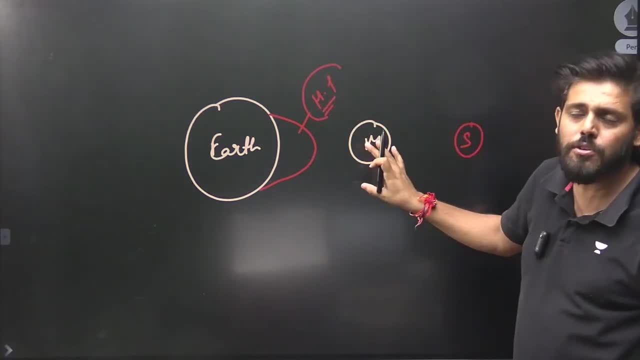 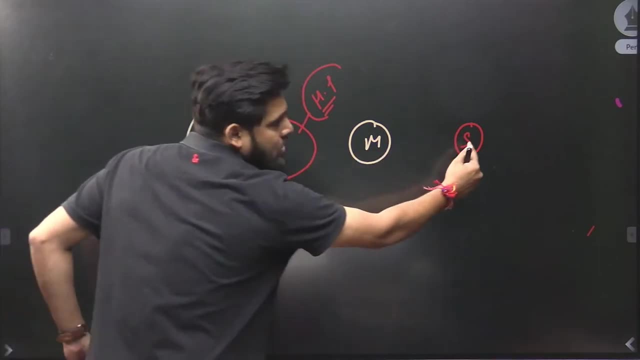 Now you will say, sir, will it be only the gravitational force of the moon or the gravitational force of the sun? Because when the moon and the sun will be in the same line, that means earth, moon and sun, these three are in the same straight line. then the gravitational force of the moon and the sun will be added to both. So that means the gravitational force of the sun and the gravitational force of the moon will be the same. Both these gravitational forces will be stronger and will be applied to the earth at the same time. 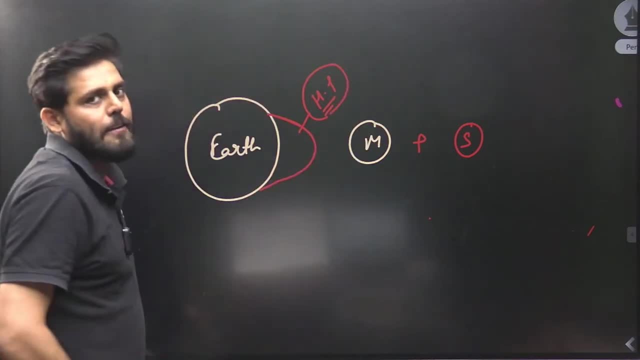 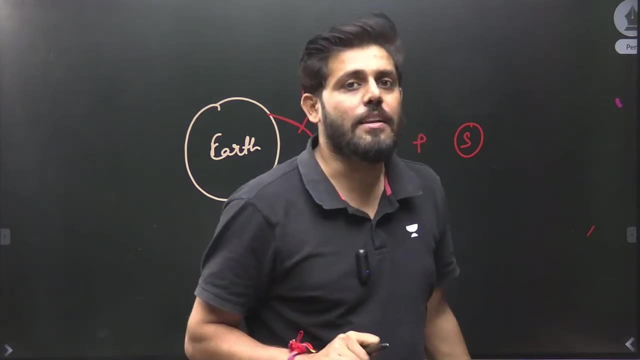 Because of which your high tide will come in this portion of the earth. And if I ask you whose gravitational force will be more, which will be applied to the earth, Your answer will be the sun. But that is absolutely wrong. The gravitational force of the sun is very strong. 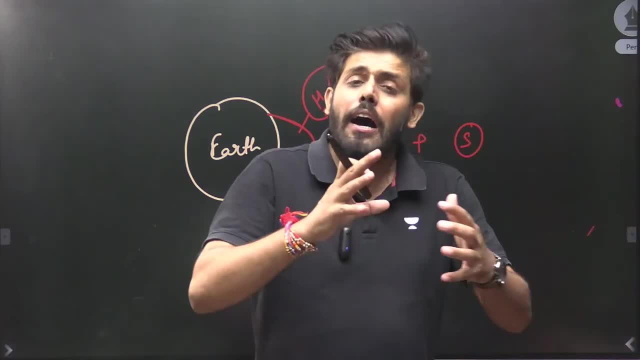 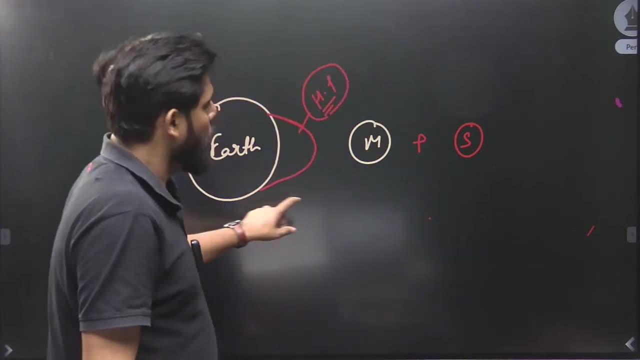 It is very strong. It is very strong. It is 1000 times stronger than our moon, If I talk about the gravitational force of the sun. But the point is that the distance from the earth, the moon is close and the sun is very far. 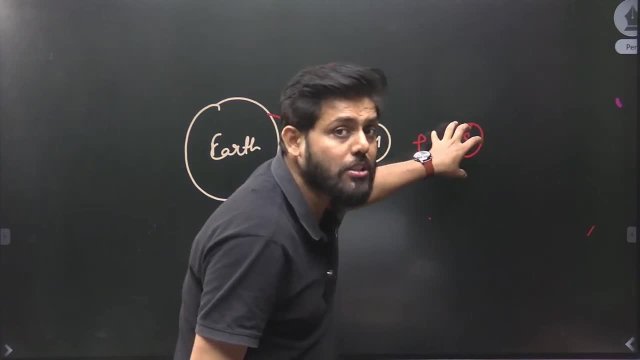 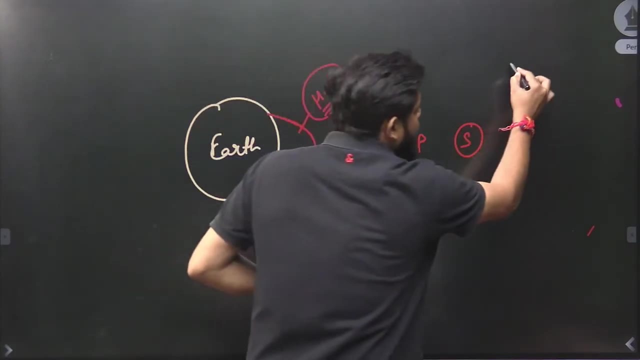 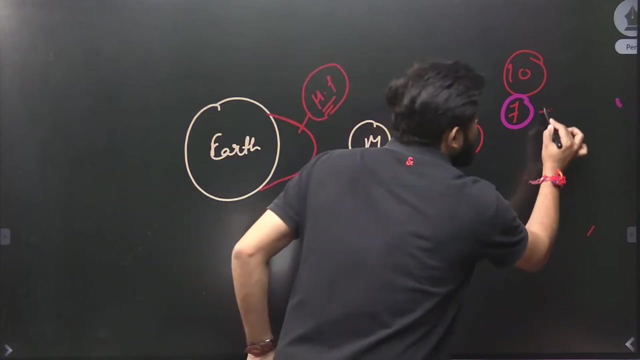 So its gravitational force is very strong, But the force that will act is not that strong. The force of both will be added, But the point is that if 10 units of force is applied to the earth, then 7 units of force will be of the moon and the remaining 3 units will be of the sun. 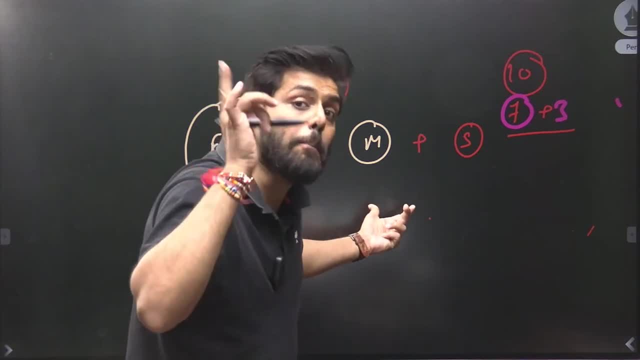 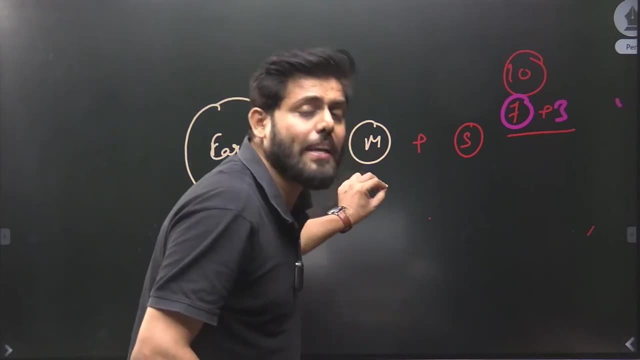 That means the gravitational pull will be stronger. Always remember about the moon whenever there is a tide. In the case of the tide, the tide that comes on the earth is stronger because of the gravitational force of the moon, Because the moon is close to our earth. 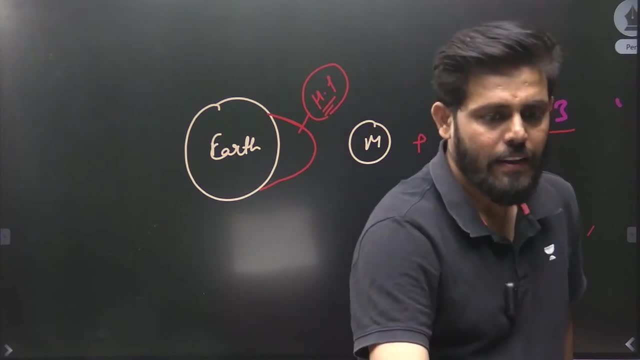 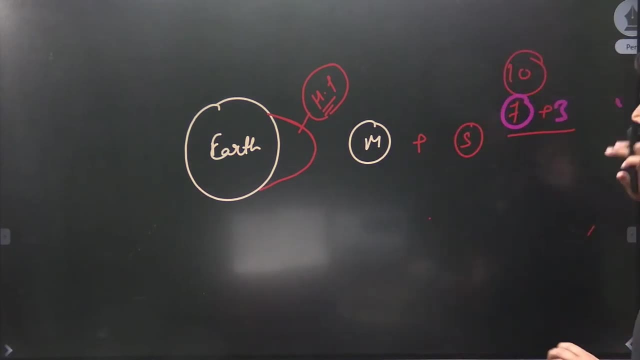 Okay, Who understood this point? Who understood this point here? Is it clear? Did you understand this point? Once all the students like and share if the things are clear, Okay, You understood this point. So now what happened? The sun and the moon are in a straight line. 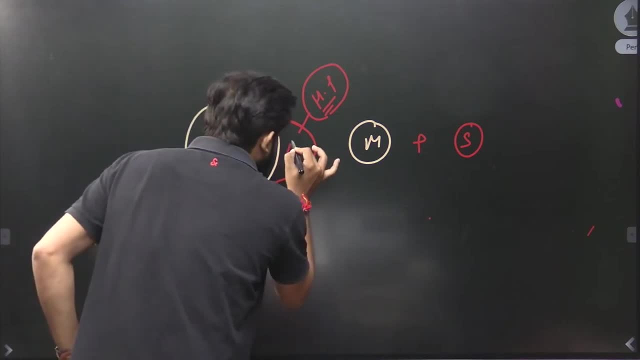 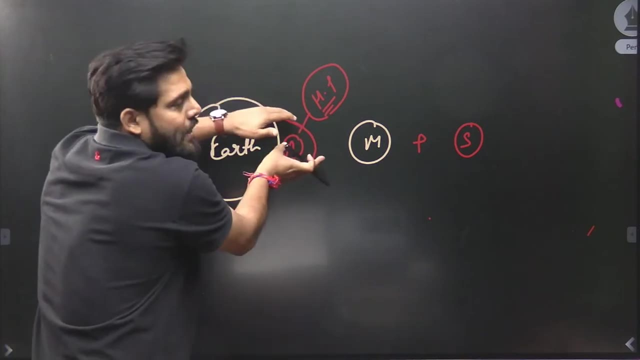 Because of which our high tide came here. So the point A: our high tide will come here on the earth. That means the water of this area will also come here And the high tide will come here. Remember these things. Now, the point is that the high tide will come here. 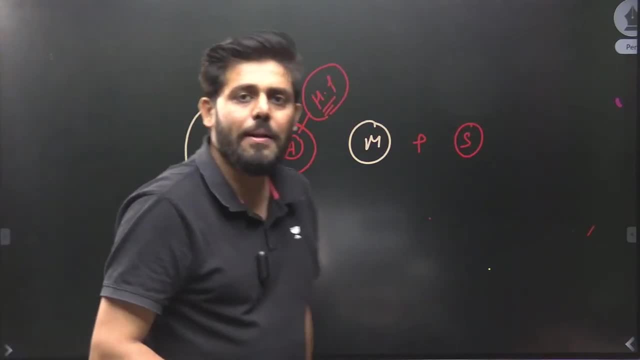 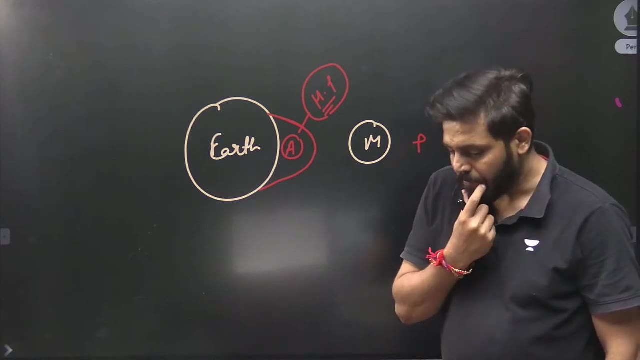 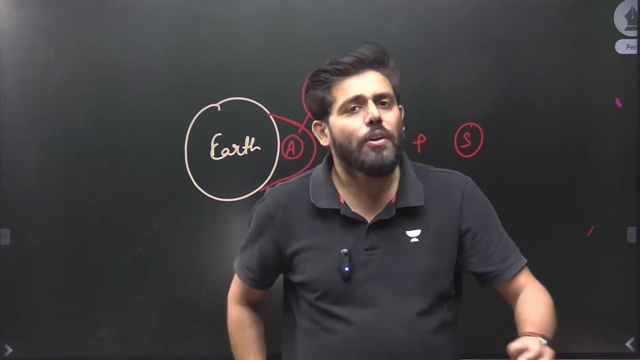 And the back part of it will come here. Here it means that the low tide should come. The back part should be low tide here. No, sir, This does not happen. Always remember Any body, Any body, Every rotating body, If any body is rotating. 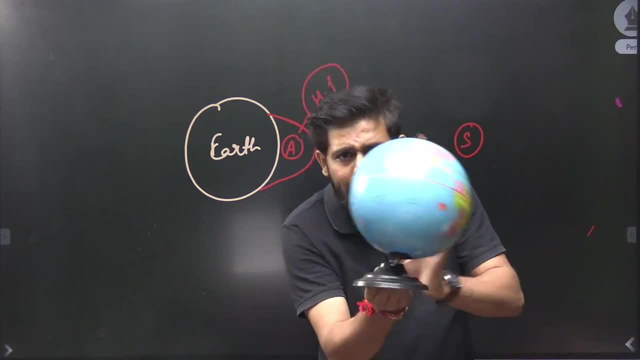 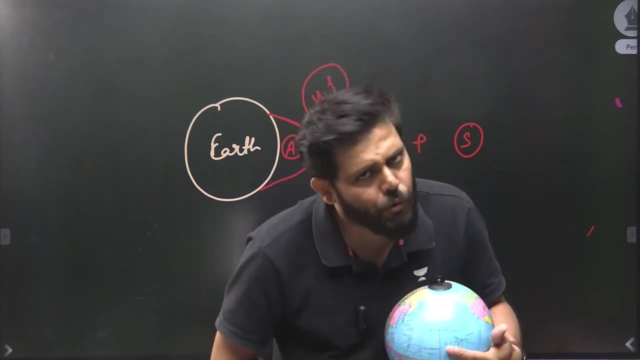 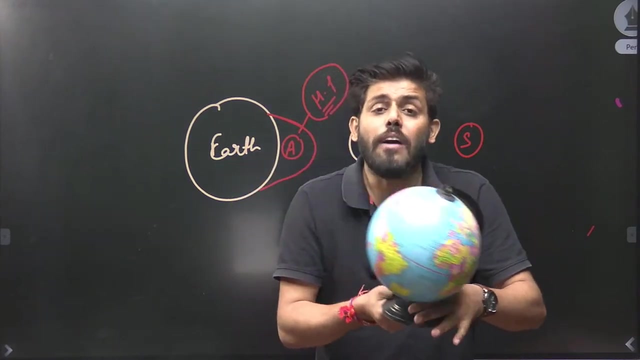 If any body is rotating like this, Then you know that if any large body has its own gravitational force, It has its own gravitational force. But remember To counter that gravitational force It has another force Which is generated. It is called centrifugal force. 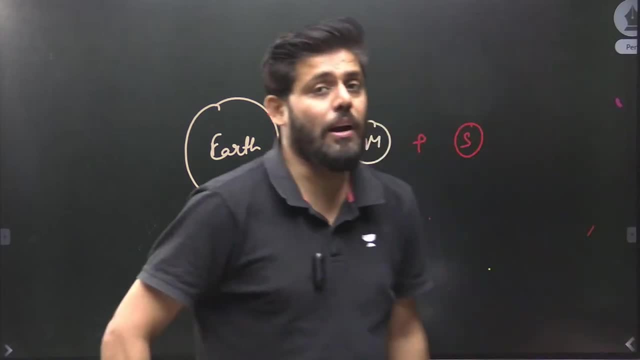 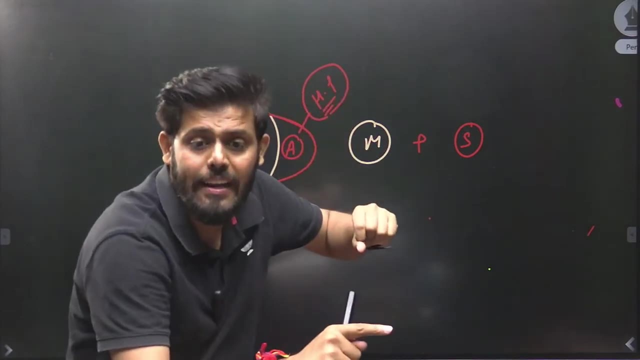 Always remember. You must have studied in physics too, That any rotating body, When it rotates, Then its gravitational force To counter it, To counterbalance it, There is a force. It is called centrifugal force. So when this gravitational force is applied here, 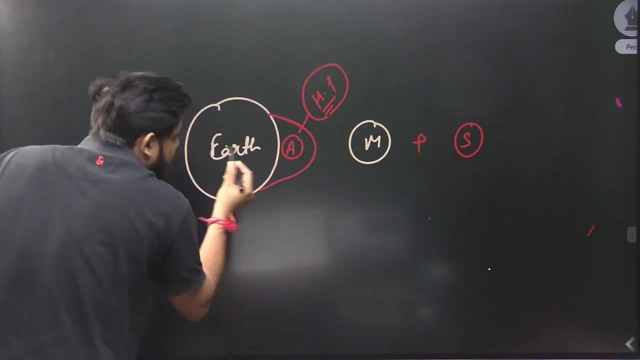 Of the moon and the sun To counterbalance it In the opposite direction. Here There will be another force applied, And that force is called centrifugal force. And this centrifugal force too, An equal and opposite bulge, Will apply in the back too. 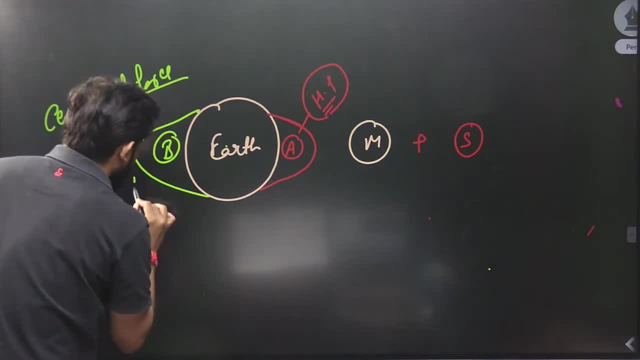 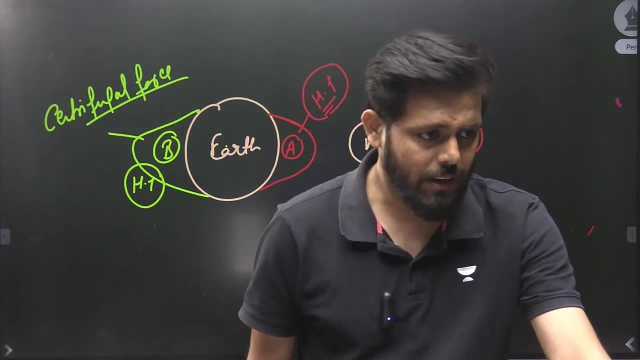 And here too, high tide will come At this B location. What will happen? High tide will come. I will tell you an example. Very good. I will tell a very good example. Try to listen. Have you ever done washing? Have you ever seen a washing machine rotating? 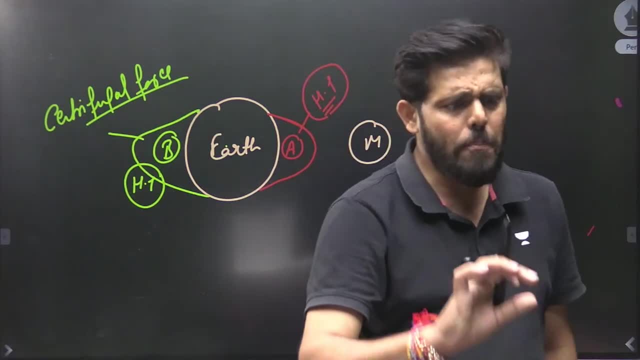 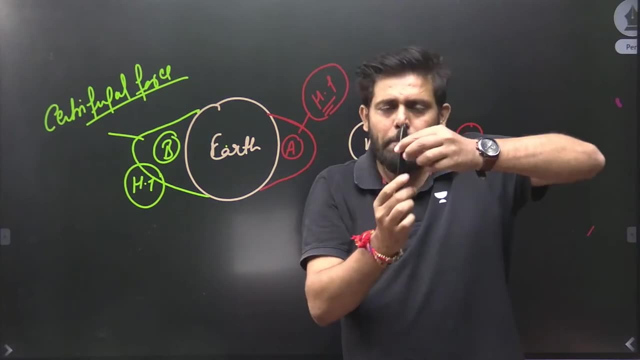 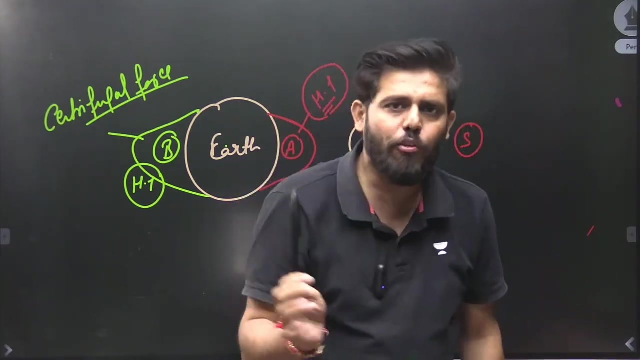 How many students have seen a washing machine rotating? A lot of people have seen a washing machine. So when a washing machine rotates it goes towards its center. When in the middle a washing machine has a stand type in the middle, if it is automatic then it doesn't even exist there. 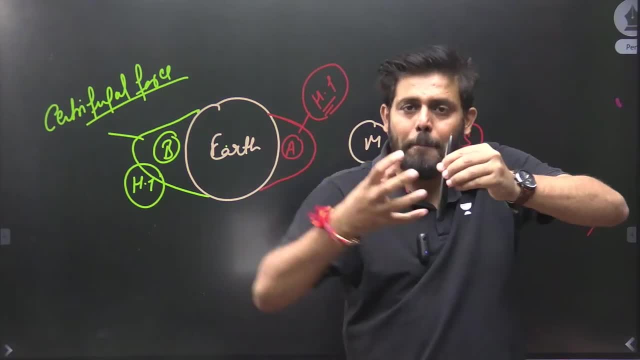 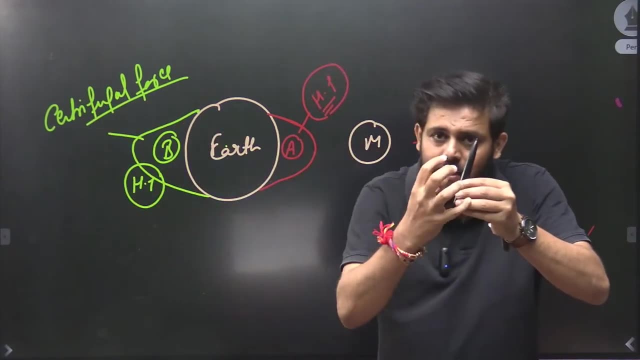 So when it rotates, it drags the clothes towards itself, But sometimes, when you have that gravitational force due to the rotation, but there is a centrifugal force, so the clothes that are going inwards also go outwards, Due to which all the clothes are washed. 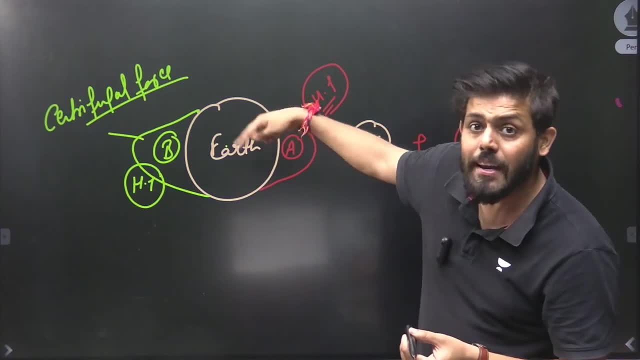 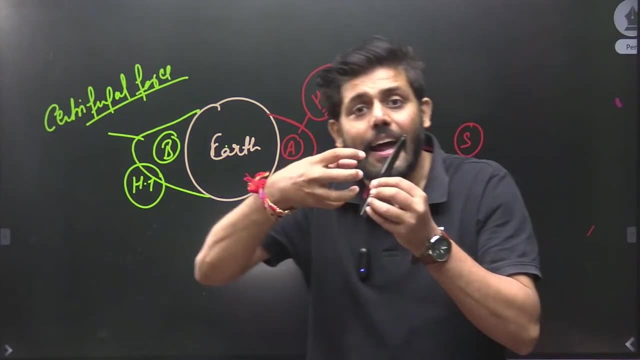 So the same concept that is applied in the washing machine, it is also with our earth. Any rotating body, if there is a gravitational force that is pulling it towards itself, due to which a centrifugal force is applied in an opposite direction, equal. 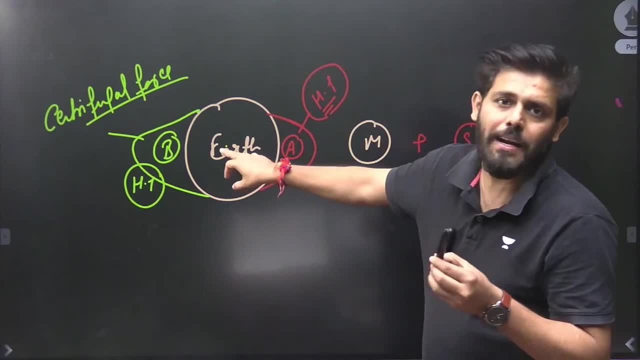 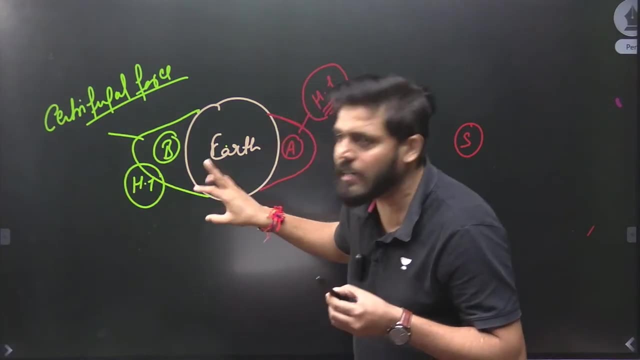 which will counterbalance it. it is exactly equal. it is applied on the earth And on that counterbalance force, our centrifugal force, is applied on the back and it will also bring a high tide towards the back. It will also bring a high tide towards the back. 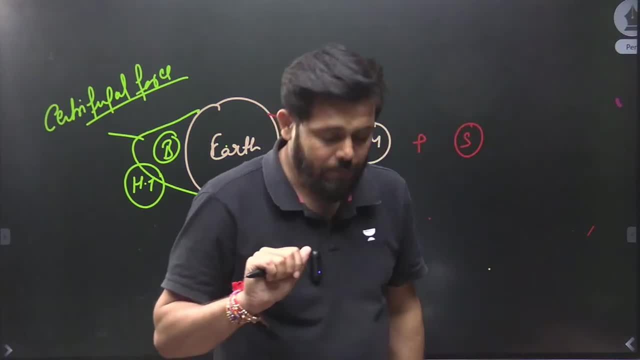 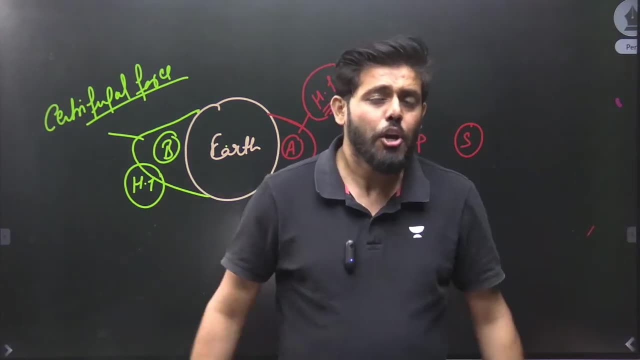 Is it clear? Now I will tell you one more good concept. very good, You must have seen that a rotating wheel comes. I think my name is getting skipped. What happens is that when we were very small children, so everyone would stand on it and move. 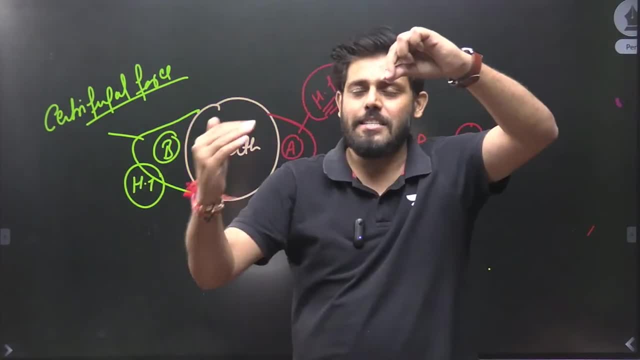 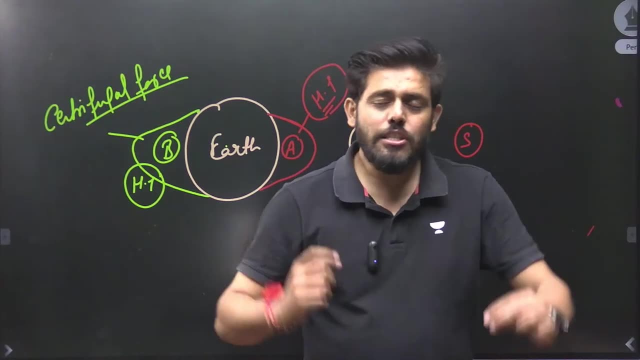 they would rotate in this way in the round There were different stands in it. four or five people would stand and then rotate it, So it would rotate. So have you ever noticed that when we stand on it, when we used to rotate it fast. 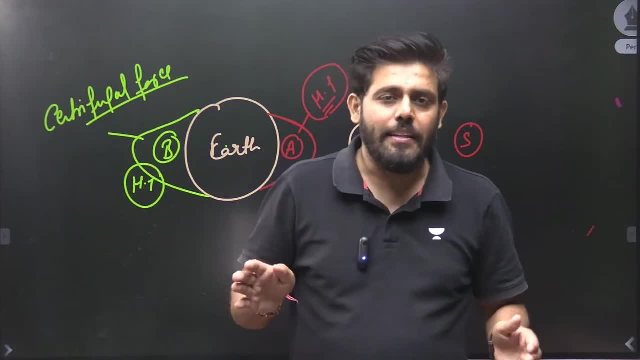 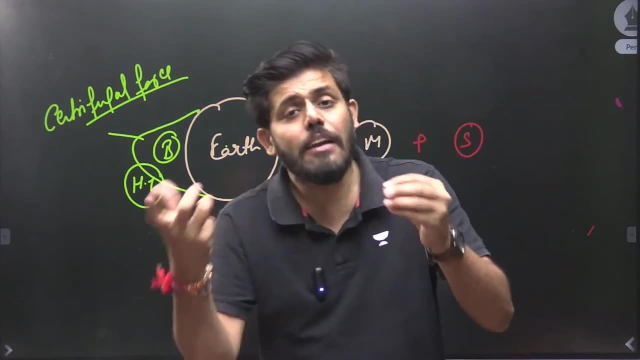 then if any child is standing on it, then it would not fall When we used to rotate it fast. if we hold it properly, because the gravitational force is looking like a force equal to balance it, that is, centrifugal force, due to which any outside 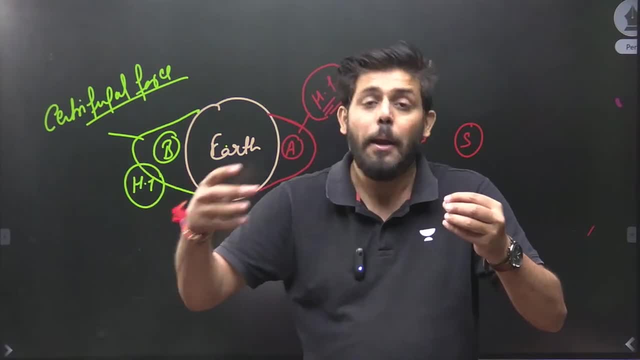 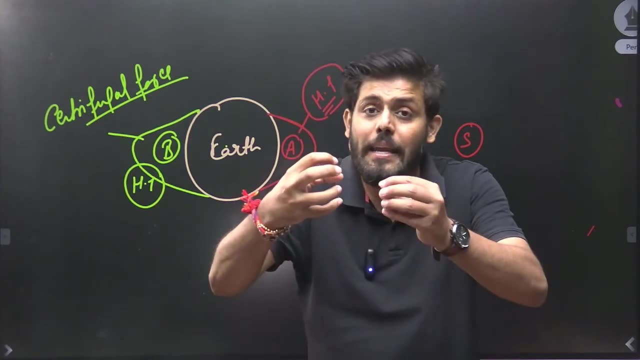 if someone is looking inside, then so much force is applied to the outside. But remember when we stopped rotating it its speed was a little slow. then you see that on the outside see things you fall. then you will start rotating it. 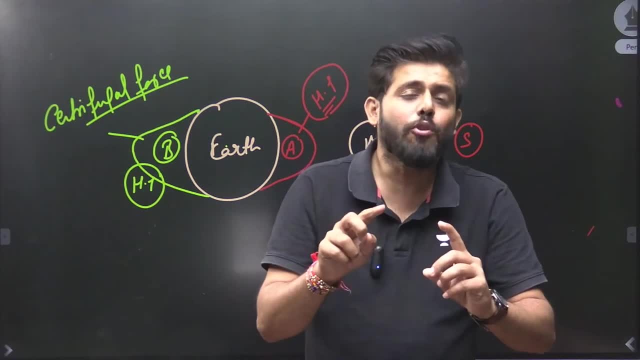 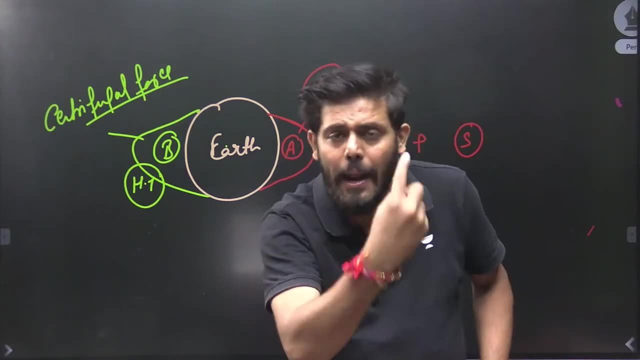 Or you will come inside. Do you know the reason? Because the counter-balance forces are not equal there. That means the gravitational and centrifugal force are not equal. If you are rotating it at a high speed, then you will start to spin in this way. 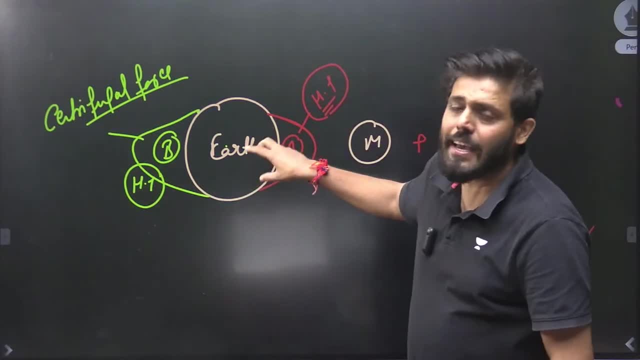 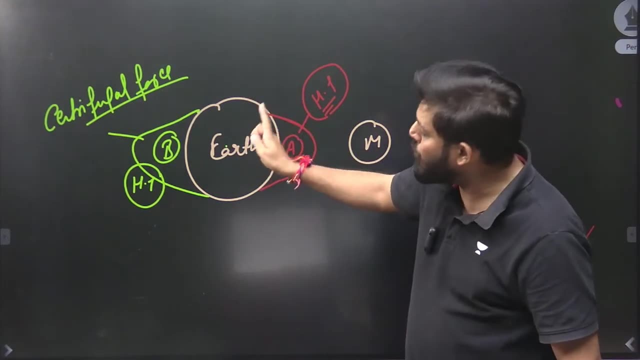 but you will not fall from it. So the same condition applies here, that when, due to rotation, there is gravitational force here, then, due to the gravitational force of a rotating body, an equal counter-balance force is applied. It is called centrifugal force. 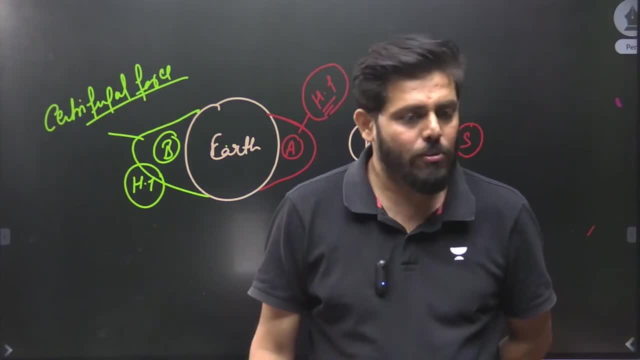 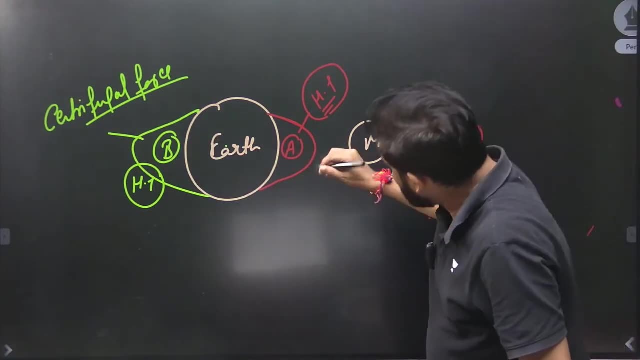 Remember this thing: Merry-go-round is absolutely correct, Ferris wheel is absolutely correct, So those things happen here. The same concept applies here Now. here, at A point, the high tide will come. Due to whom? Due to the gravitational force of the moon and the sun. 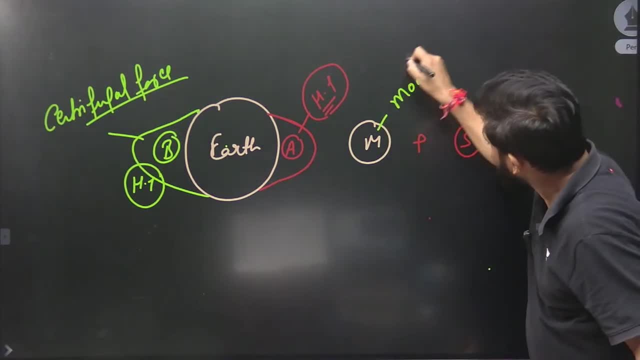 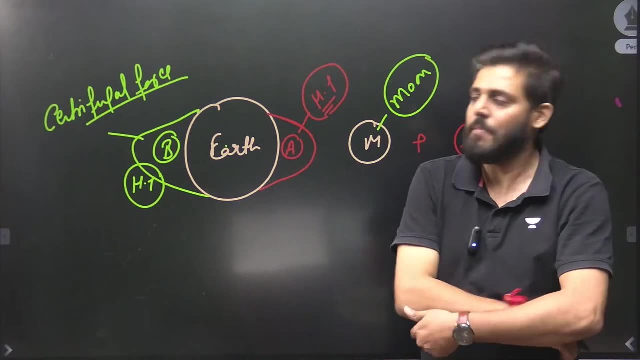 Who is strong? The gravitational force of the strong moon, Now the gravitational force of the moon, And here at the back, the high tide that has come. it has come due to centrifugal force. Here is the high tide. here is the high tide. 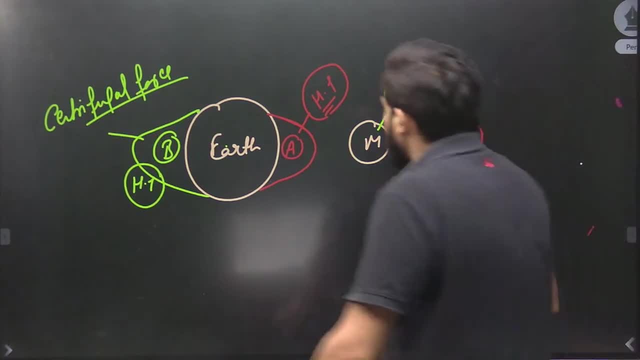 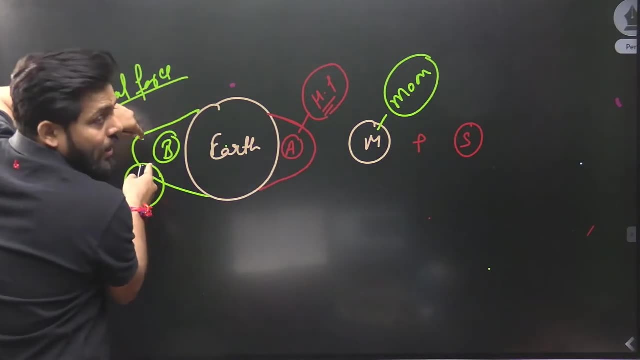 Now remember when the high tide will come at two places. then all the water of this part here has displaced and has come here. All the water here has displaced and has come here. So here at A and B, the high tide has come. 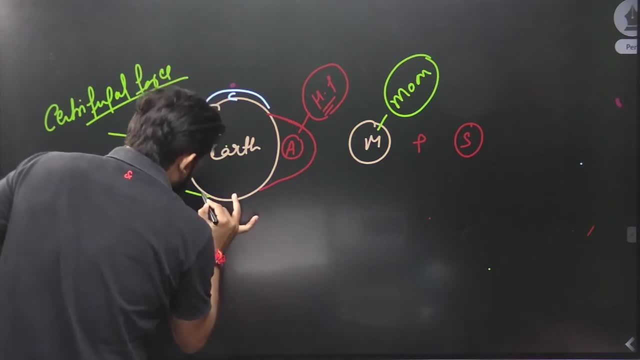 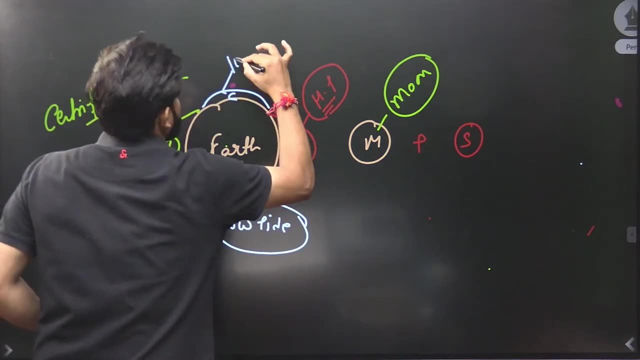 At the same place: this area, this C, and here, this D. here will come your low tide, Here will come low tide, Always remember. So this area will come low tide. So you have understood how this high tide and low tide come. 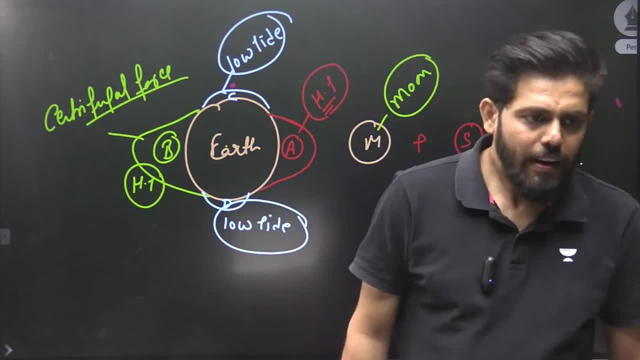 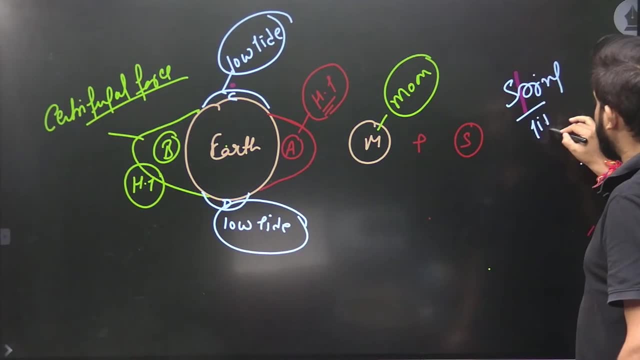 Ok. So always remember, whenever I tell you spring tide, spring tide means high tide. Whenever I say spring tide, if someone tells you when will spring tide come, you have to tell him when the high tide is, when spring tide is called. 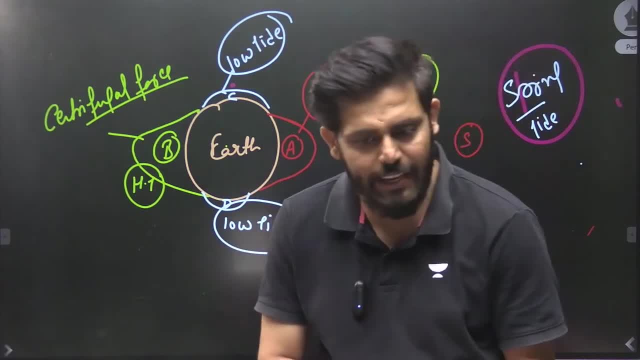 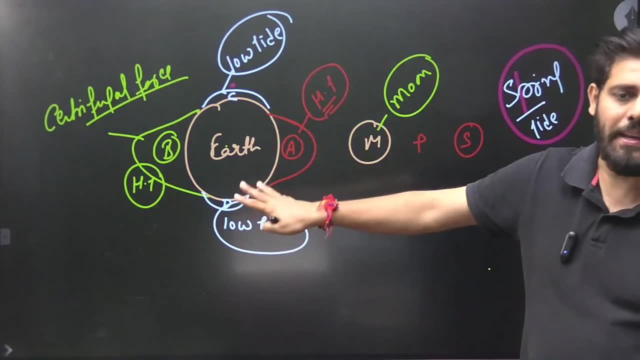 Ok, No one is in any problem. High tide and spring tide come very often. The spring tide comes when the high tide And high tide is the spring tide. Again, I am telling you this Tide, both are the same thing. I will clear all the concepts one by one. 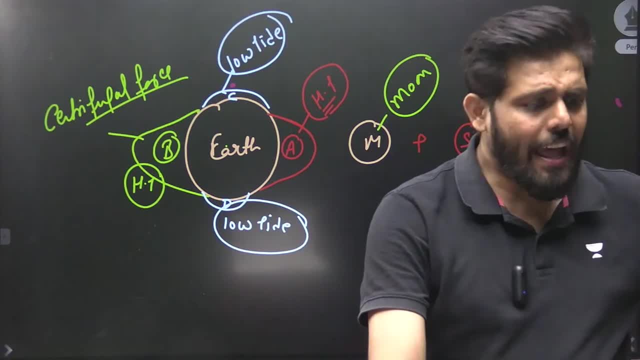 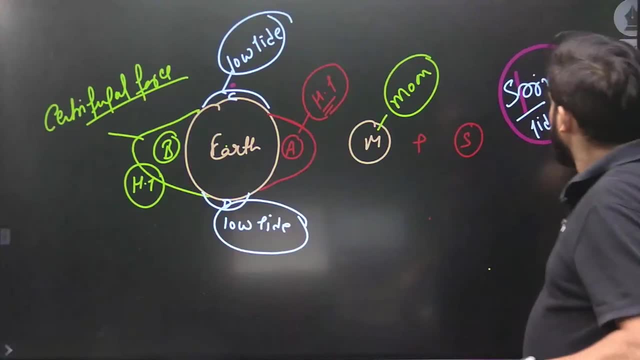 But till here, like share and remember all the strengths that you understood. Now, what did I tell you in the question? Quickly, whatever things I am telling you, you can write them too. Come here again Now. some things I will tell you. 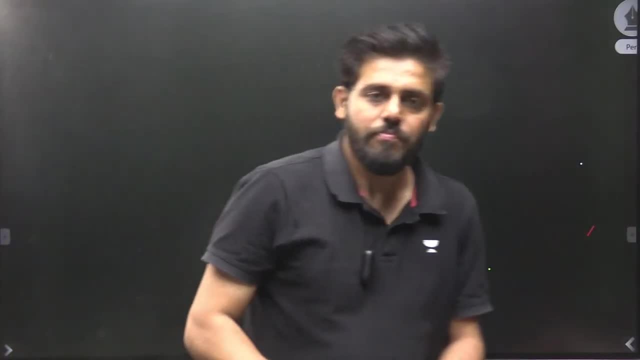 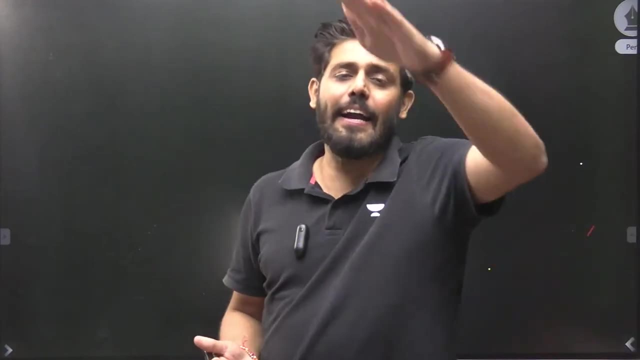 these questions will be asked in direct UPSC. Now let me tell you one thing Generally: where will the high tide come? more The highest high tide, the height of the tide. where will the high tide come? High tide means: 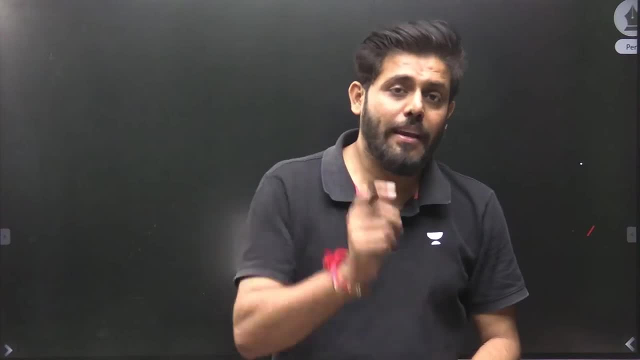 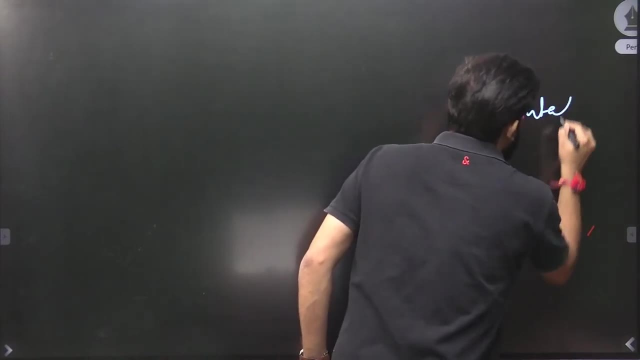 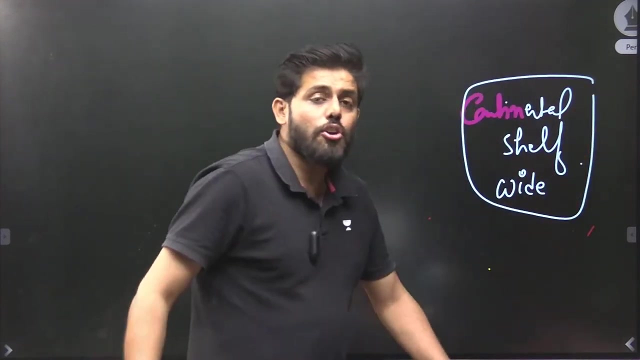 where will the height of the tide come more? Always remember that area: where the continental shelf will be wide. in that area the high tide will come most. Why? Because if the continental shelf will be wide, then it means this area. 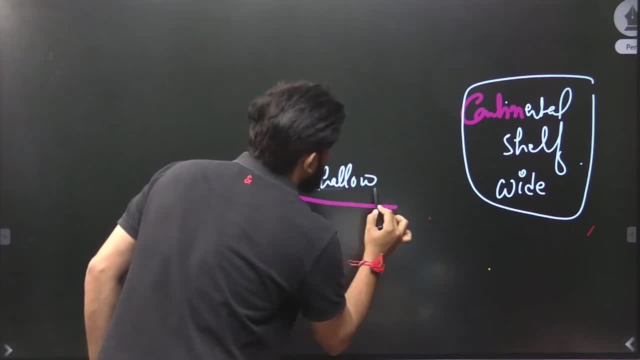 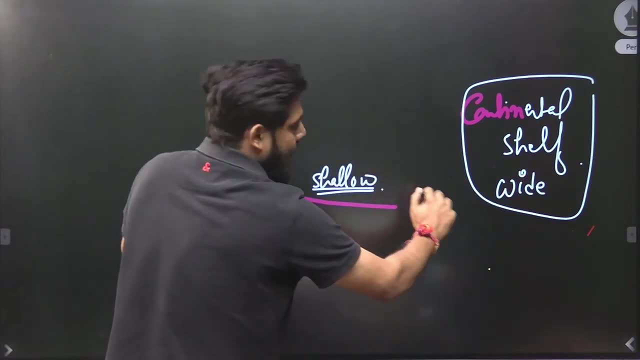 this shallow area here because the depth of the continental shelf is not much, so it is a shallow area, So here the water level is more, but it is getting less area, due to which it will rise more upwards. 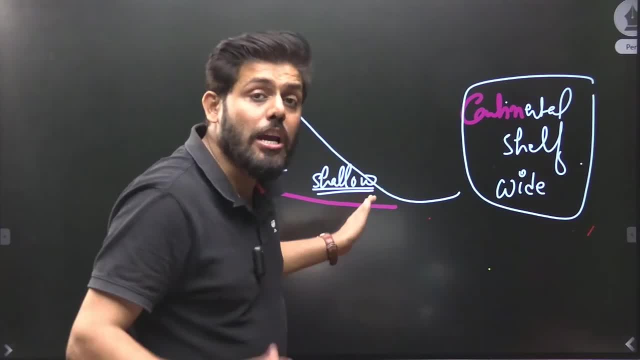 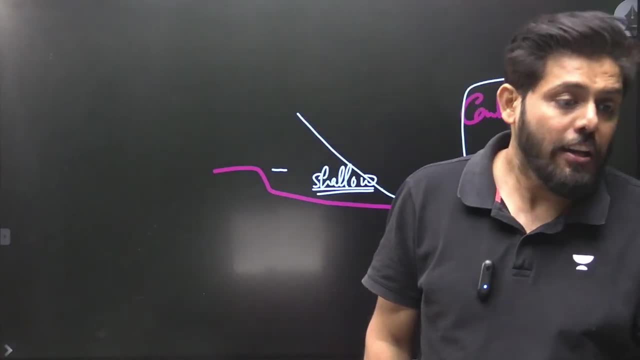 So that means that area where the continental shelf is wide, there the high tide generally comes more in height. Always remember this thing. Always remember this thing, Or any such point, which is Bay and Estuary. try to understand. 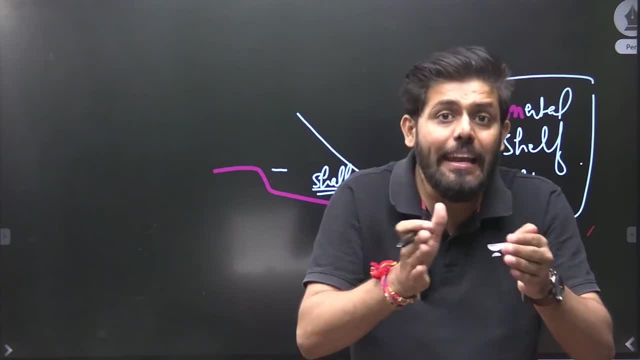 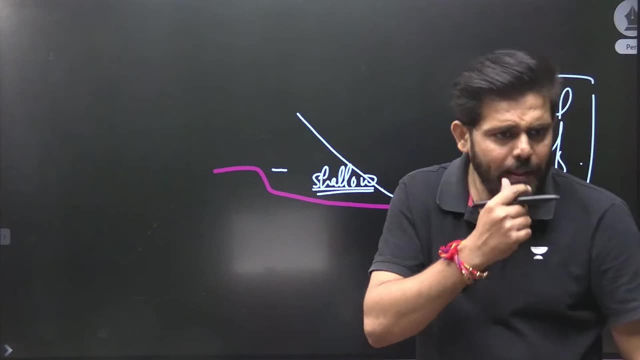 such a point where the Bay and Estuary, where the Estuary is, where the inlet is narrow, at that point also you will get to see the high tide. Remember these things too. Now I will give some examples of all these things. 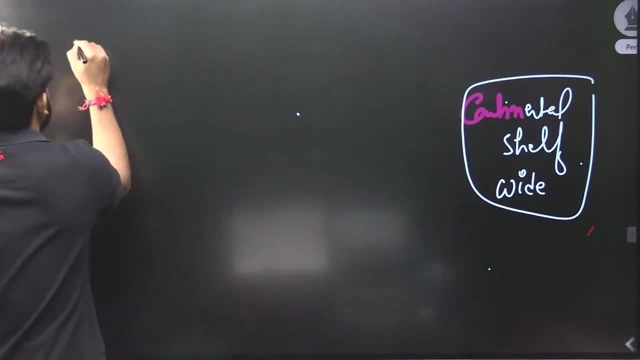 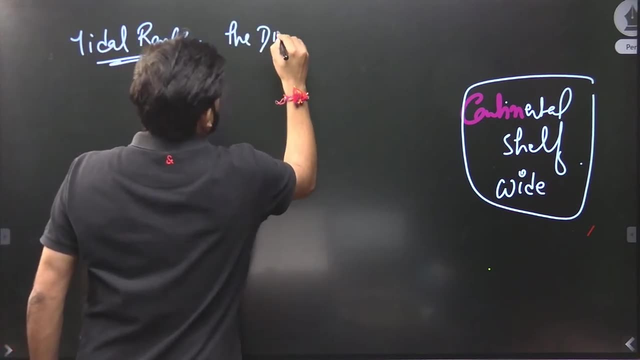 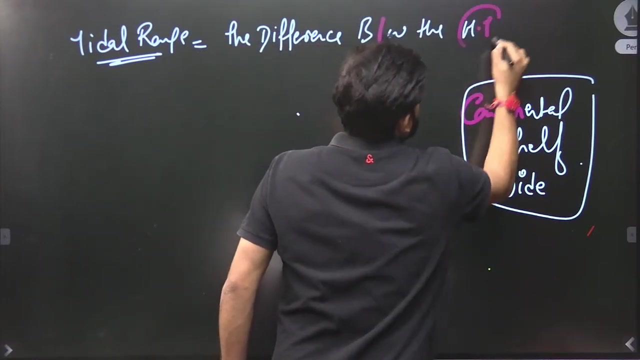 So, first of all, if you ask yourself what is tidal range, If you ask yourself what is the tidal range, So first of all tell me the difference between the difference between the high tide ht and the low tide. The low tide and the high tide. the difference between them is called tidal range. Remember this: The difference between the height of the high tide and the height of the low tide. The difference between the height of the high tide and the height of the low tide. 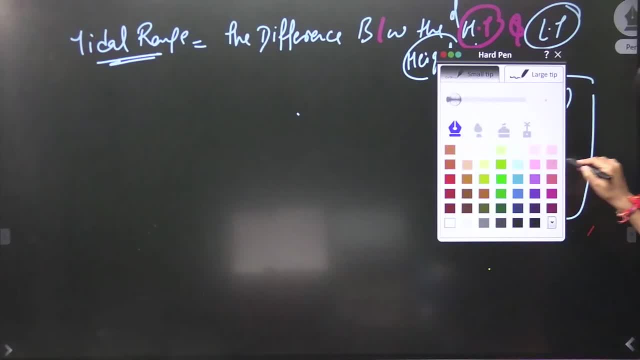 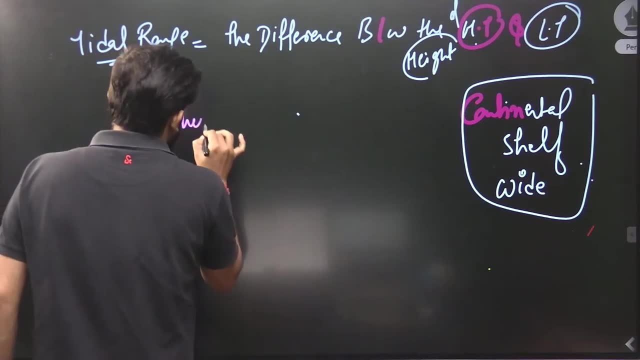 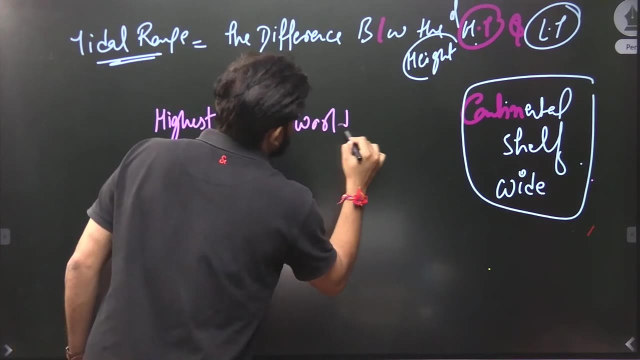 the difference between them is called the tidal range. Now the second point is another, a very good one. If I ask you a question that the world's highest, highest, Which area of the world is the tide of the world, Your answer should be the Bay of Fundy. In the Bay of Fundy the world's highest high tides occur, whose height is very high, which is in Canada. The Bay of Fundy in Canada is where the world's highest high tide occurs. Did you understand? Now, if someone asks you where will India's highest high tide come? 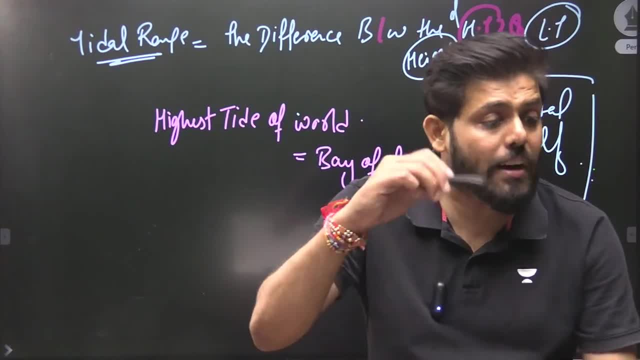 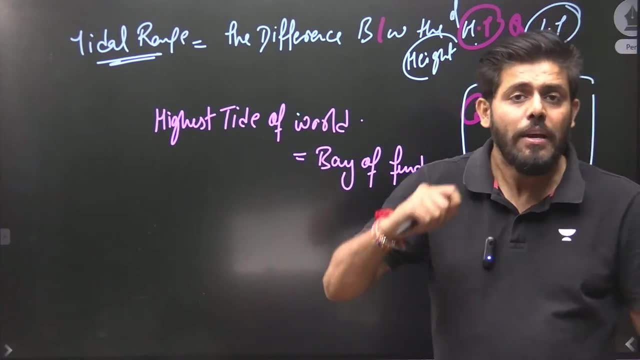 Where will India's highest high tide come? I will try to clear your conceptual clarity. In Canada, the highest high tide comes on the Bay of Fundy. If I ask you where will India's highest high tide come, Someone will answer me. go to tomorrow's class once. 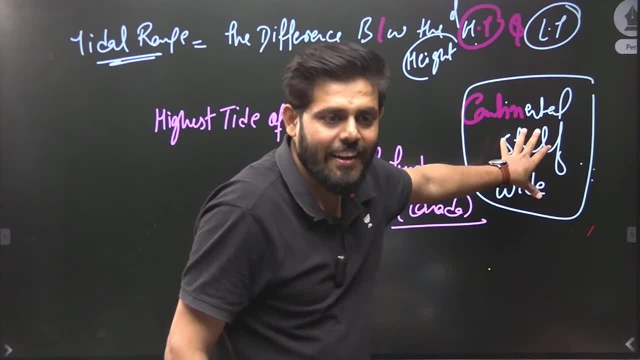 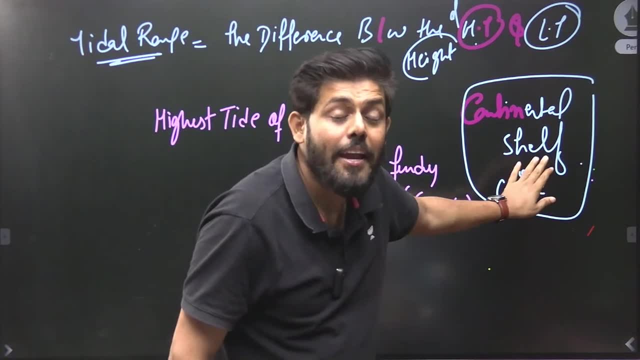 Go to tomorrow's class and come here, Come here, here, here. What did I tell you? Where is the most wide continental shelf in India? What is the state on the western coast? What is the state? Some students are absolutely right. 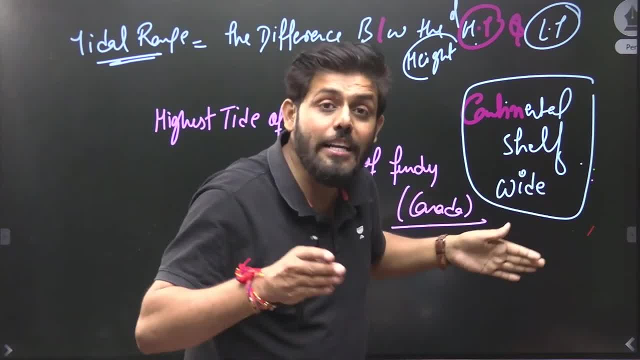 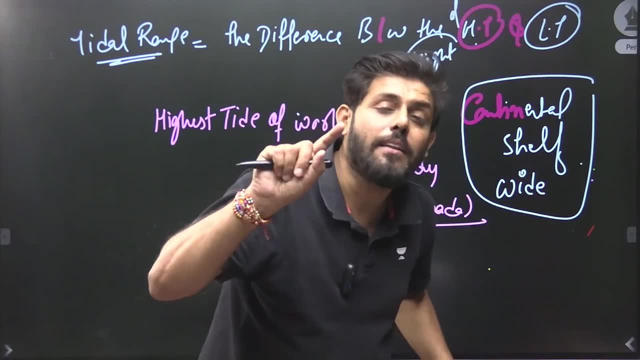 In Gujarat the most continental shelf is wide. If the continental shelf is wide, then in which area? Not the Kutch region, but the Gulf of Khambat. Strictly mention the Gulf of Khambat And you can say the Gulf of Kembe. The Gulf of Kembe and the Gulf of Khambat are the areas where the highest high tide comes in India And, remember, in India where the most tidal energy is produced and the most stations are installed. which area is that? The Gulf of Khambat, region of Gujarat. 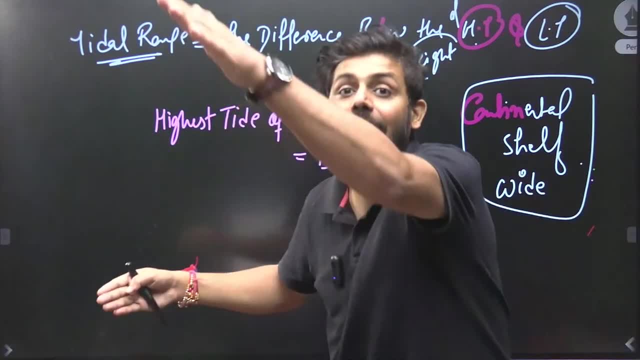 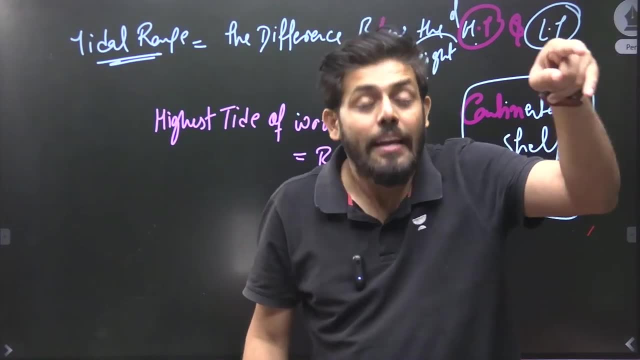 Why? Because the continental shelf is wide. If it is wide, then the high tide will come. So which state is the most important for tidal energy? Gulf of Khambat, Gujarat state? Okay, Remember these things. West Bengal is also there. But where have the questions been asked? Gujarat, Where Gulf of Khambat. And the Gulf of Khambat is in Gujarat. The name of that place is Highest High Tide in India. Highest High Tide in India. Where is it? 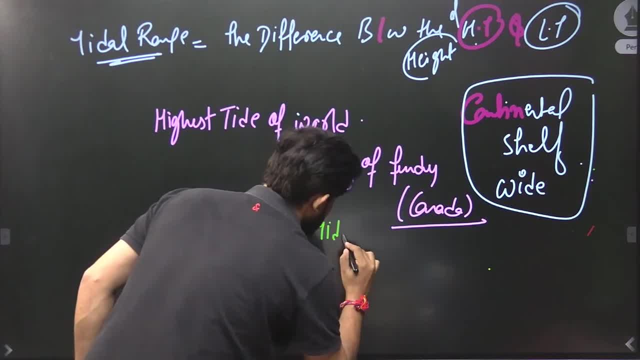 In the Gulf of Khambat. And where is this Gulf of Khambat? guys, Here is your Gujarat coast And there is a place here. The name of that place is Okha, Okha, Okha. This Okha is a place. 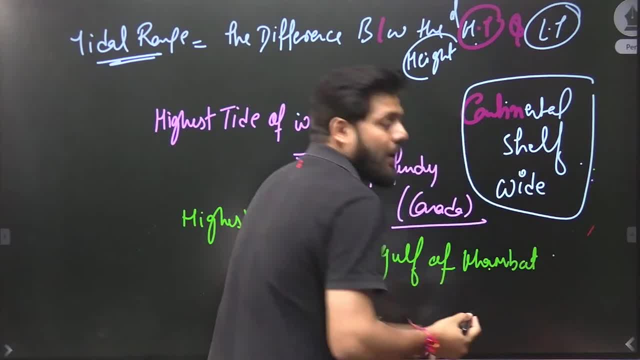 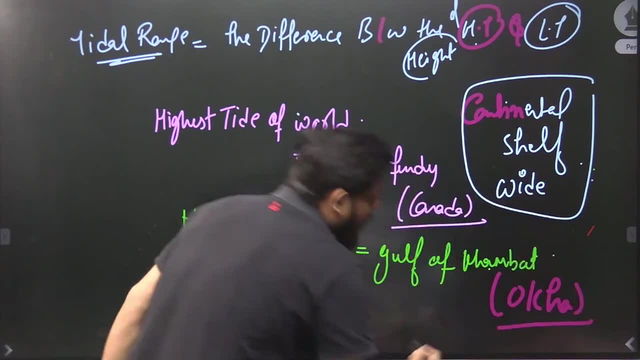 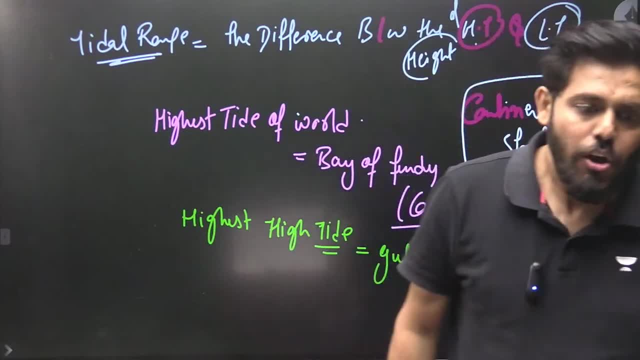 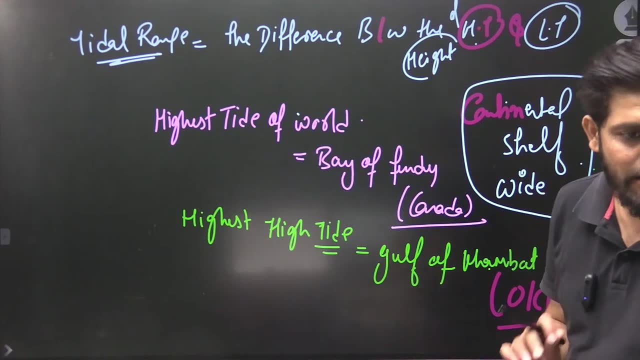 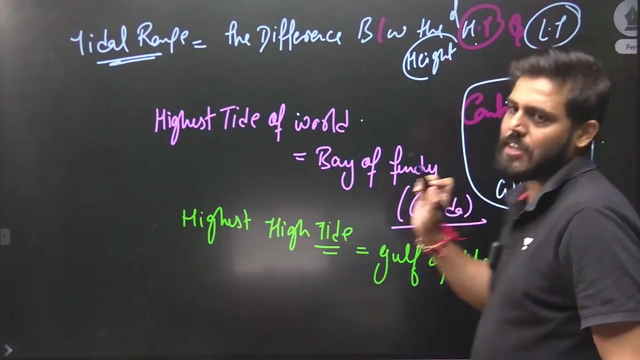 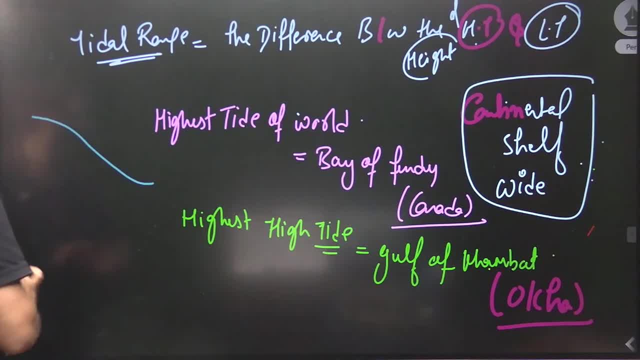 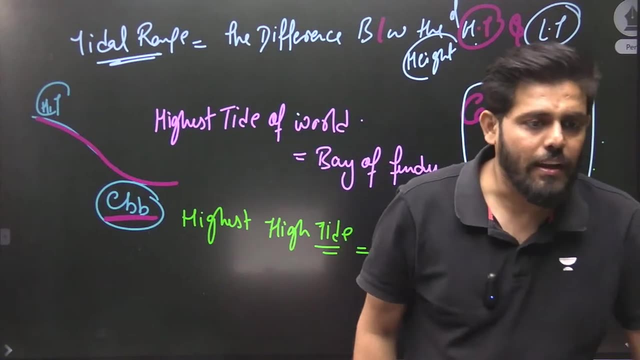 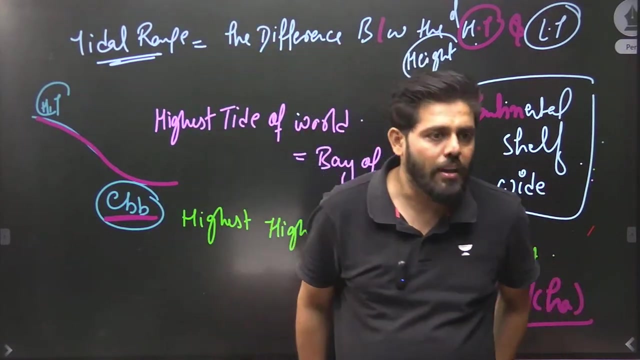 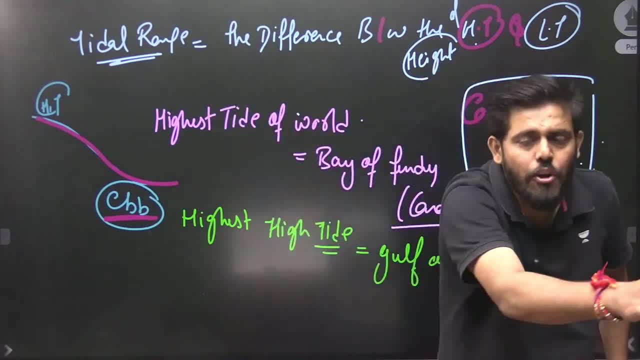 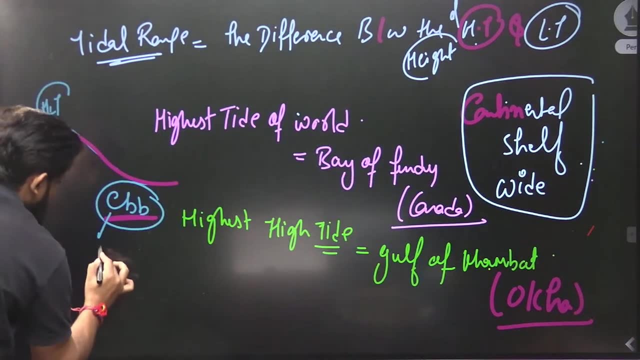 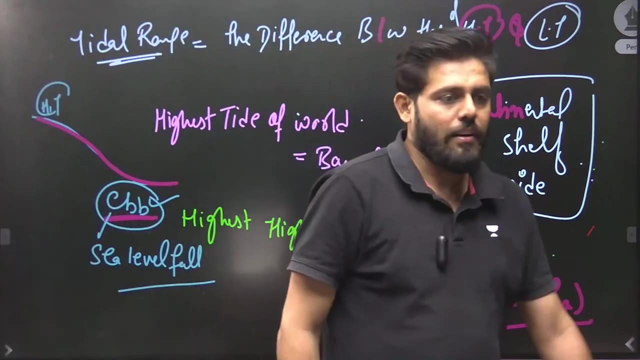 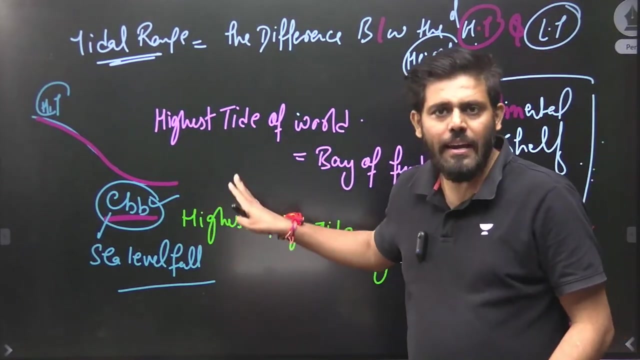 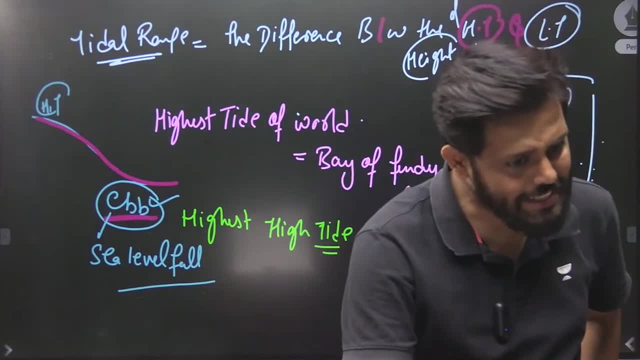 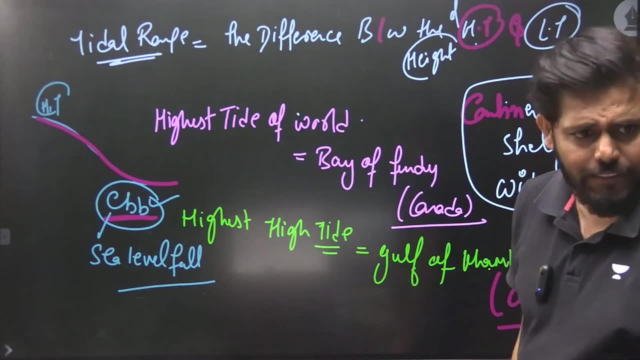 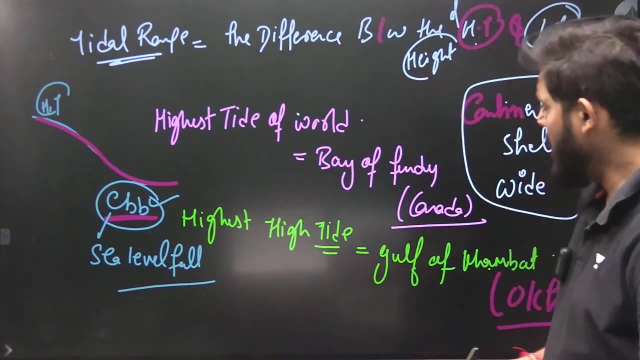 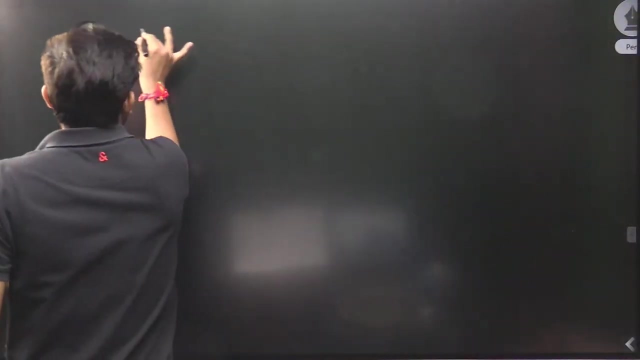 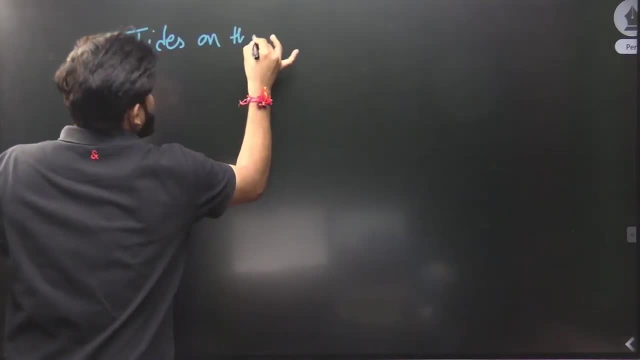 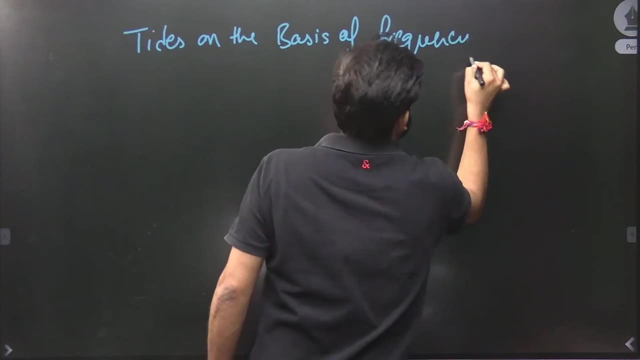 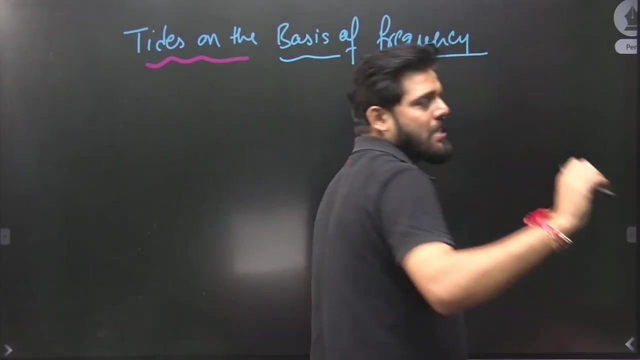 Tides on the basis of frequency. See guys, some students might be thinking, Sir, one or two things are missing. See guys, If I talk, I am taking it to the maximum level, to the maximum level that it is possible to give the best content for free. 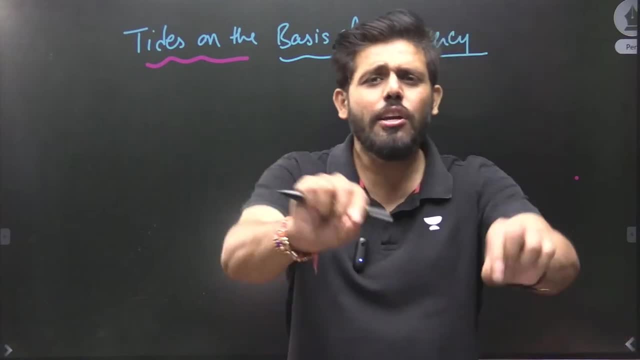 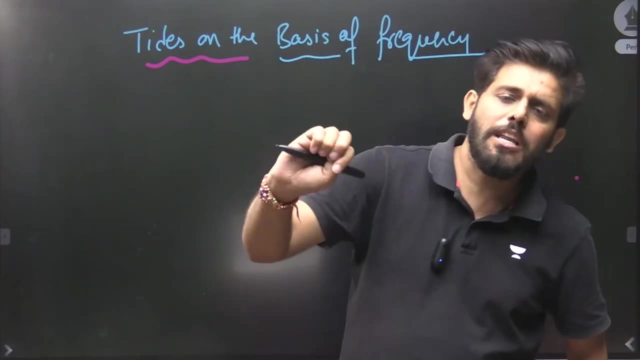 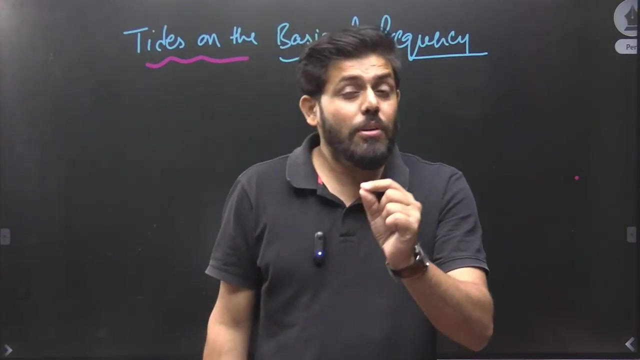 But there are some things that one topic is complete, Some things are missing when the course is so wide. But when you do things through subscription, there is a course sheet that is in more detail. I promise that I never leave things from my mind. I promise from my end. 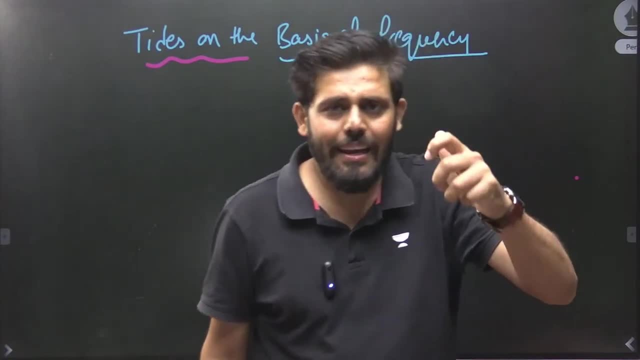 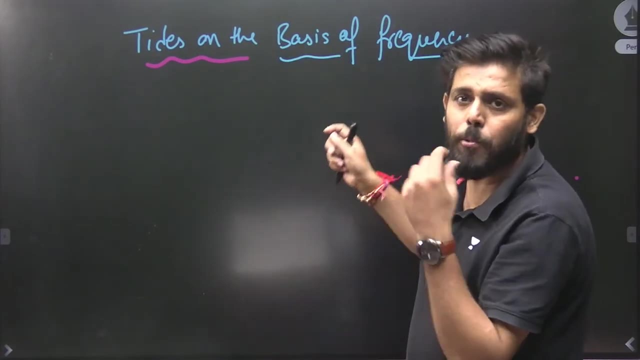 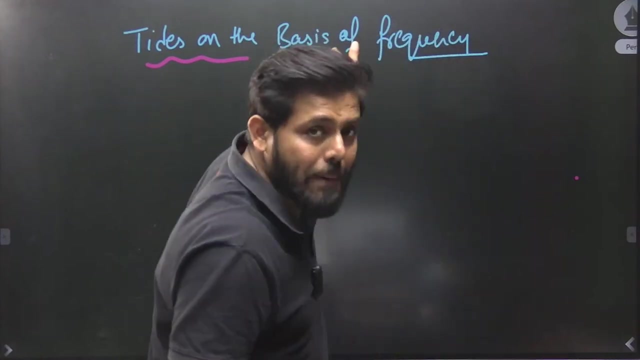 that, whatever comes in my mind, I am never bringing things by writing Here. I am not teaching by looking at PPT. Who knows some things in PPT? And there are so many things that I am saying. Always remember that I have a very important point In the question class. 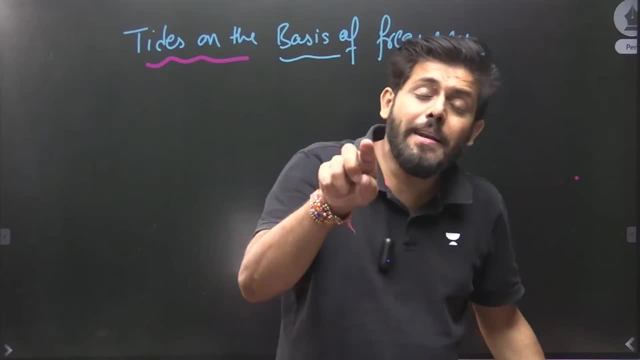 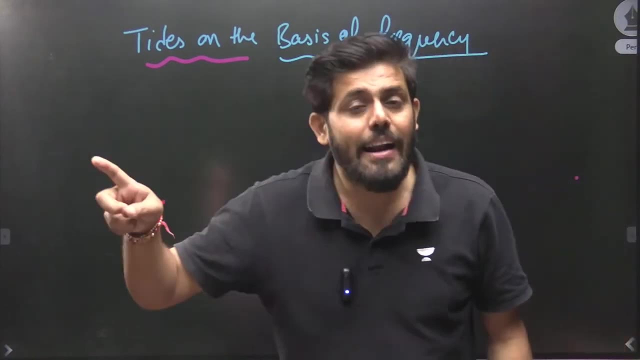 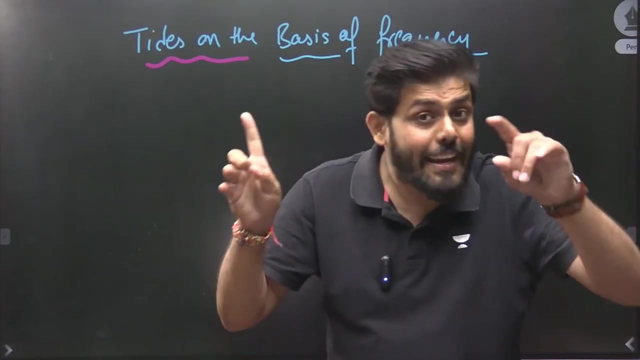 whatever I am writing from here, these questions will be asked, But there are chances that I am asking from mouth. There are so many things that I am asking from mouth but I am not writing. There will be questions directly, Because I told you that continental shelf is wide. 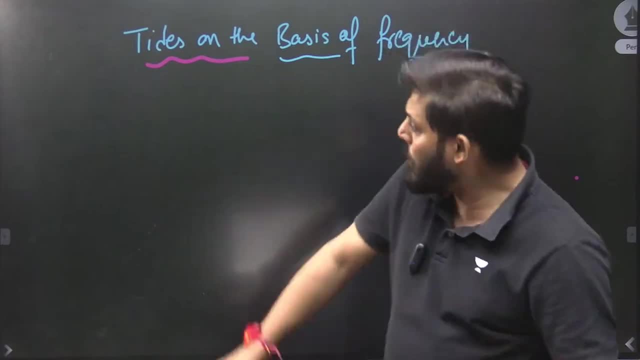 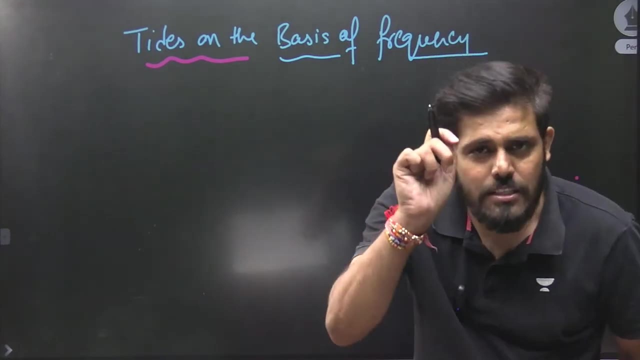 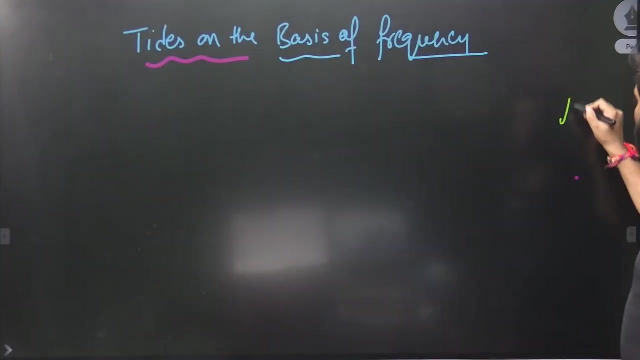 There will be more high tides So you have to link things. I will not make you write, But you have to link automatically. There will be more questions, So keep your mind and notes And all these things you get on subscription. If you are interested, You can purchase using AM10 code. 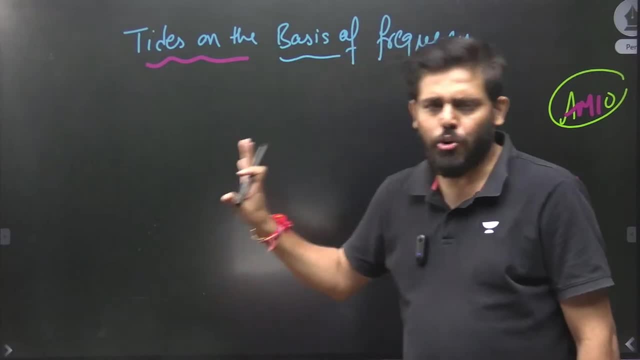 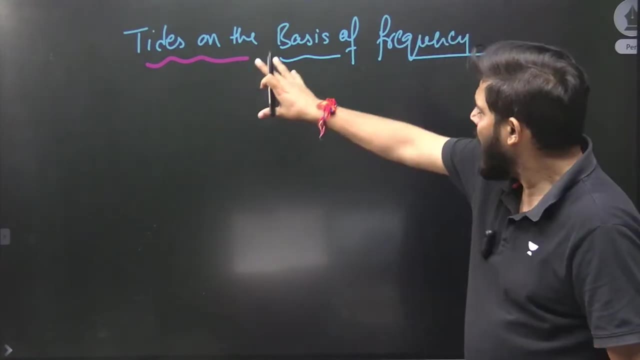 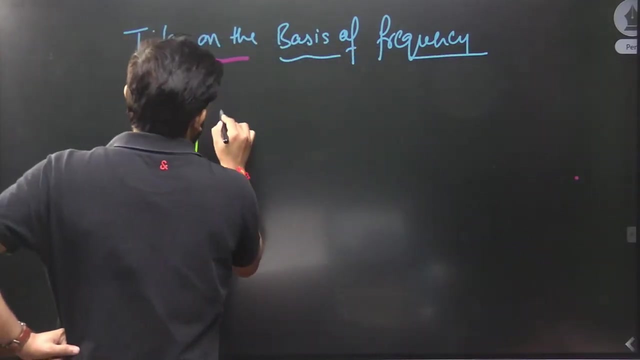 For those who want. Otherwise, I am trying to give maximum content on YouTube from my end, But if in detail, All subject options. Now we will talk about tides on the basis of frequency. What are the tides on the basis of frequency? First of all, we will talk about 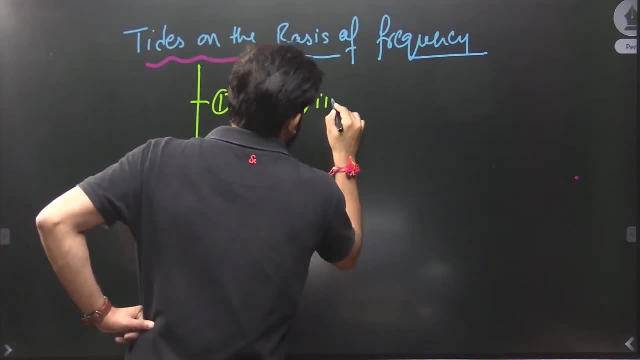 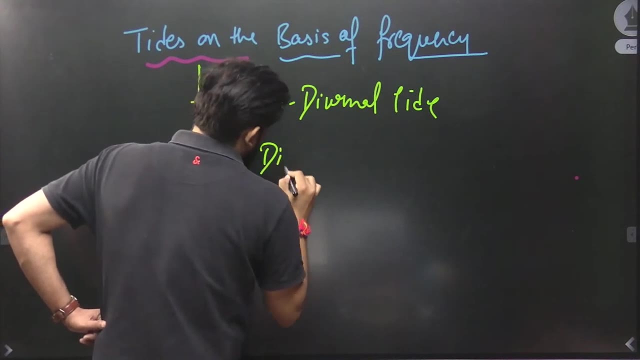 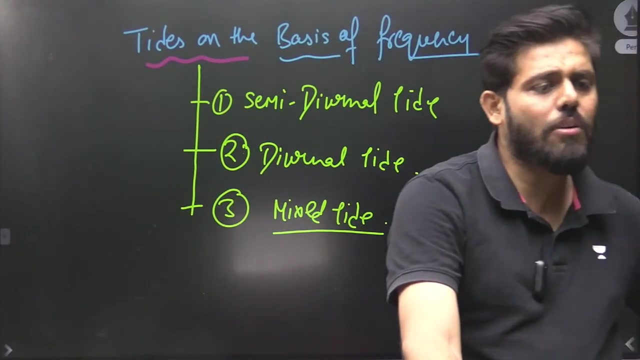 Number 1 Semi-Diurenal Tide- Semi-Diurenal Tide, And then Number 2 Diurenal Tide, And then Number 3 Mixed Tide. Mixed Tide. These are tides on the basis of frequency. On the basis of frequency, We have classified these tides. 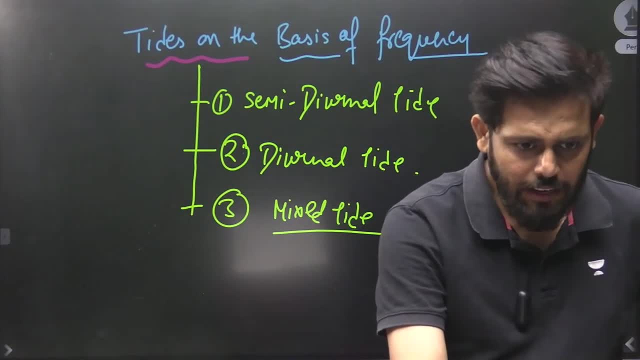 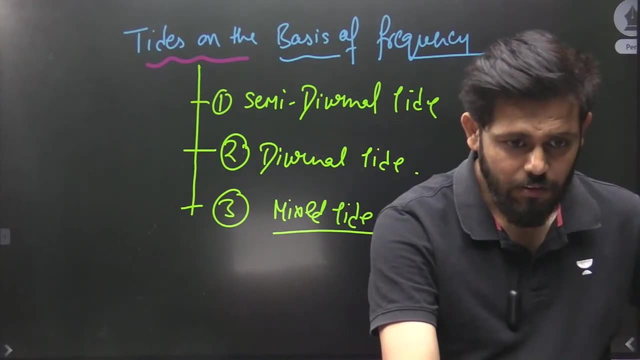 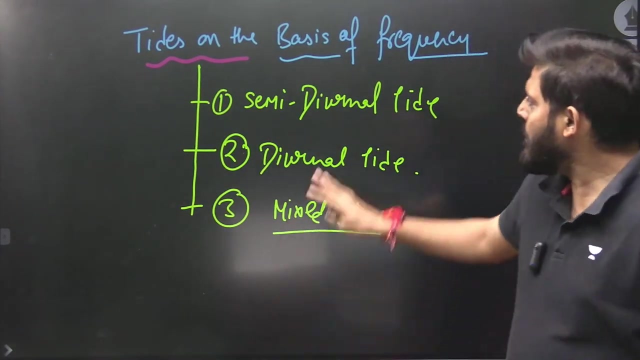 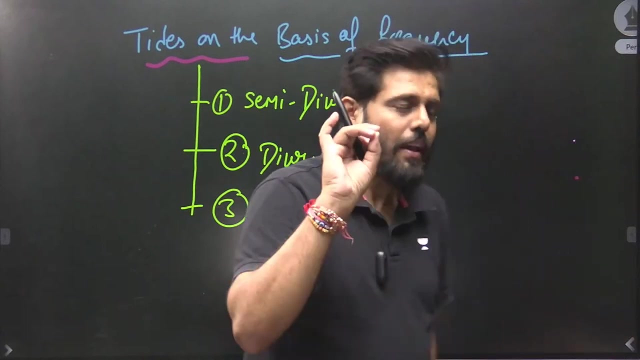 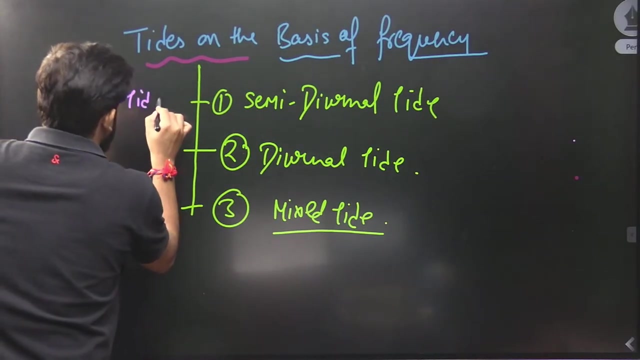 Which tide comes. how much On that basis, Ok, Ok, Ok. So we have talked till here. Ok, Now I will talk about Semi-Diurenal Tide. What is Semi-Diurenal Tide? Listen very carefully, Listen very carefully. In a day, Two high tide And Two low tide. 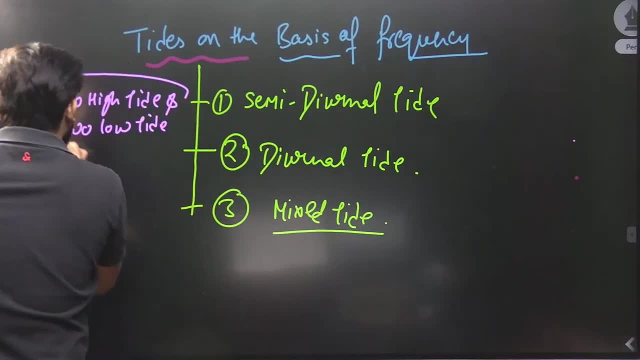 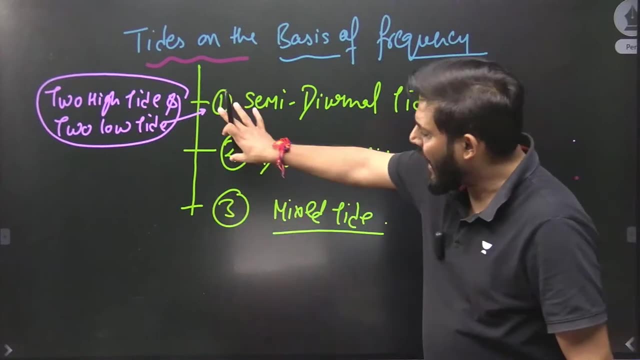 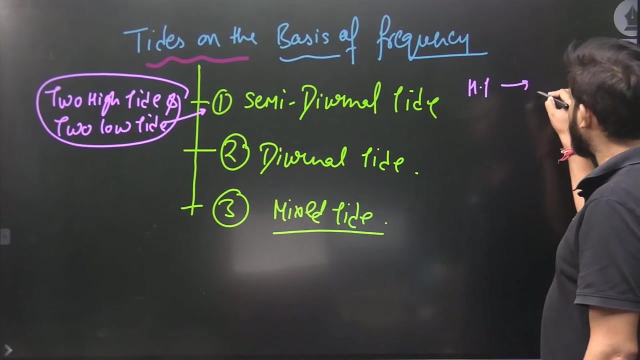 When, in a day, Two high tide and two low tide come, It is called Semi-Diurenal Tide. In a day, Two high tide and two low tide come, And remember How these two high and two low tide will come. Suppose one high tide came, Then the second high tide. 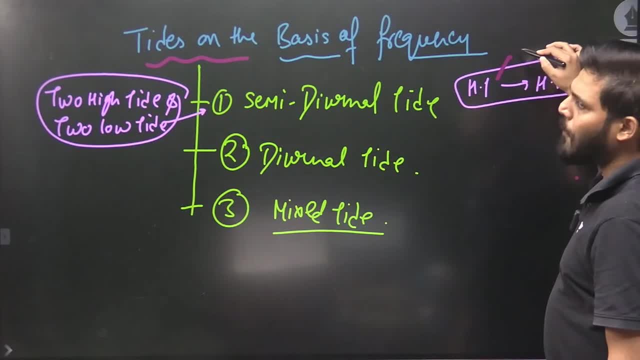 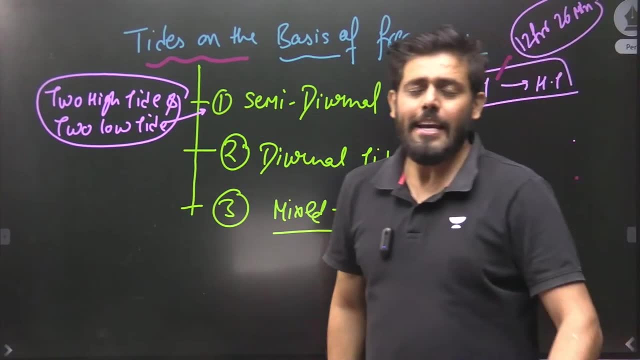 The gap between it, That is Aprox 12 hours and 26 minutes. 12 hours and 24 minutes. There is a difference of 12 hours and 24 minutes In this generally. what happens When the moon revolves? Then it does not revolve in 30 days. The time period of the moon to revolve. It does not revolve in 30 days. How long does the moon do? In 27 days. So because of this, This time does not come in 12 hours. It comes in 12 hours and 26 minutes. In 12 hours and 26 minutes. Then, after one high tide, The second high tide That will come after 12 hours and 26 minutes. Remember these things. So the time between the two high tides: After 12 hours and 26 minutes, One high tide. 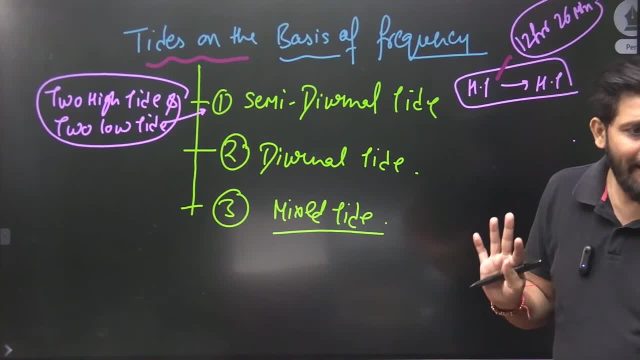 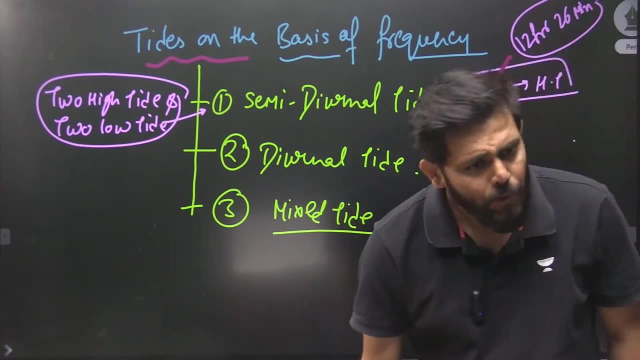 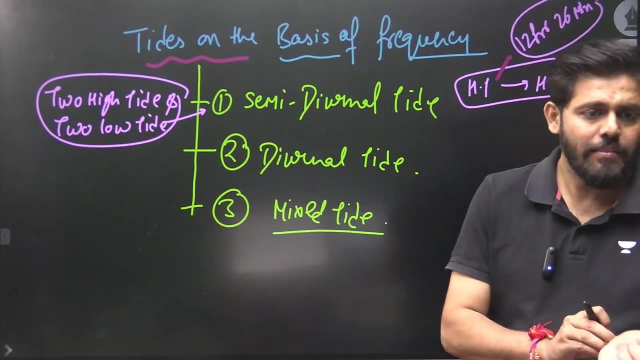 Then your second high tide will come Understood. Is it clear? If anyone has any problem, Then tell me quickly. Anyone of you. Sir, I have this problem. Okay, Now I will tell you one thing. Very good example. There is a place in England You must have heard of, Southampton. 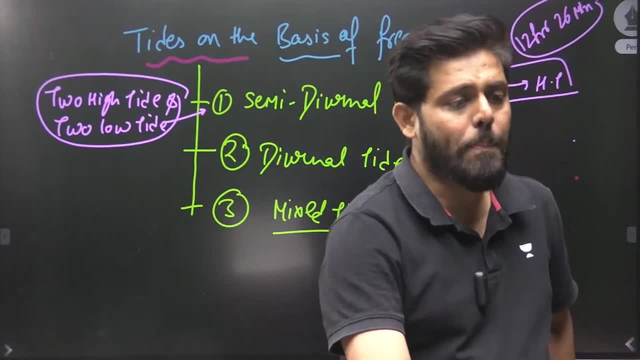 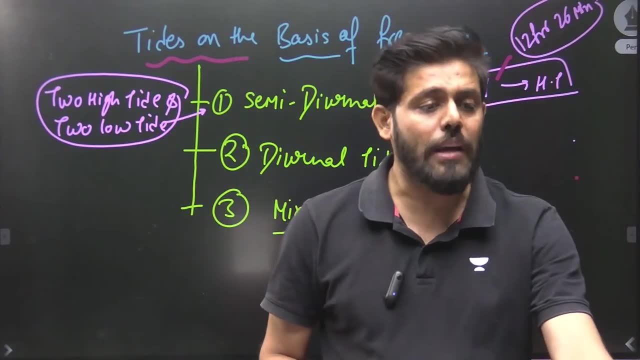 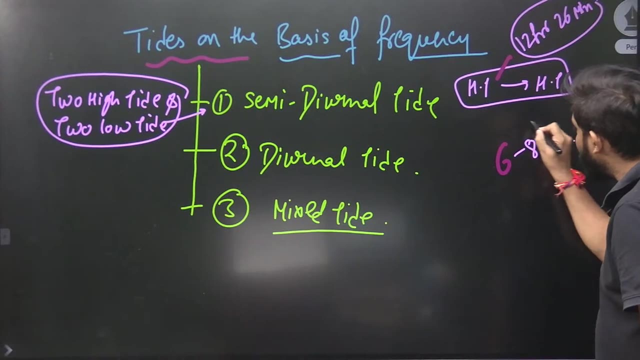 Those who watch student cricket, They will know. Those who watch student cricket, They know. There is a place in England, Southampton. You must have heard about Southampton. How many students have heard. Southampton is such a place Where tides come six to eight times a day. Tides come six to eight times. 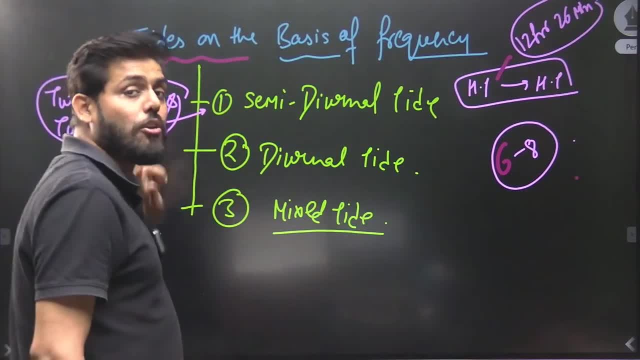 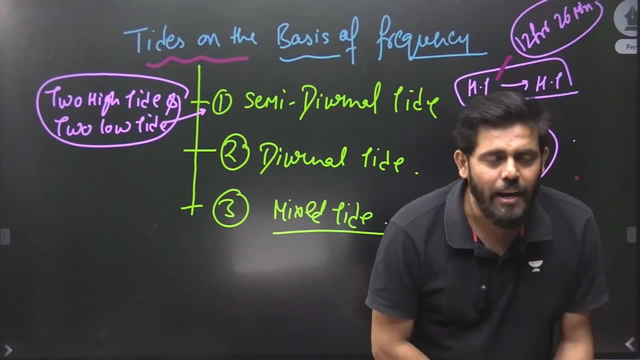 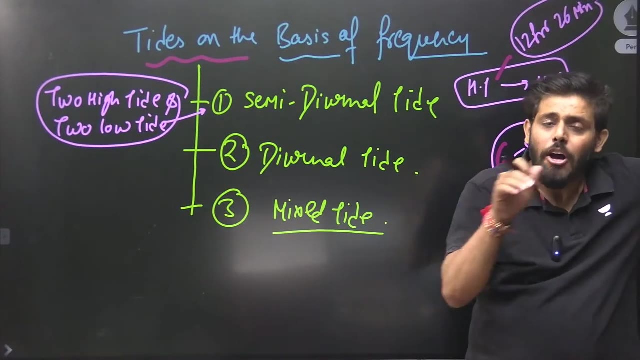 I have told the semi diurnal That two high tides and two low tides- There are six to eight times Tides come here. If you look at the location of Southampton, There is English Channel, There is North Sea, There is English Channel and North Sea. So what will happen? There will be two high tides From the English Channel region. Two high tides will come from the North Sea area. Two neap tides Will come from the English Channel area. So your Southampton. There are six to eight times tides. There are six to eight times tides. 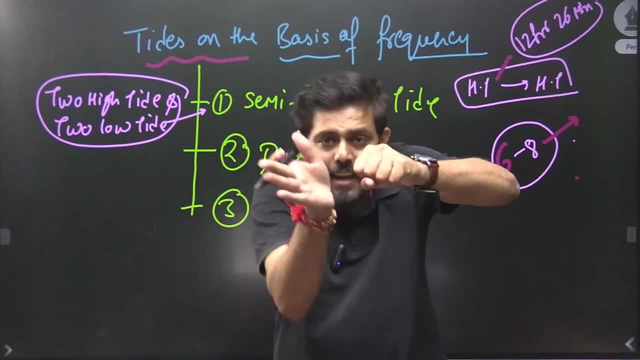 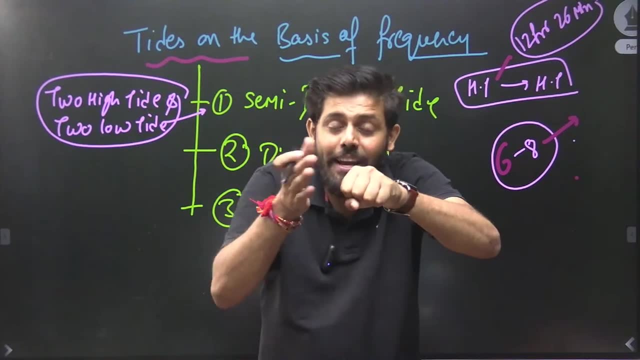 There are six to eight times tides. The reason is that this is Southampton, So in Southampton, This area is English Channel And this area is North Sea, So this area is also influenced And the English Channel is also influenced, Due to which there are more high tides. And low tides. So the question can be: Which area has more high tides And low tides? After that comes diurnital tides, After that comes diurnital tides, Semi diurnal, Two high tides And two low tides. What is diurnital tides? 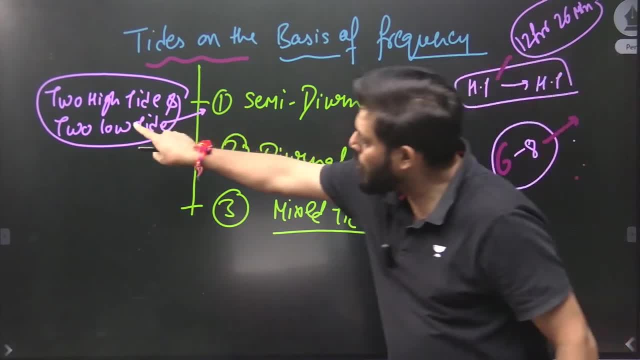 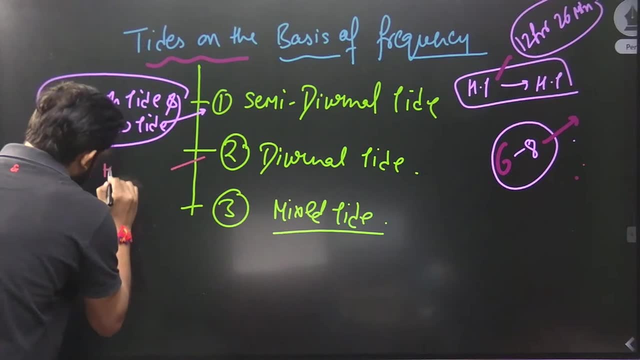 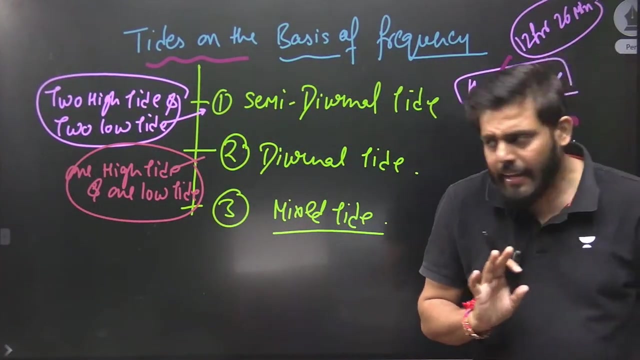 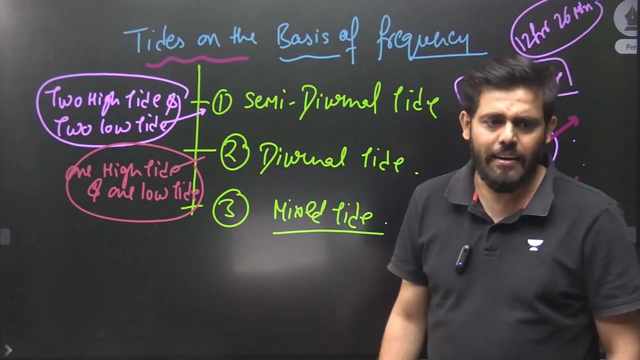 Diurnal tides: One high tide And one low tide, One high tide, One low tide, One high tide And one low tide For a day. One high tide and one low tide will come in a day. The height of one high tide and the height of another high tide is almost the same. 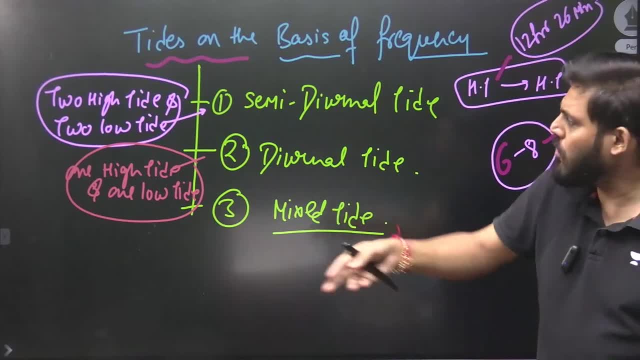 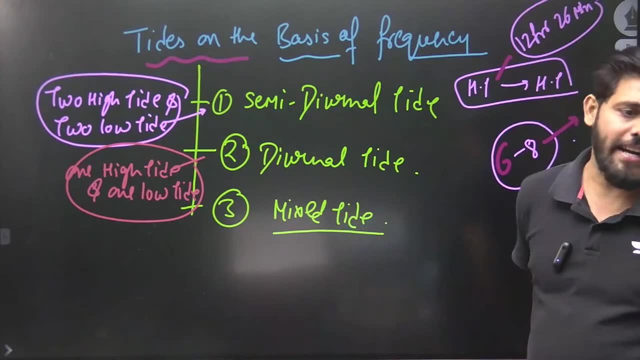 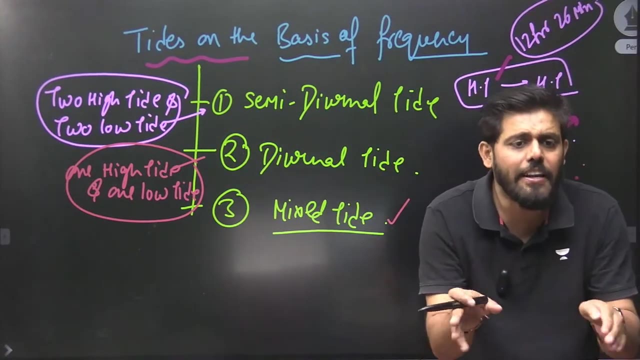 That means one high tide and one low tide. That is called diurnal tide. Did you understand? Is it clear? Okay, Next comes mixed tide. What is mixed tide? The variation of the height of the tide is mixed. That means the variation of the height of the tide. 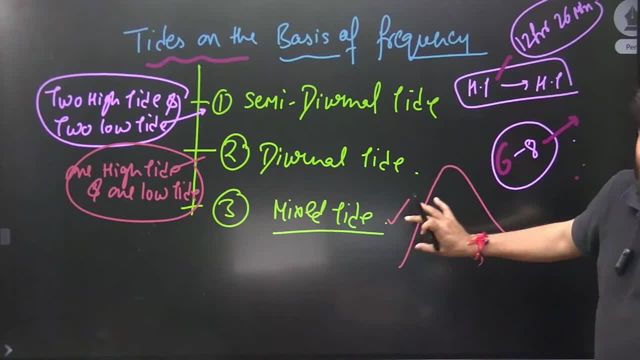 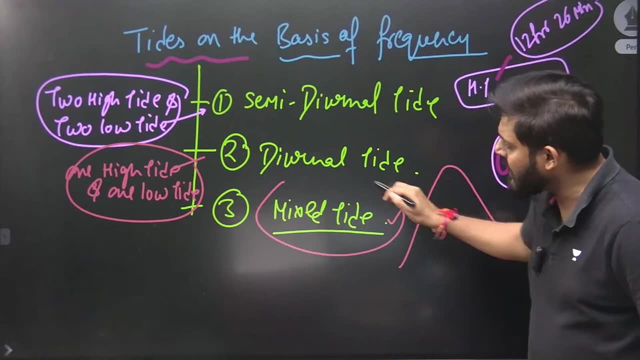 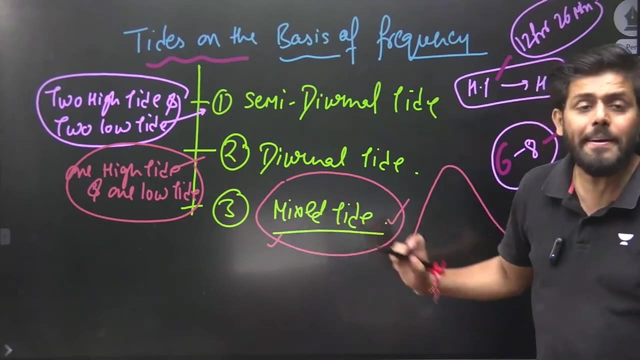 It doesn't matter if it is high or low. There are variations in the height of the tide. Sometimes it is high, sometimes it is low. The height is not fixed. The variation of the height of the tide is called mixed tide. Where can we see it? 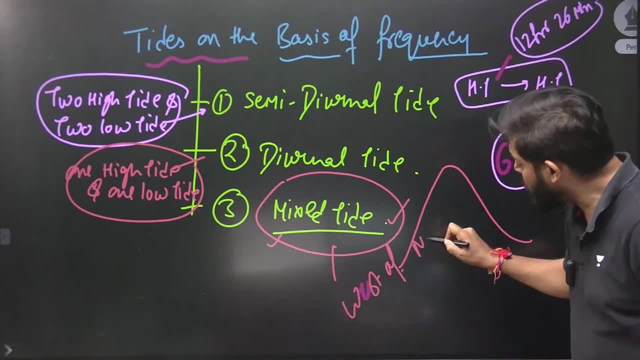 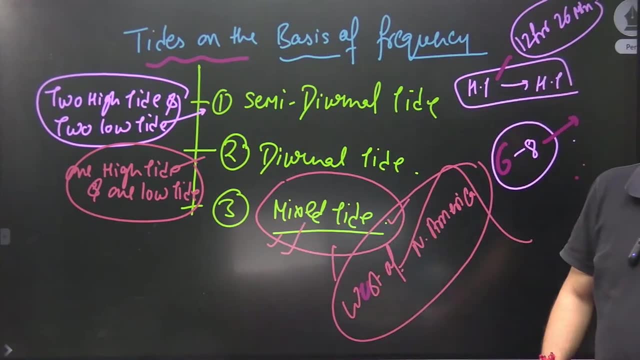 West coast of North India, North America. In the west coast area of North America the height of the tide can be seen as a variation. That is called mixed tide. That means the height of the tide is not fixed. There is a variation in the height. That is called mixed tide. On the basis of frequency, there are three types of tides: Semi-diurnal, That means two high tides and two low tides in a day. Diurnal tide: One high tide and one low tide in a day. 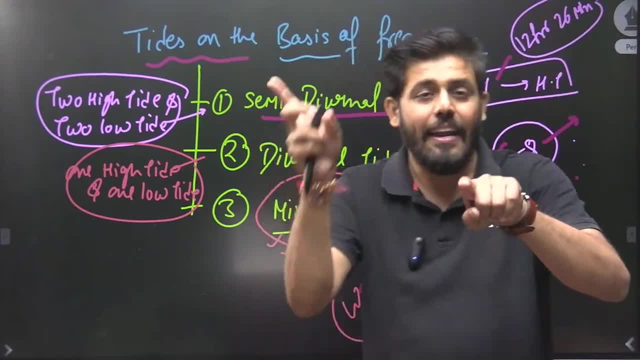 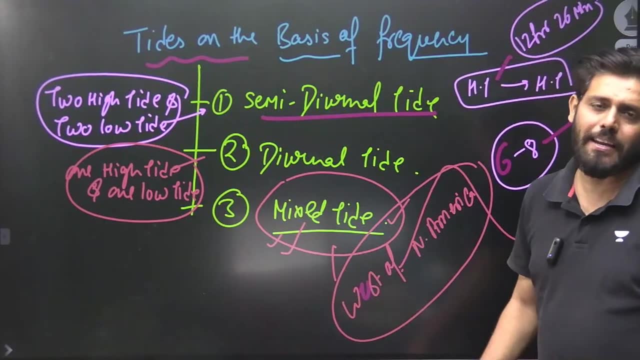 If you put semi in semi it becomes two high and two low In diurnal, one high and one low In mixed. the height variation is on that basis. Where In the west coast of North America How many students have cleared everything so far? 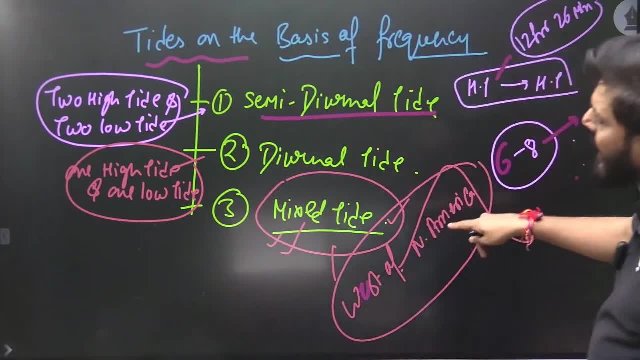 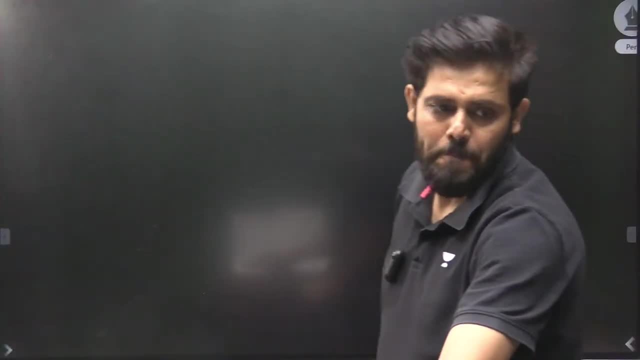 Now I will teach you everything one by one. I will teach you about spring tide, I will teach you about neap tide, I will teach you about tidal bulge, And I will explain everything. well, I think you must have cleared everything so far. 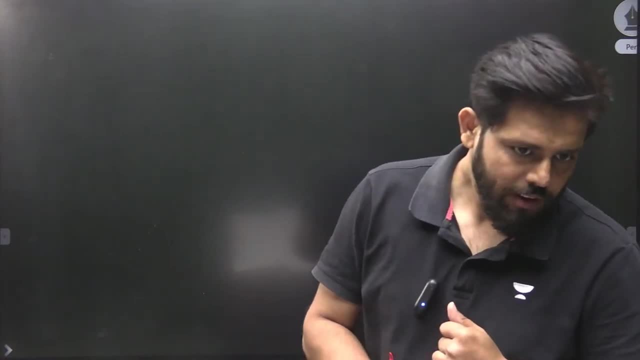 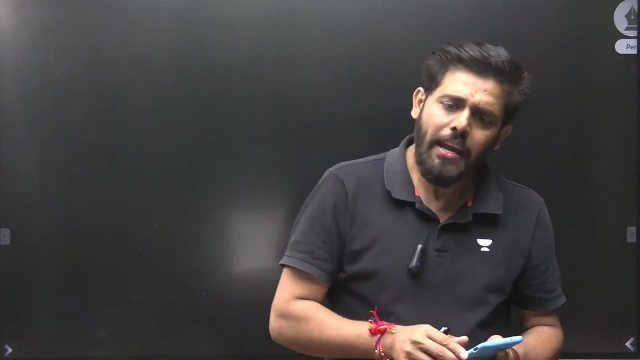 Is it clear? Yes, Variation in tide. Absolutely, Each and everything is clear. Like and share. There is a topic of 10 to 15 minutes more, Then we will finish. it Is it clear? I hope you have cleared everything so far. 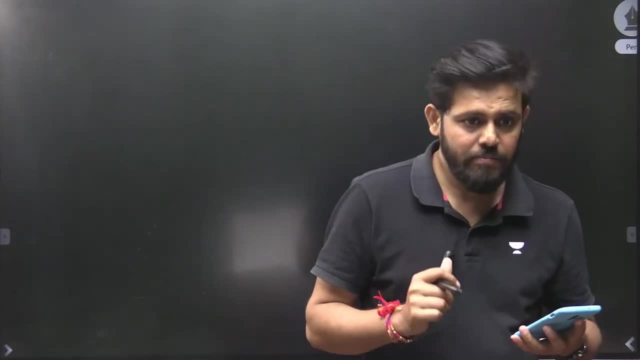 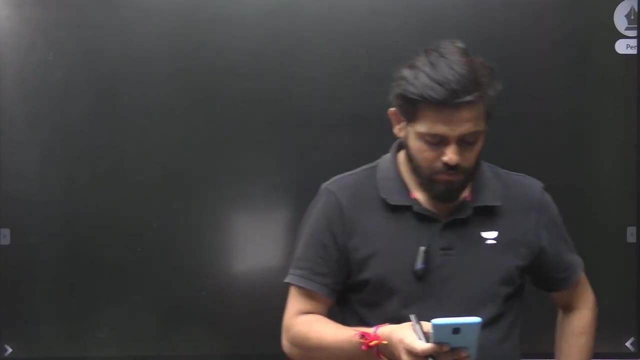 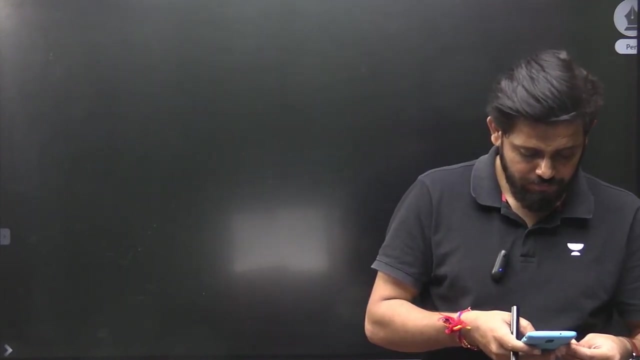 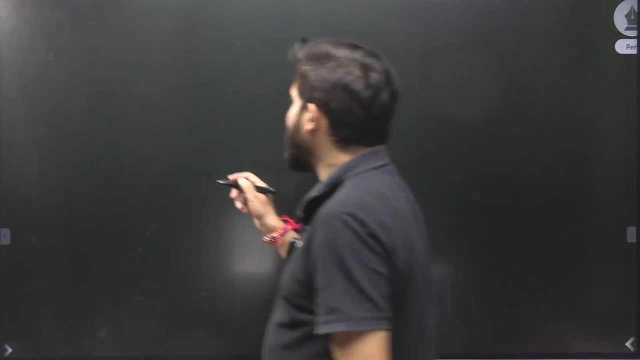 Everyone must have cleared everything. We will move ahead and do things in detail. Okay, Just give me one minute, Okay. Okay, Let's move ahead. This is done. Okay, Let's move ahead. Let's talk further. First of all, I am talking about types of tides. 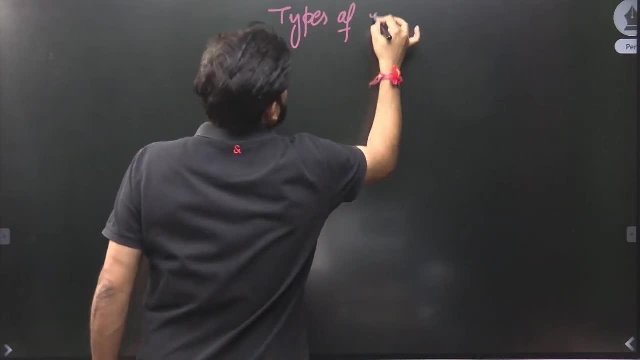 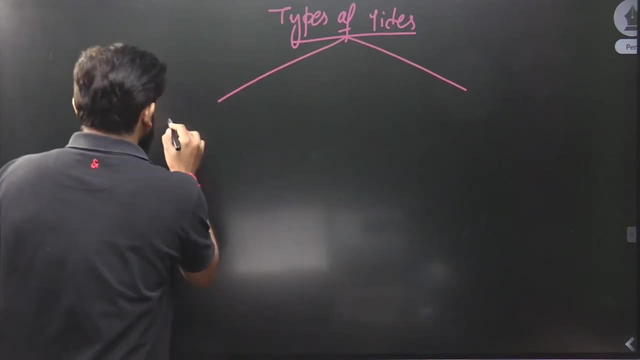 Types of tides. Till now, I have talked on the basis of frequency. On the basis of frequency. Now, on the basis, what are the types of tides? First comes spring tide- Spring tide- And on the second number comes neap tide. 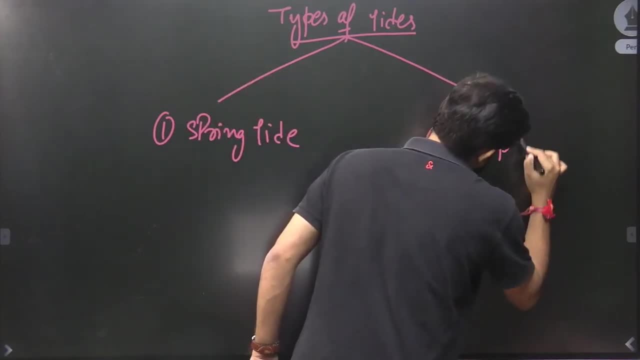 And remember this same spring tide is called high tide And this same neap tide is called low tide. Till now, we had taught the concept of high tide. Now I will teach you the concept of low tide. How does it happen? 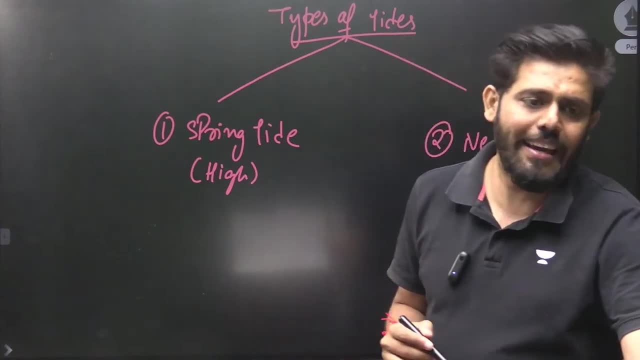 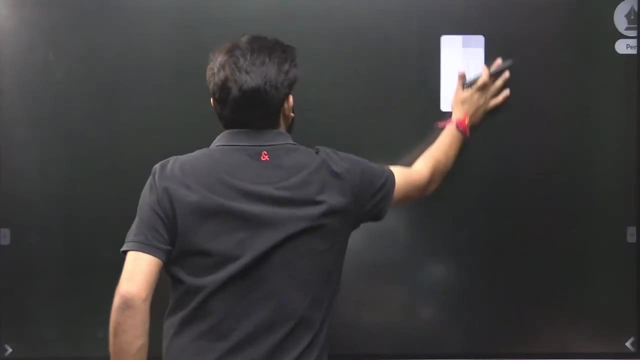 What is the whole reason behind it? What is the concept, One by one. So, first of all, I will bring the spring tide in front of you once again, so that you can understand things in a better way. Here, spring tide is written on the basis of frequency. 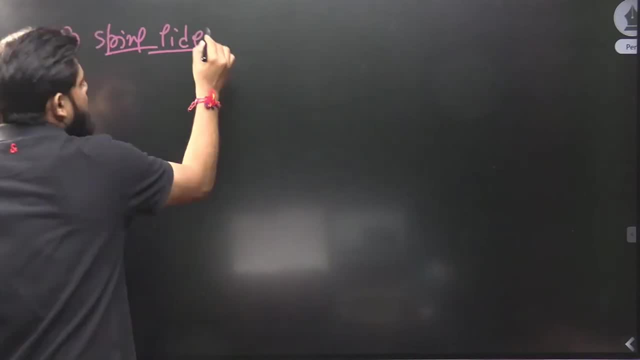 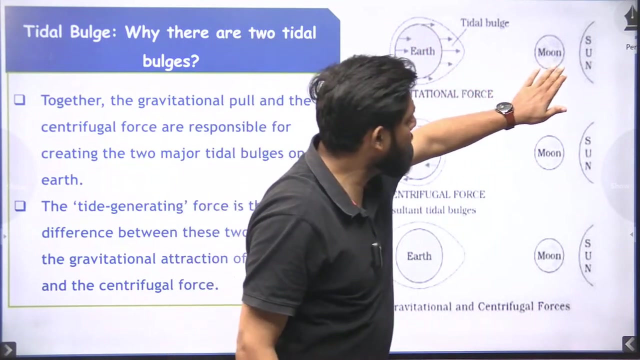 I will bring the spring tide here To explain the concept. I will go to the image and there I will explain things. Let's talk about it first. See what happens here. Here is the earth, Here is the moon, Here is the sun. 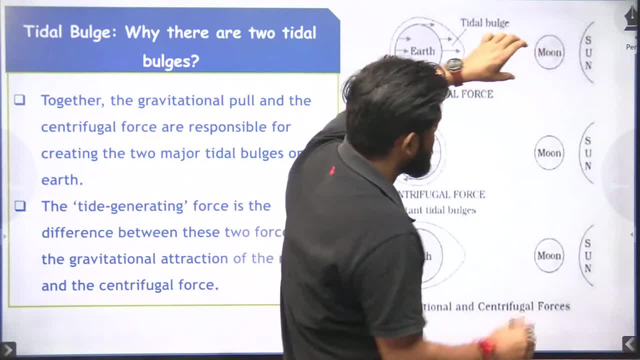 The gravitational force of the sun and the gravitational force of the moon. The gravitational force of both will be added. And where will this gravitational force be applied? It will be applied on this part of the earth, Because of which water will also be applied. 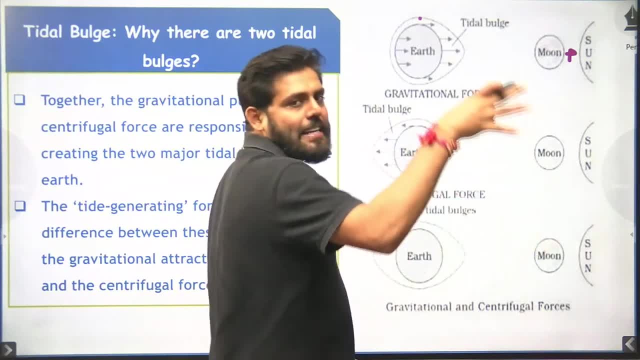 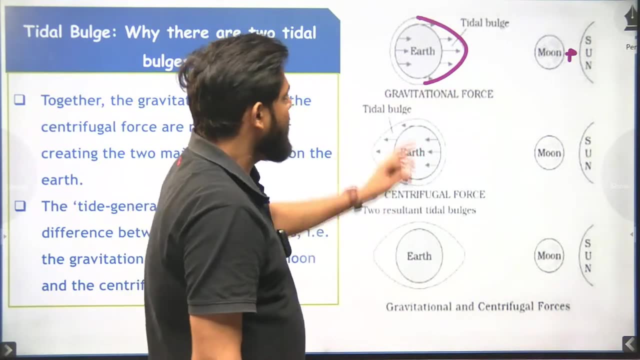 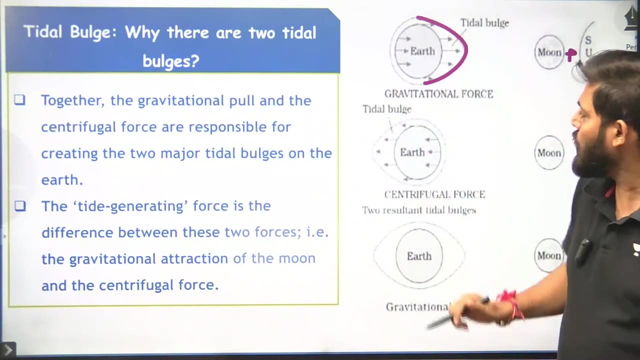 Because of which water will rise, So a tidal bulge will be generated here, Due to which? Due to the gravitational force. And remember when the earth, the moon and the sun are in one line, try to understand. When the earth, the moon and the sun are in one line, then that position is called SISGI. 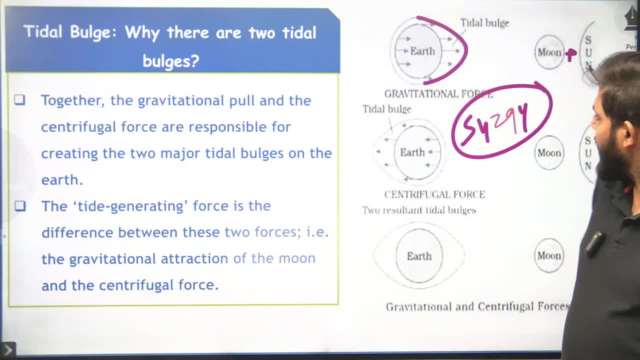 That position is called SISGI. Remember What is that position called? It is called SISGI, SISGI. Okay, When the earth, the moon and the sun are in one straight line, then that position is called SISGI. 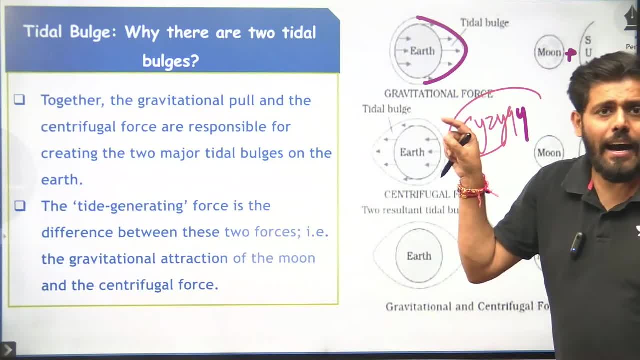 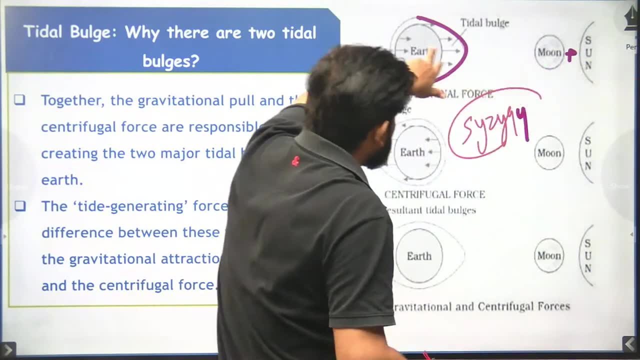 There is a question made in the previous year of UPSC. When the earth, the moon and the sun have a 90 degree angle between them, then that position is called SISGI. No, When the earth, the moon and the sun are in one straight line, then that position is called SISGI. 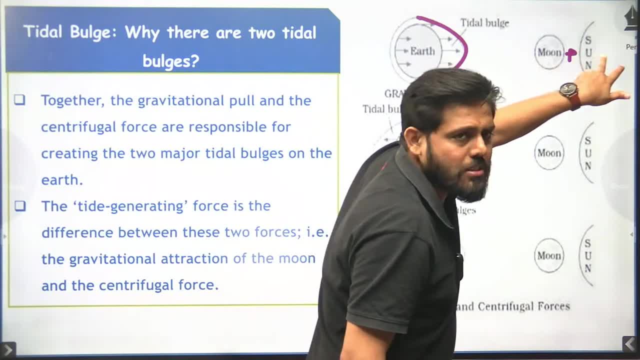 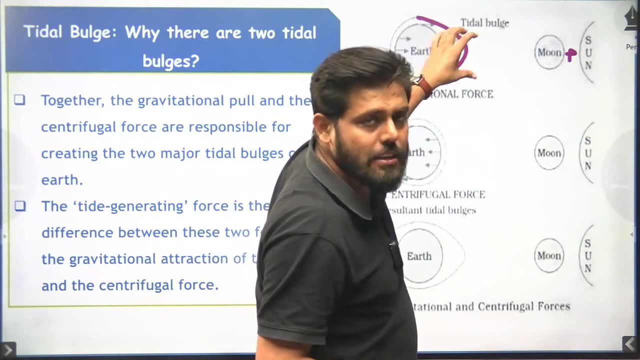 Is it clear. And when these three are in one straight line, then the gravitational force of the moon and the sun will be strong. Who will have more? It will be the moon, Because the moon is near. What will it do? It will rise the water from here. 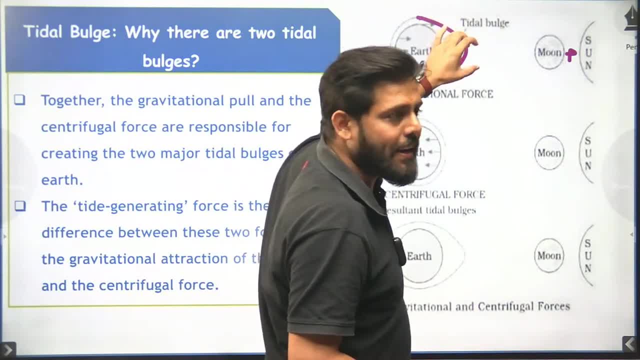 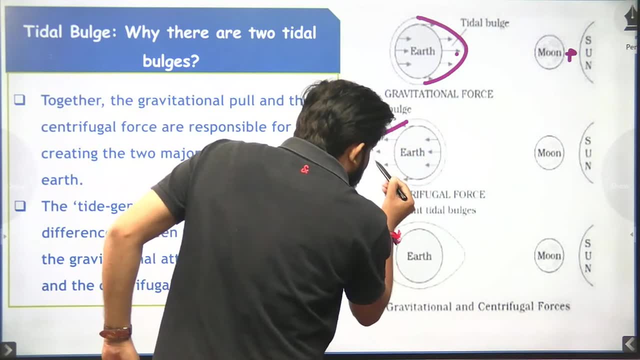 It will rise the water, A tidal pulse will come, because of which the high tide will be in this area, And the reason for high tide is due to the gravitational force. Now what will happen? A tidal pulse will also be made towards the same place. 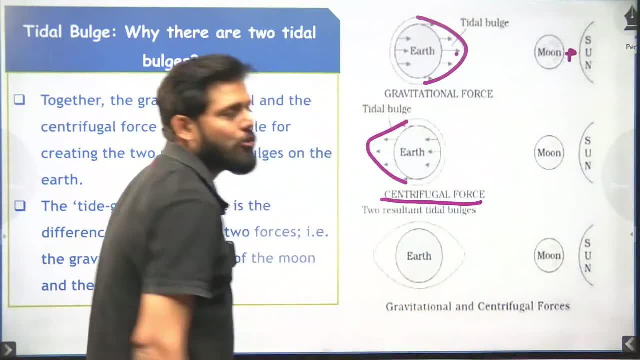 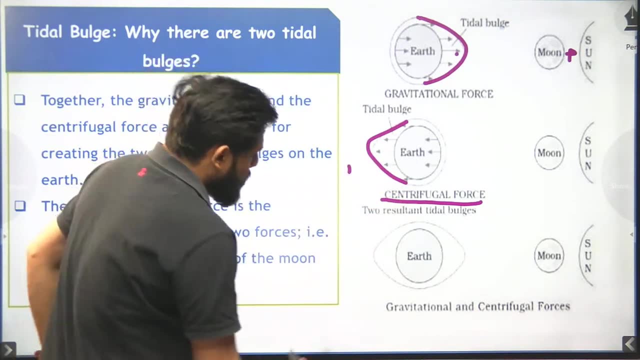 And the tidal pulse will be made here due to the centrifugal force, Equivalent opposite force- which is there to counterbalance towards the back. High tide is also there here, So there is high tide in this area. There is high tide in this area. 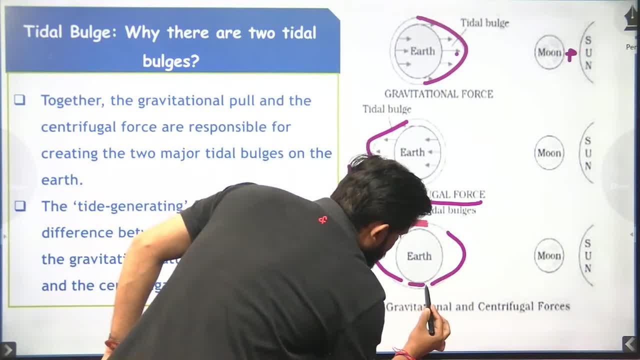 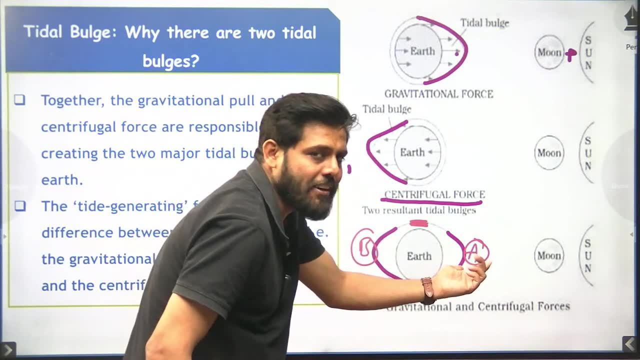 But here the upper portion. Here, in both the areas, low tide will come. So A area has high tide and B area has high tide. This high tide is due to gravitational pull. This high tide is due to centrifugal force. 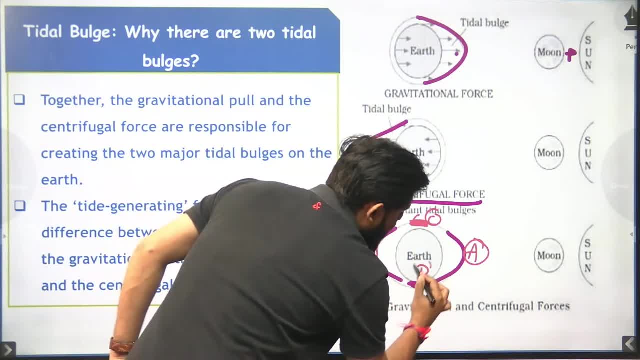 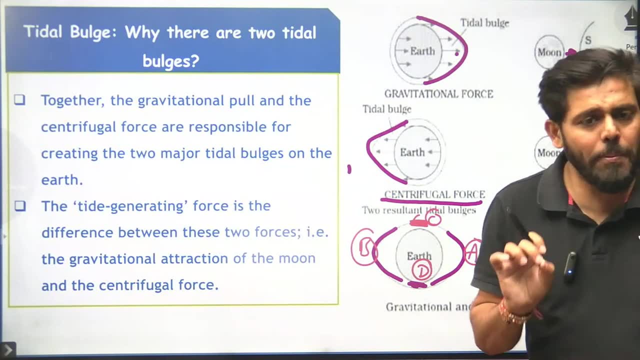 And here this is C and this is D. Here low tide will come in both the places. Is it clear? Does anyone have any problem? Okay, In any way. Is it clear? If anyone asks you Now, if anyone asks you when high tide and low tide are formed, 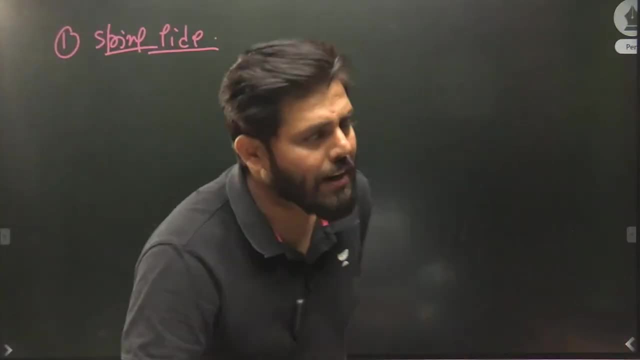 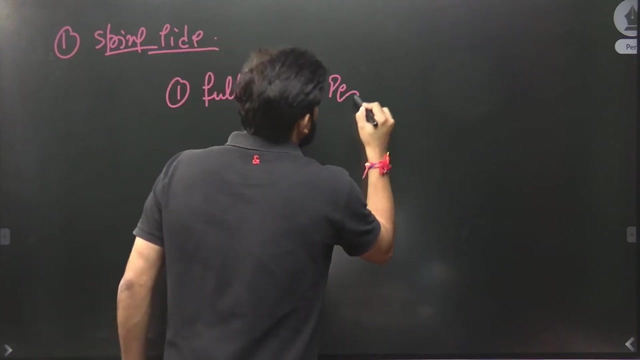 In what condition will it be formed? So you have to tell. It will be formed in two conditions. One will be formed at the time of full moon period. At the time of full moon period, What is it called? Full moon is called Amavasya. 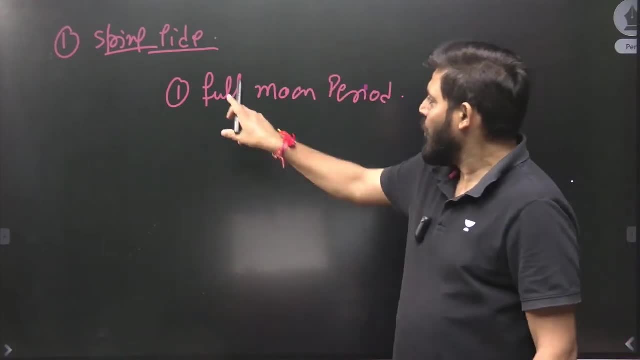 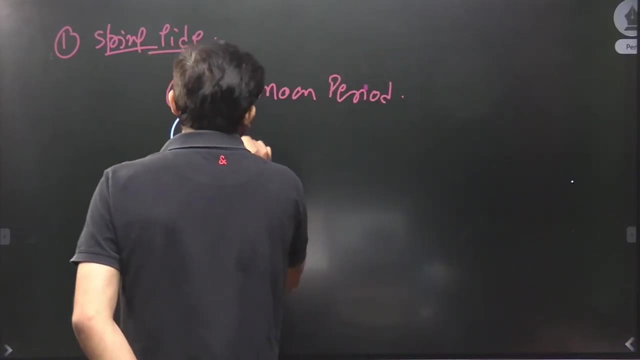 What is it called? Or it is called Purnima, Full moon period. At that time, your high tide will come. Is it clear? And what will come next When there is a new moon period? At the time of full moon and new moon period, your high tide will come. 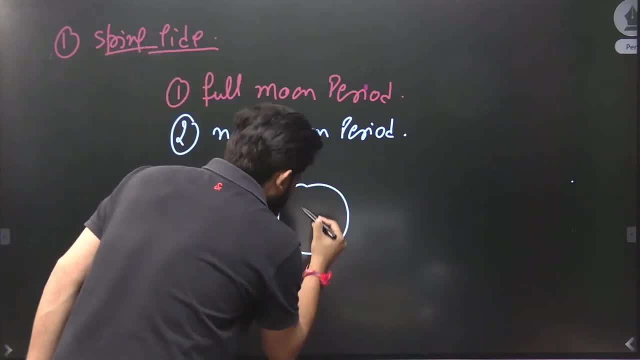 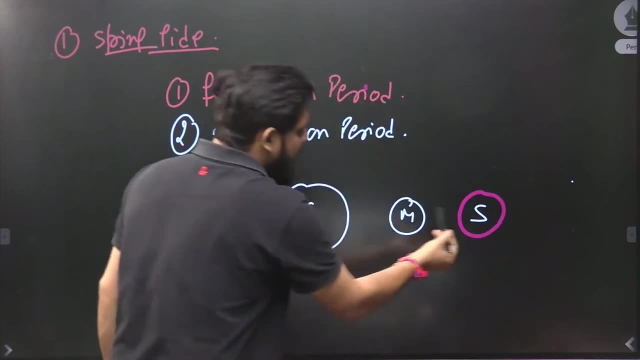 When will it be formed? I will tell you this Here. Here is the earth. Okay, If our moon is here after revolving- And here is the sun, Here is the sun, Here is the moon- If this is the condition, then also high tide will come. 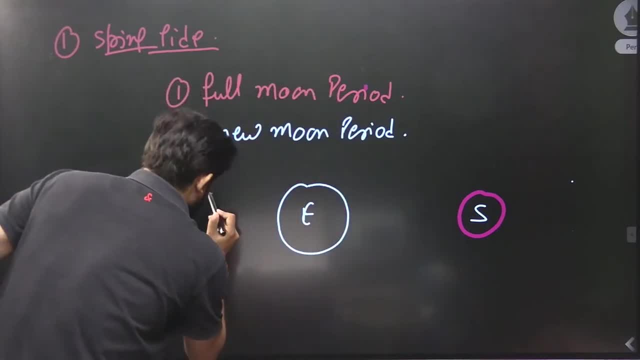 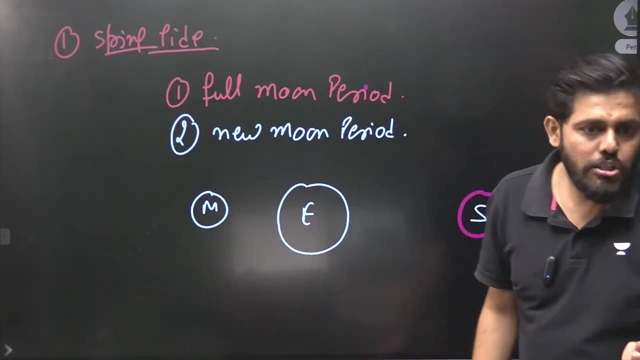 And when the moon comes here after revolving Here, Then also these three are in one line, Then also your high tide will come. Try to understand. If anyone has any problem, tell me Here. also high tide will come When all three are in straight line. 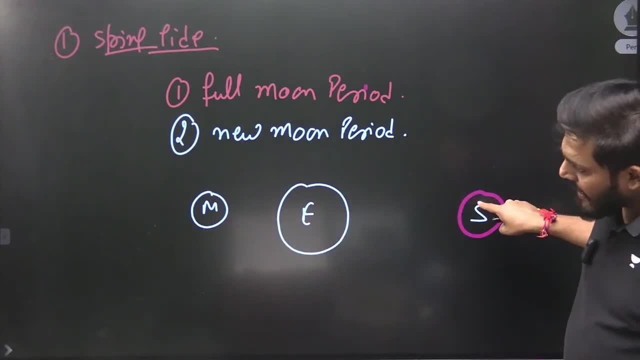 If it is possible that there is earth between sun and moon, then also high tide will come When there is earth between sun and moon. And if someone asks you when there is earth between sun and moon, When there is earth between sun and moon, 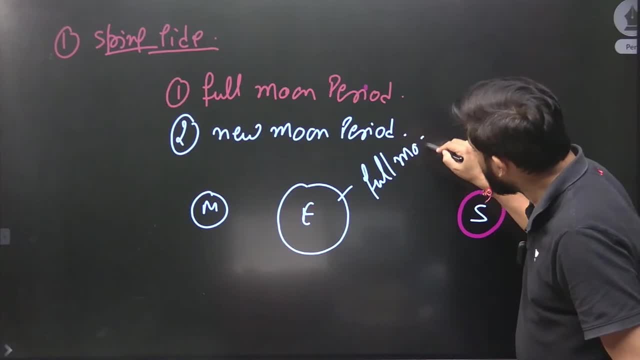 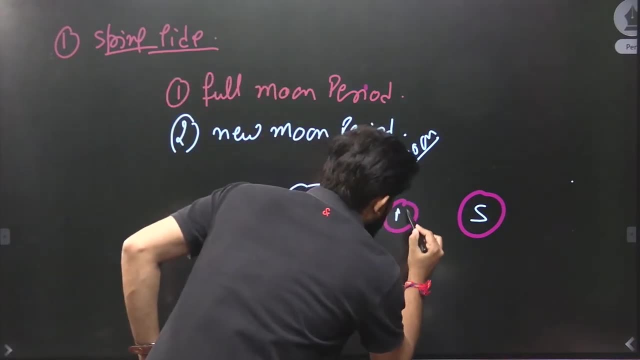 This condition is called full moon. What is it called Full moon? And when this moon comes in between from here, That means when there is moon between sun and earth. So what is this called? This is called your new moon. What is this called? 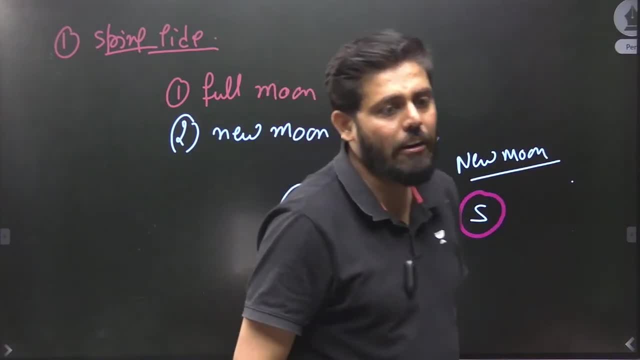 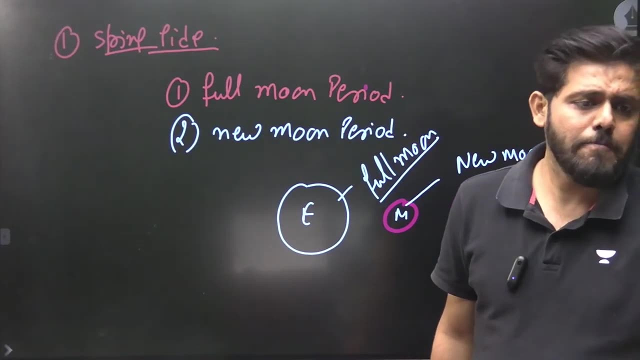 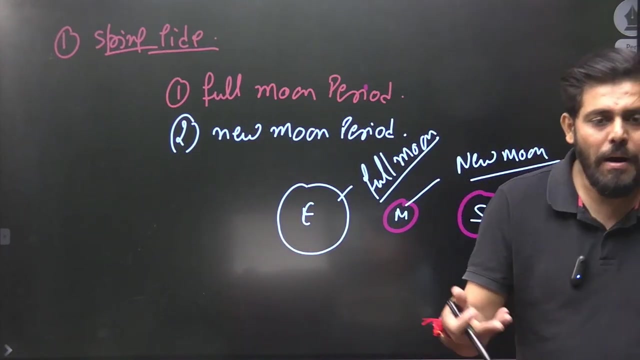 New moon. So you have to remember these things too: When full moon will come and when the condition of new moon will come. Did you understand? Does anyone have any problem? Tell me quickly. New moon is amavasya. Amavasya means black night. 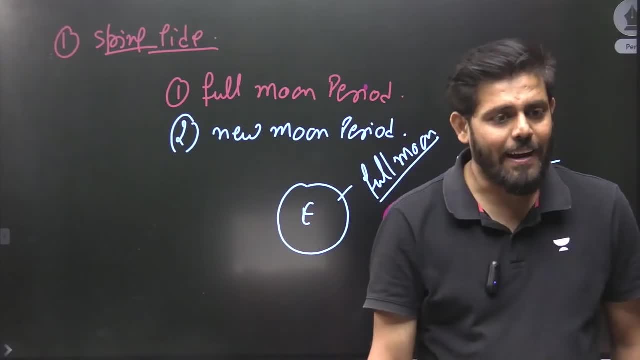 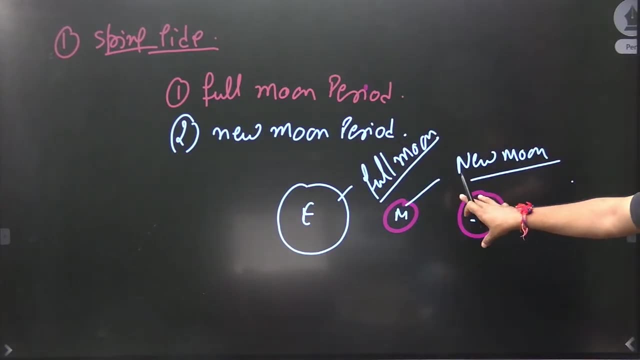 What is the meaning of new moon Amavasya? Amavasya means black night, Okay, Okay. And what is the meaning of full moon? If someone asks you New moon? What is the meaning of new moon Amavasya? 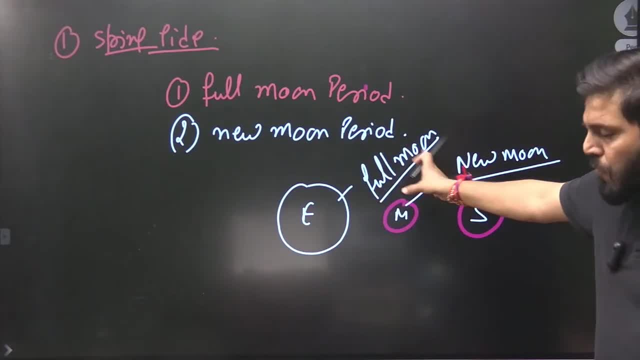 Amavasya means black night. And what is the meaning of full moon? What is the meaning of full moon? Full moon means your full moon cancer. Okay, It means when there is more. Okay, Okay, This point is clear till here. 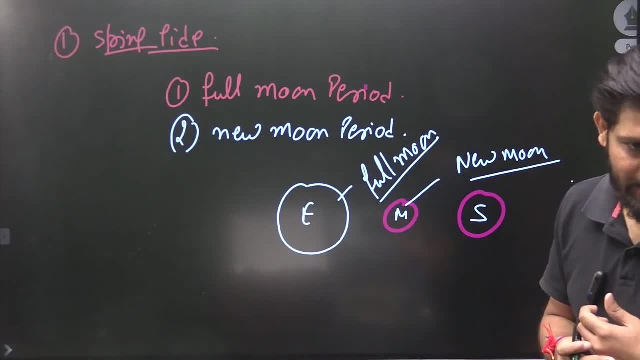 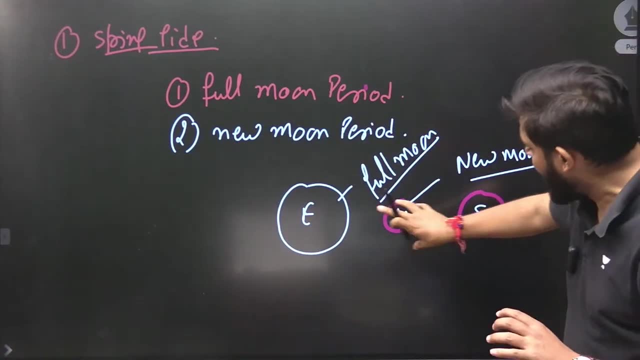 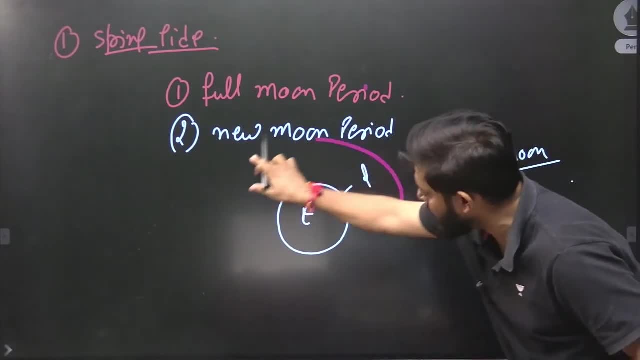 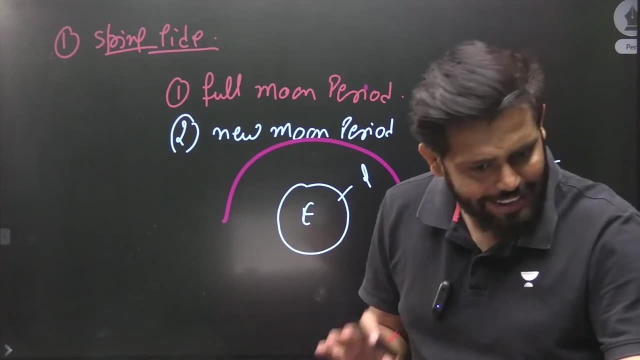 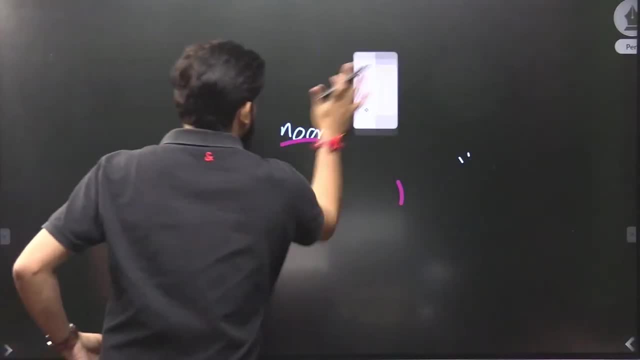 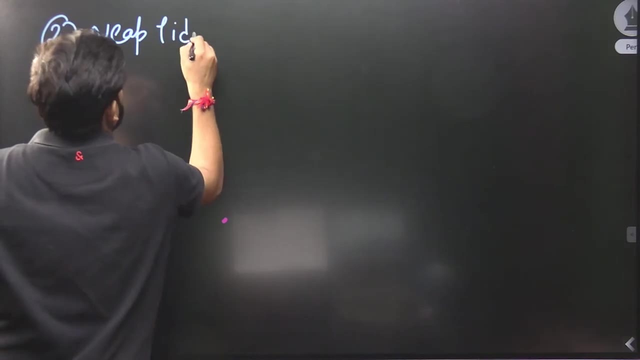 Sorry, neep tide's condition. This is your spring tide. Now I will talk. second condition: what is neep tide for you? Nip tide, What is neep tide After that? I will teach another concept, I hope: tidal bow or theirs. 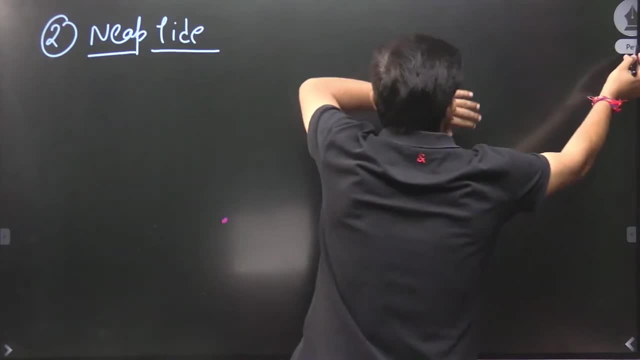 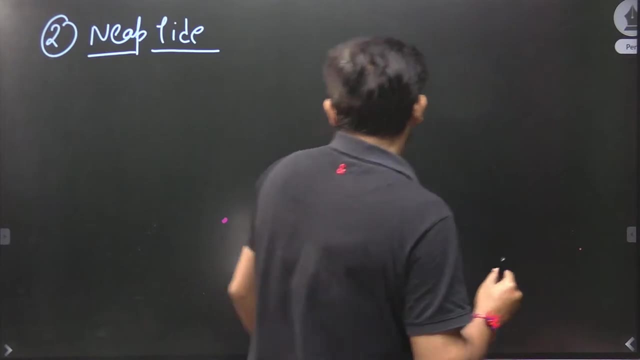 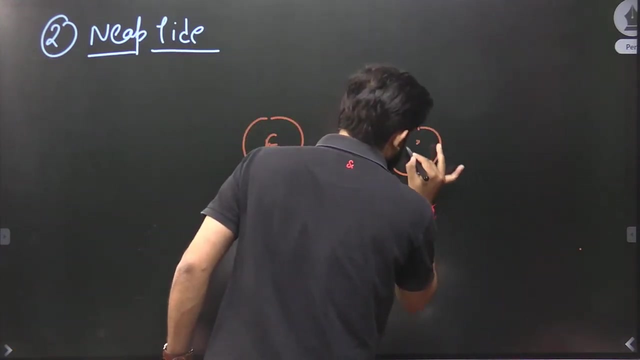 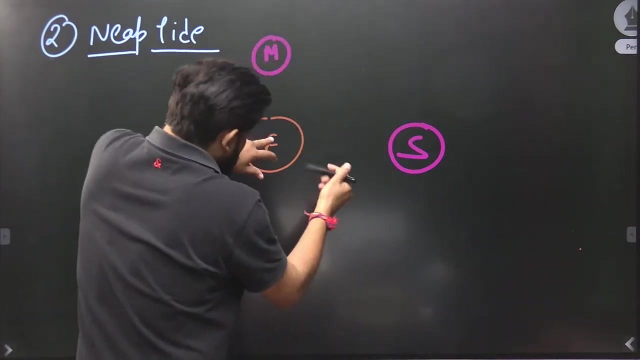 The question be asked by UPSC, by tidal core. Now let's talk about neap-tide. try to understand neap-tide more. just give me one minute. here is our earth, here is our sun and here is our moon. so when this moon is here, let's. 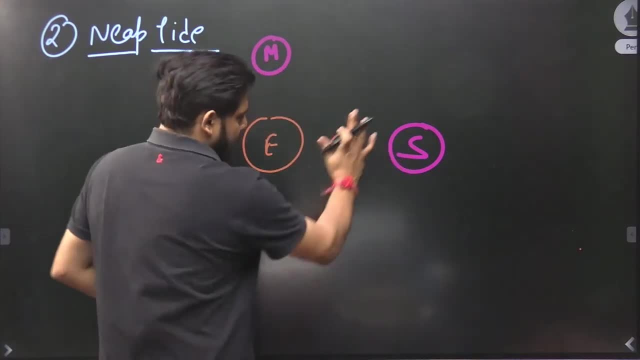 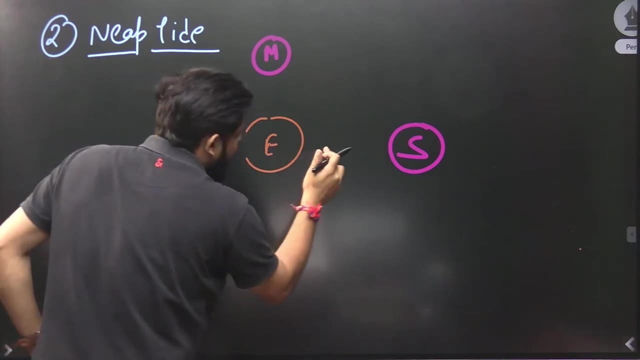 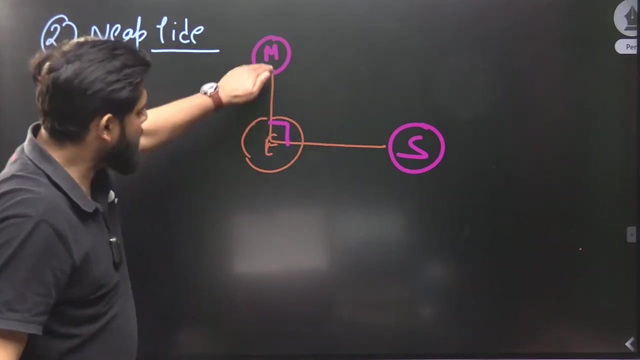 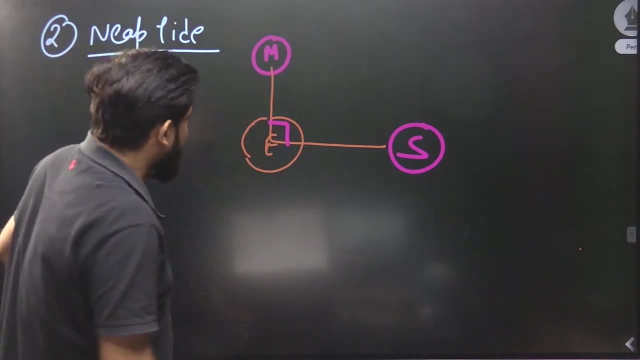 assume moon, so here will come our high tide. but moon will come here by revolving then this 90 degrees angle between sun and moon. sun and moon will become perpendicular to each other. from here gravitational force is given. Here gravitational force will be of moon. suppose moon's gravitational force is here. 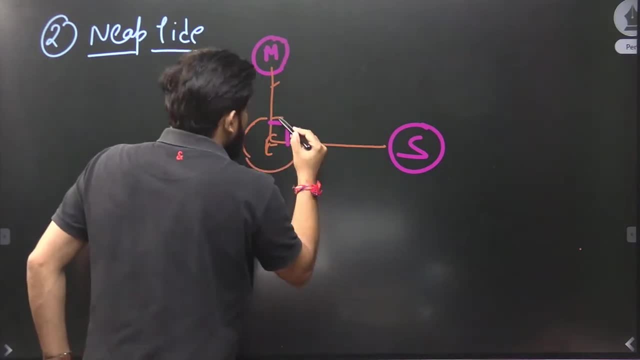 what was I saying earlier. if gravitational force is 10 units, so 10 units will come. if it is 10 units, then 10 units of gravity force- if it is 10 units, it will also come. so this is also very important. 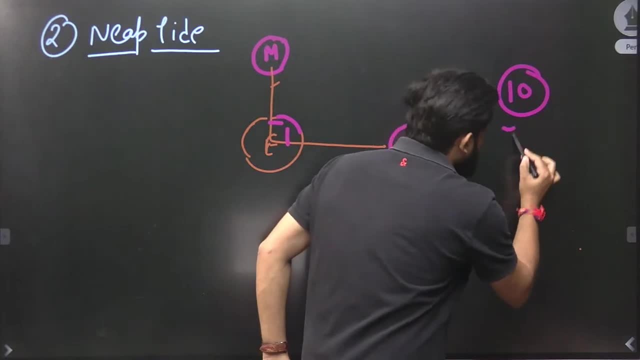 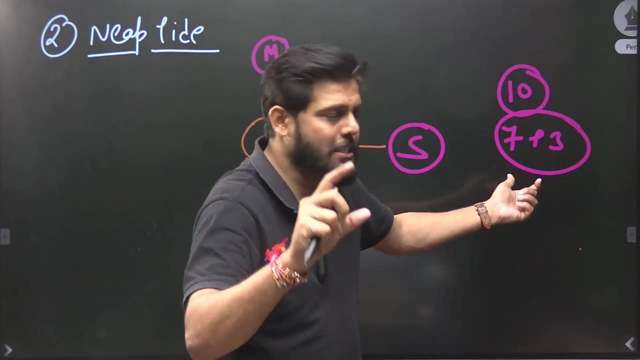 If the gravitational force is high, then what? whose gravitational force is 1 unit? Your 7 unit is of Moon and 3 unit is of Sun, Because whose gravitational pull is stronger? Moon's Moon is near, So here, if my 7 unit 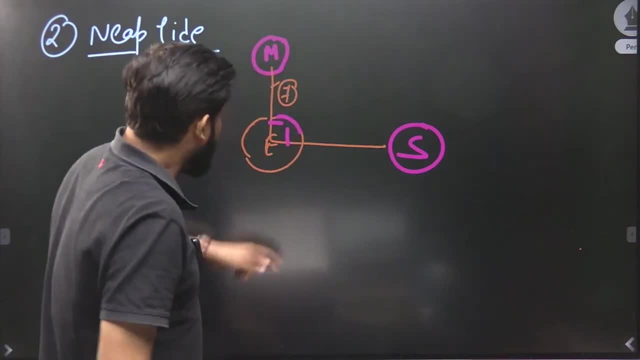 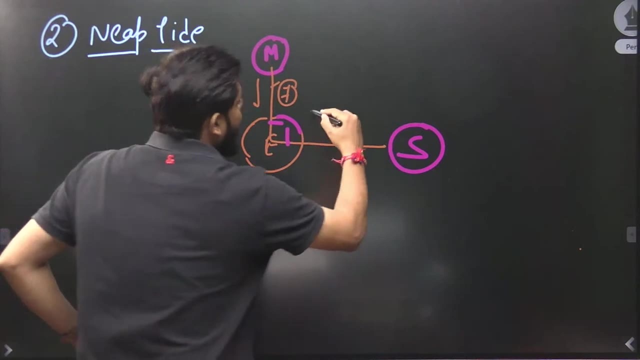 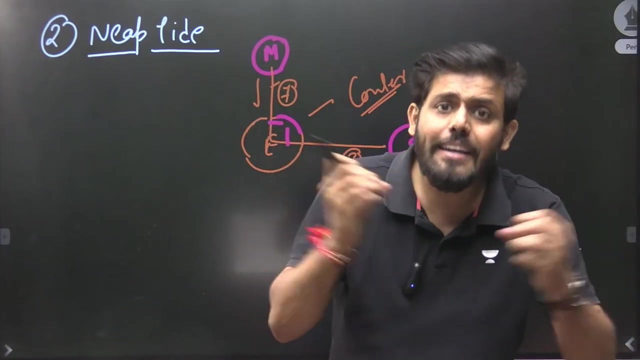 is of Moon's gravitational pull from here, from this side, then my 3 unit is also of Sun's, But here both these gravitational pulls are counter-balancing. That means they are countering each other. They are trying to cut each other, If I tell you, 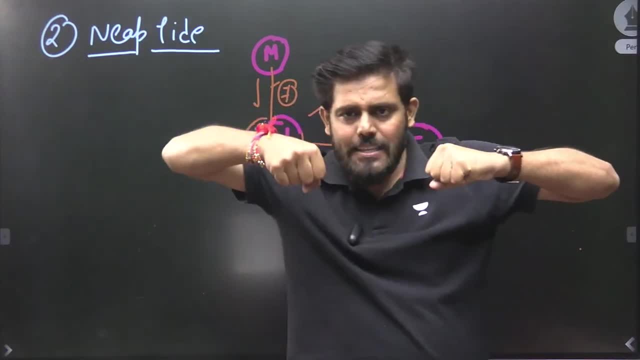 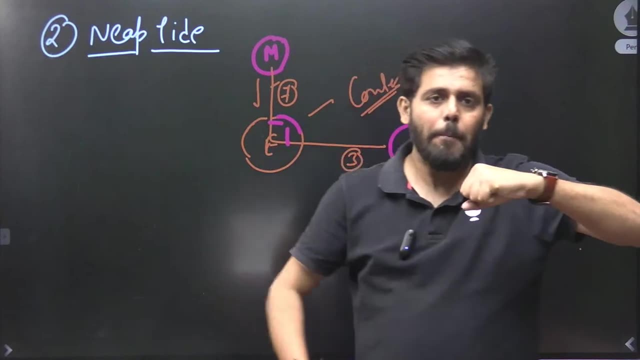 that there is an area here, pull it. So you will pull from here. If I tell you that another person comes behind you, they also pull it. So both forces are added on. But if I tell you that you pull from above and pull from one side, So someone is pulling from here and someone is pulling from here. 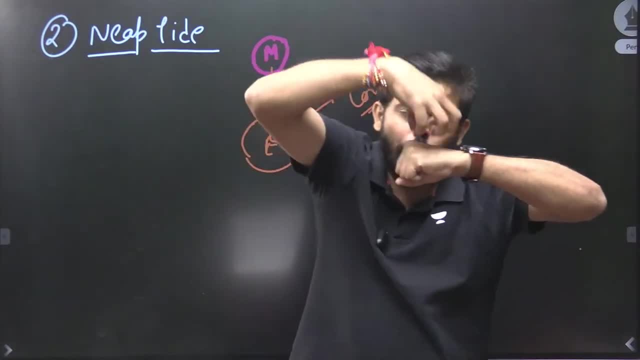 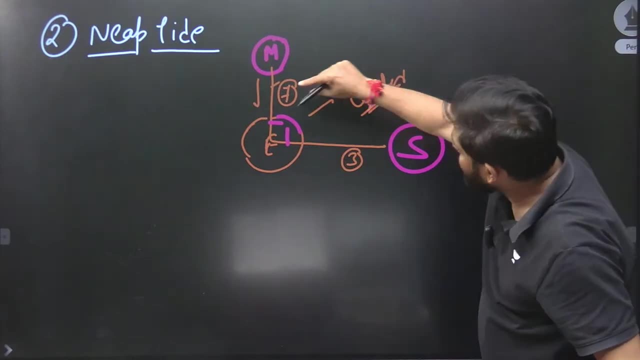 So the back will be reduced, Because the one who is pulling from here, What will he do to the upper force? Neglect decrease. Same concept is happening here too. So when the balance force of Moon is applied from here, and from here it is of Sun, 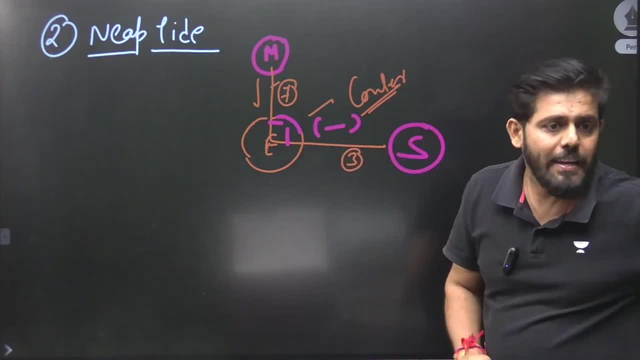 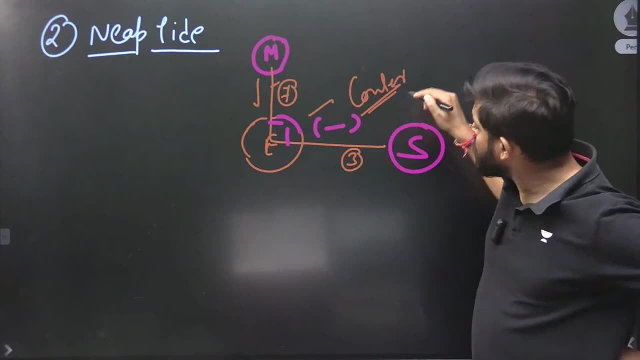 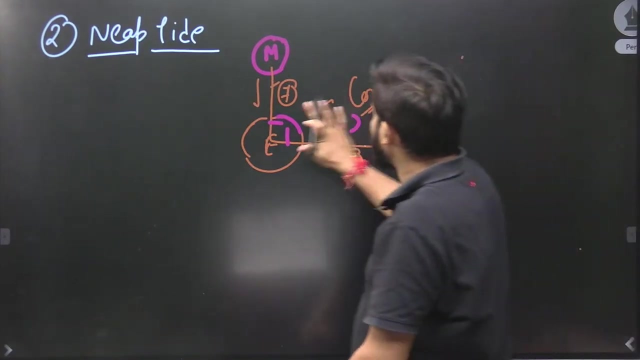 Then these negative things are coming here. Try to understand: When Sun and Moon come at 90 degree, Then the gravitational force of Moon, This gravitational force of Sun, is canceling it And, due to canceling, Moon's gravitational force is getting weak. And what will be the condition? due to being weak? 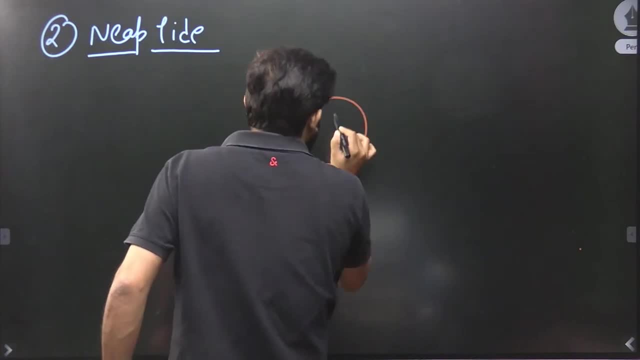 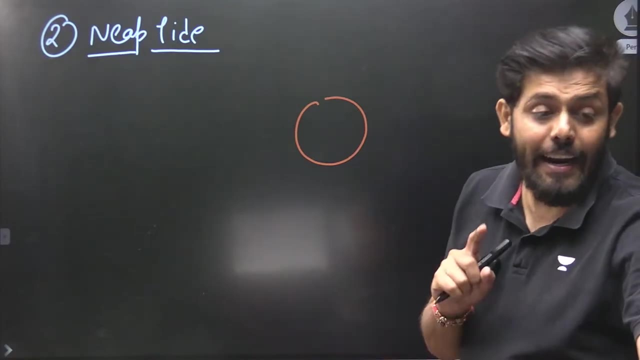 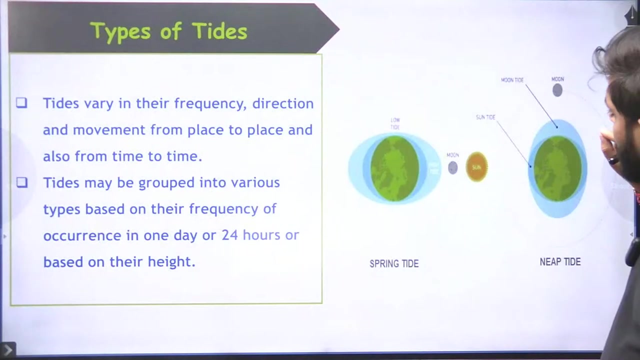 Due to being weak When Moon and Sun. So here the neap tide will come And you can say low tide. Do you understand What will come? Neap tide and low tide, Remember this. If I try to explain you, I can have the image. Okay, Is it clear? 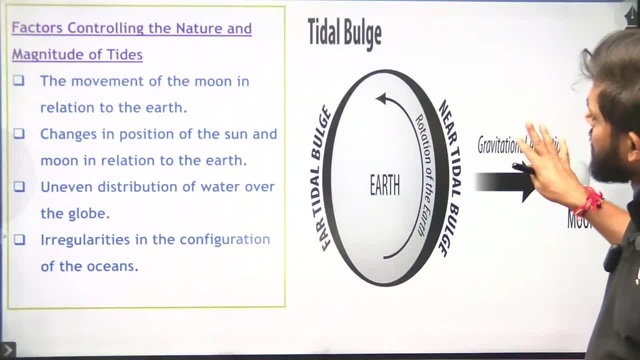 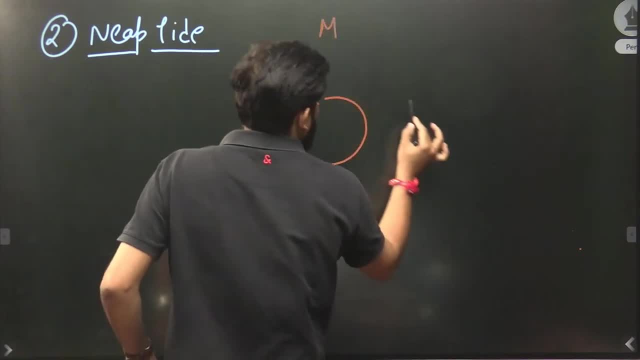 So here neap tide will come. You have to understand. So in this area where high tide was happening, Now what will happen? there, In the area where high tide was happening And here is the Sun? So if we do counter balance, Then in this area low tide will come. 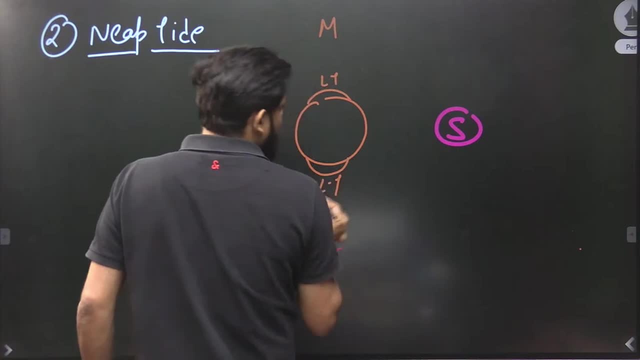 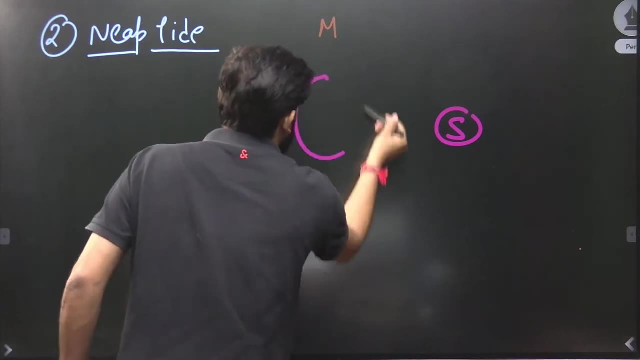 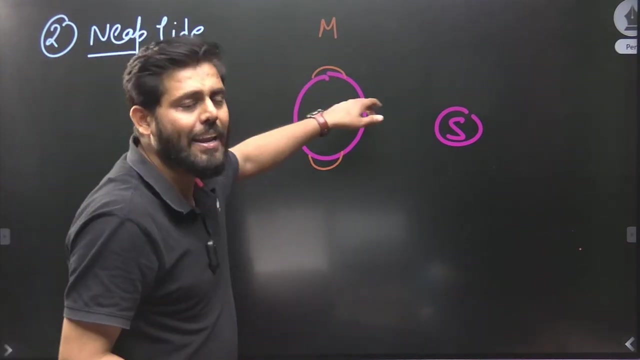 Here also low tide will come. If we do counter balance, Then here also low tide will come. So here is low tide, So in this area high tide will come. So generally you can say That in this part, In this part high tide will come. This is the most important point. 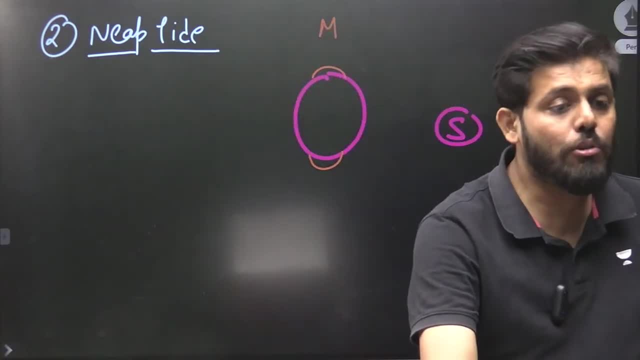 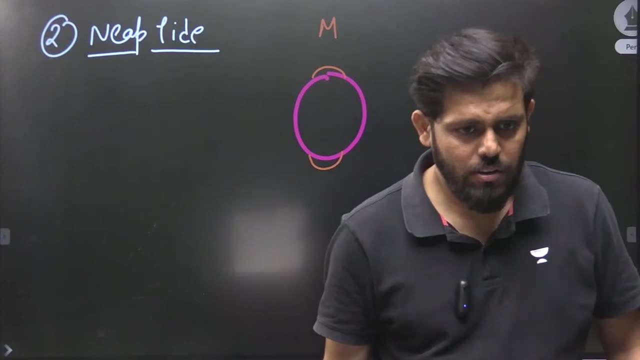 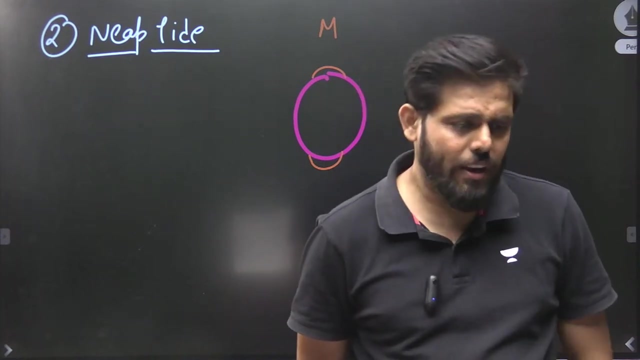 Is it clear Because of which high tide is coming? It is getting counter balanced. Do you understand? They are cancelling each other. Okay, Yes, we will say Shizgi If it is coming in one line, So where will neap tide come? Always remember. 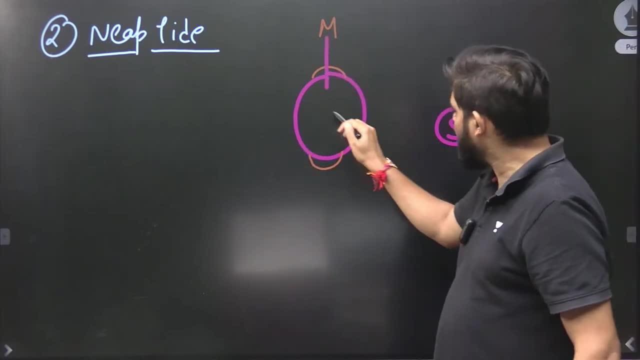 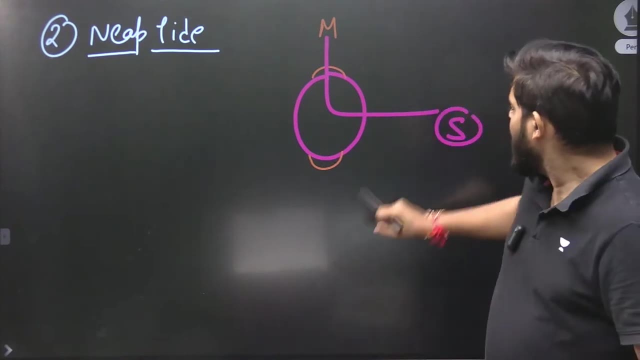 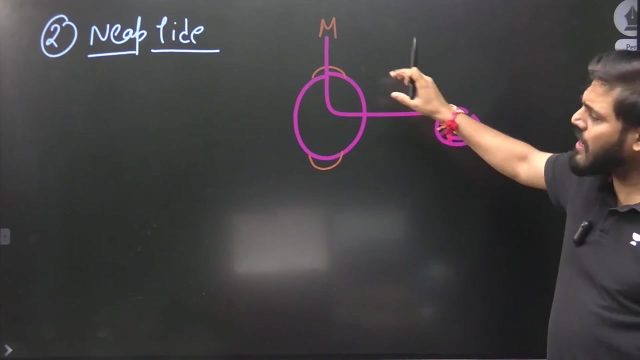 When the force of Sun and Moon will be cancelled, When they will be perpendicular to each other- And always remember That the gravitational force of Moon Will be strong And the force of Sun Will dim- the gravitational force of Moon Will try to reduce it, Because of which neap tide will come. 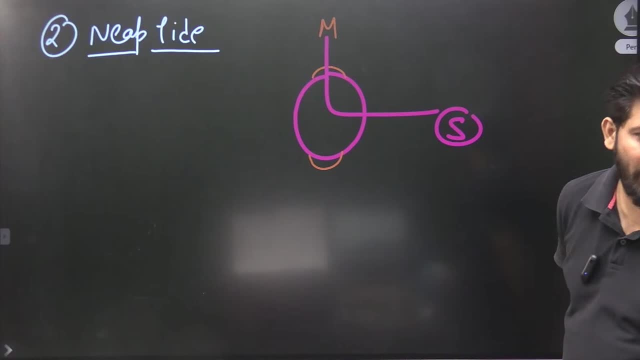 Do you understand? Is it clear? Does anyone have any problem? Okay, So you understood the concept of neap tide. So if we ask you, When will neap tide come? So tell me one thing: Here is the Sun. Try to understand. Here is the Moon. 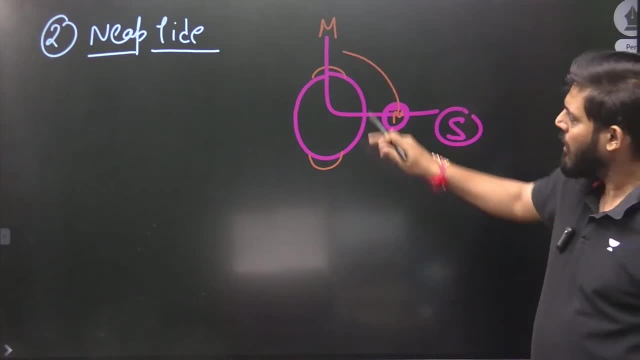 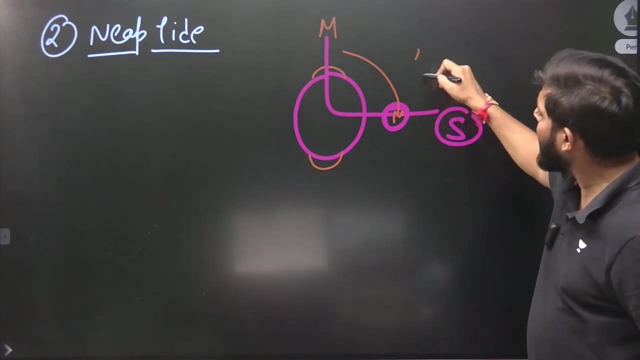 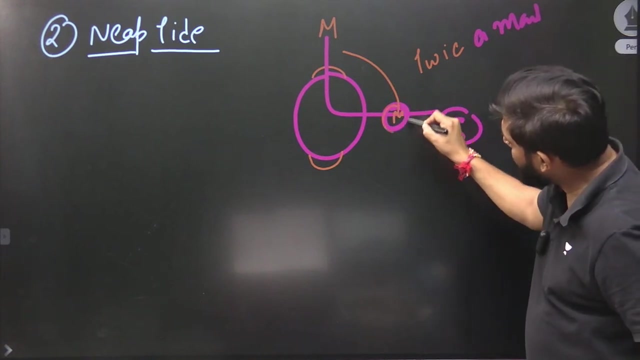 The Moon will go in this position: First quarter, Second quarter. It will change the position like this. So, basically, How much will your neap tide come Twice a month? Twice a month. It will come twice a month. When will it come Once the Moon is here? 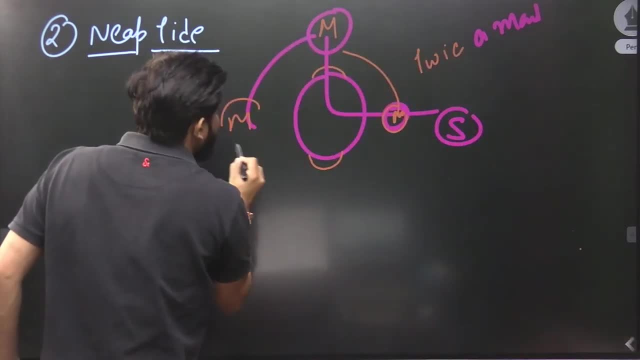 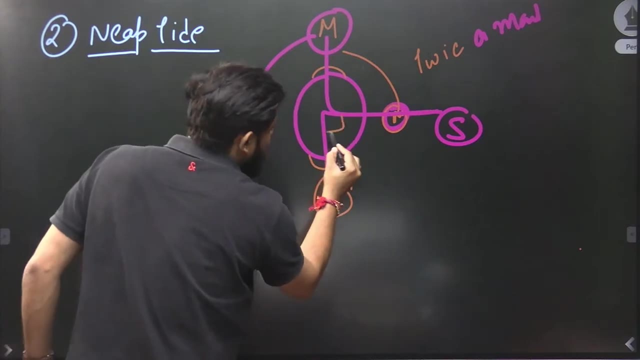 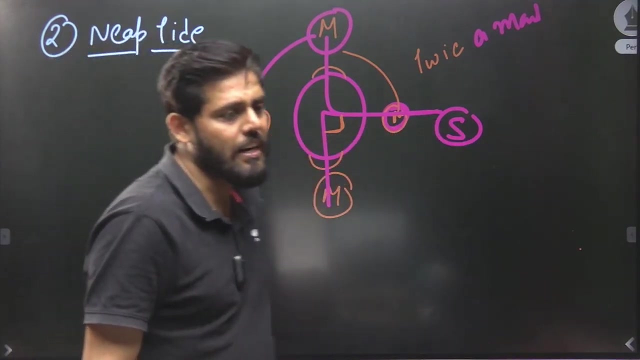 Then it will not come. Once the Moon comes here, Then your neap tide will come. Then, when the Moon comes here, Because there is still a 90 degree angle Between the Moon and the Sun, So its gravitational pull Will cancel its gravitational pull. Remember this thing. So how much neap tide will come? 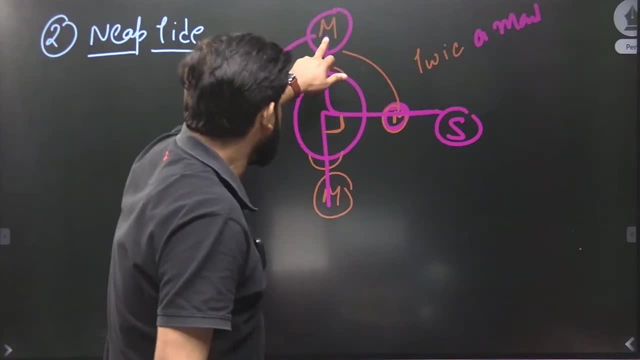 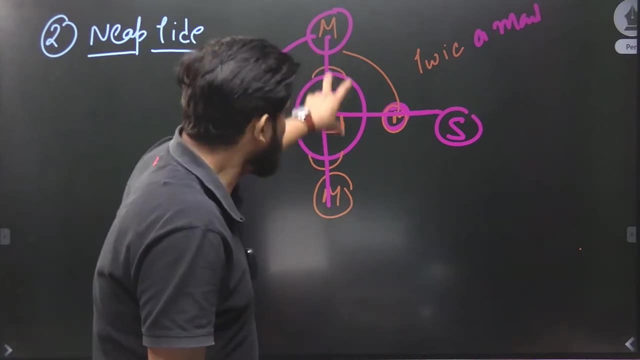 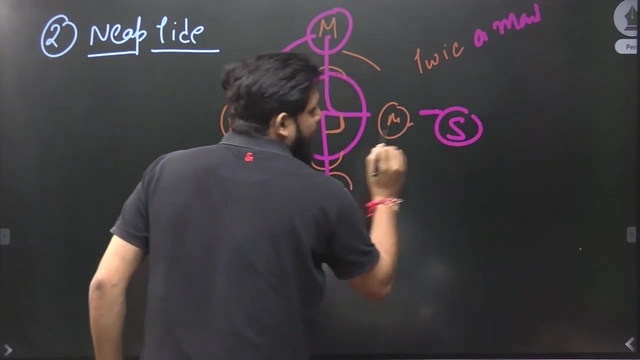 Twice a month, And in what condition will it come twice a month? So you can see In this condition When the Moon will be here And when it will come here. So when will neap tide come? Twice a month In one line, Then spring tide will come. 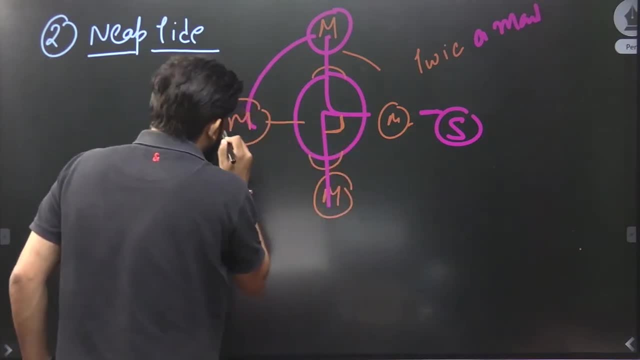 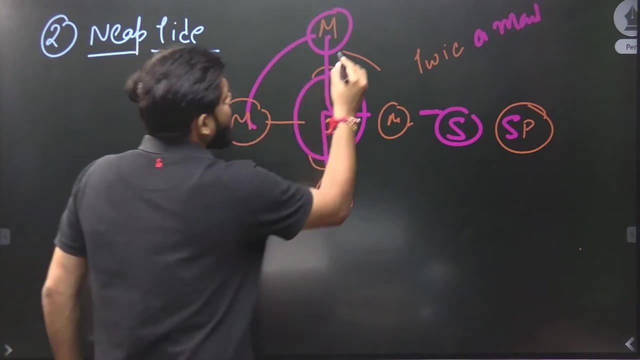 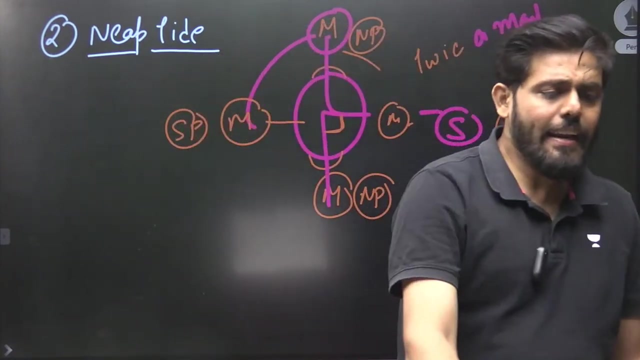 Which is called high tide, And when the position of the Moon And the position of the Sun Will be same here, Then also spring tide will come. So these two conditions are of spring tide. SP is spring tide And this condition is of neap tide. That means NP. 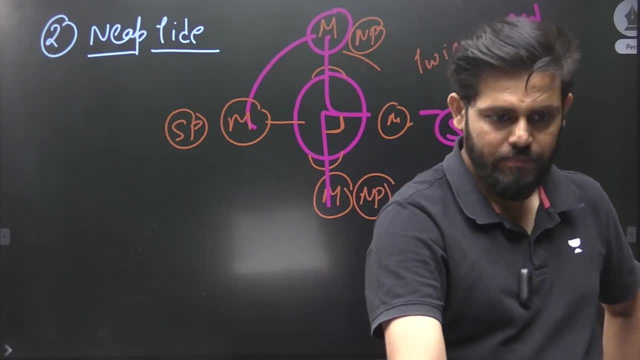 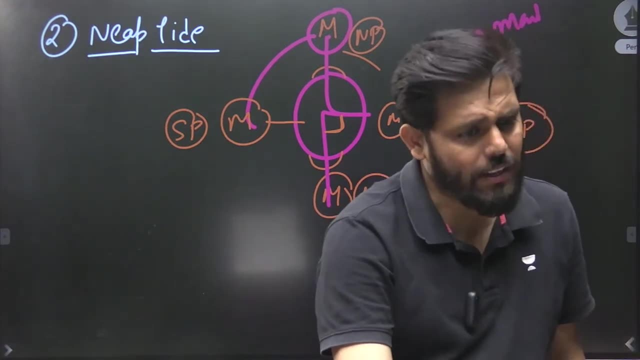 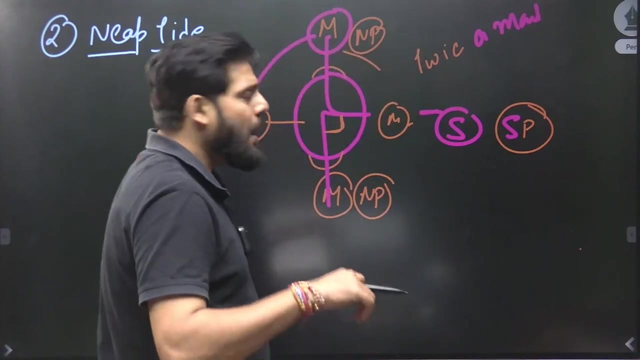 This thing is of neap tide Clear. If anyone has any problem, Tell me quickly Now. I will try to explain one thing to you Very nicely: Your high tide. When will be the highest high tide? When will be your highest high tide? Tell me one thing. 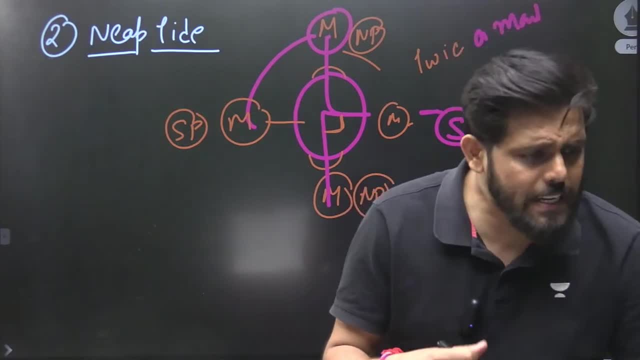 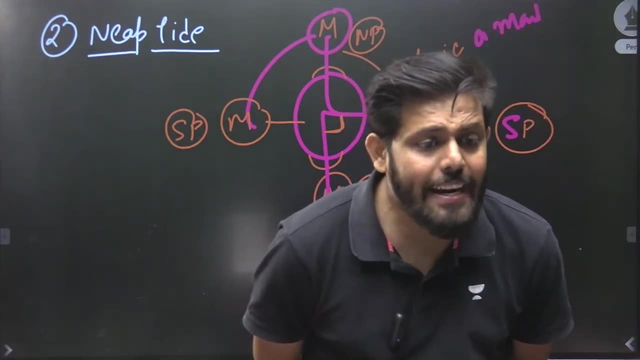 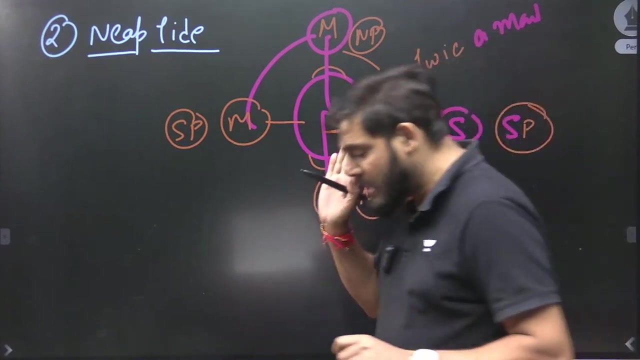 Comment it quickly: When will you get to see The highest high tide? When the height of Tide is maximum? Very good question of Anand, Sir, when will be the maximum high tide? If you Will understand, I have taught you about Parsi and Aposi. 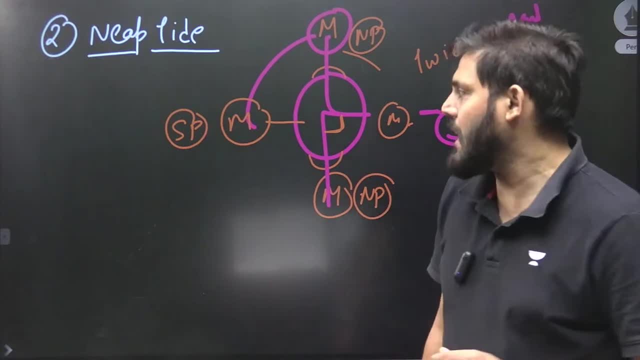 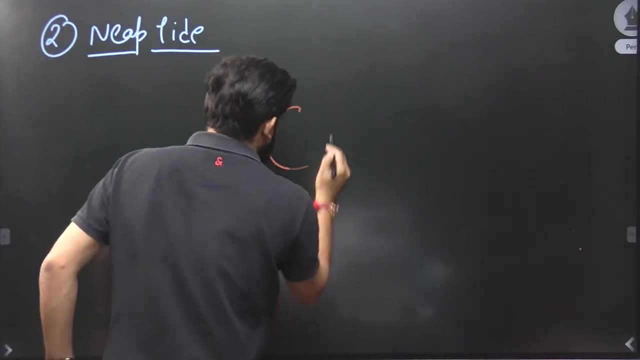 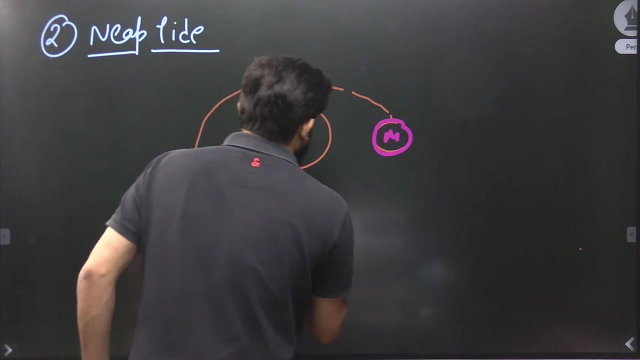 How many students have you studied Parsi and Aposi? What is Parsi and Aposi? I have taught you very well That this is our Earth And around this Earth, Our Moon is revolving. What is the Moon doing? It is revolving in the elliptical path. 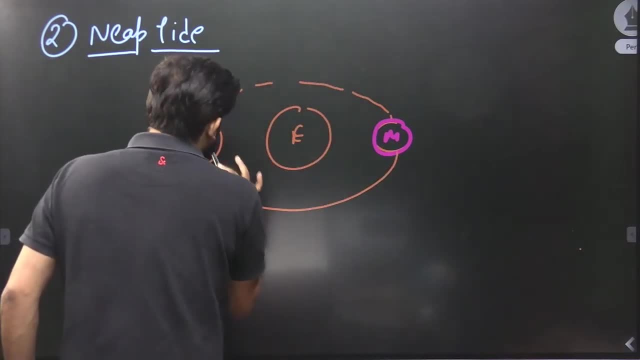 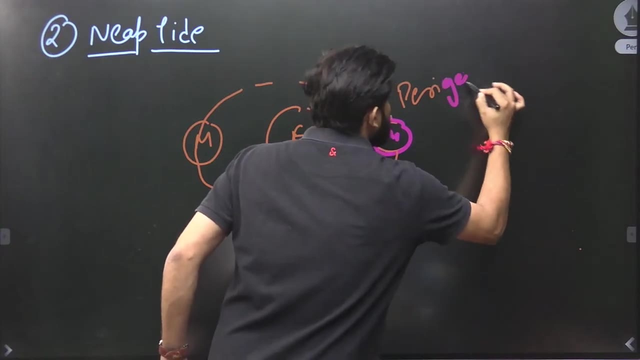 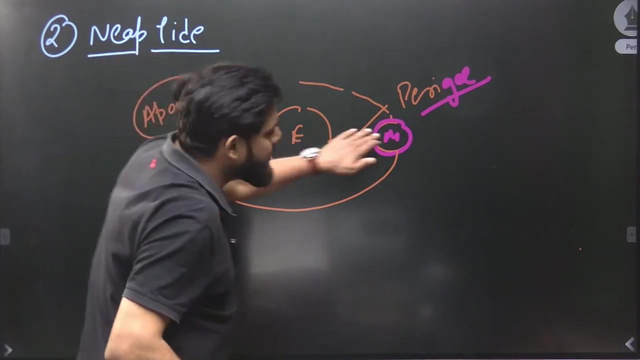 One condition comes When the Moon revolves. When the Moon comes closest to the Sun, That condition is called Parsi. When the Moon is farthest from the Earth, That condition is called Aposi. Remember At the time of Parsi, It will pass the Earth. That means 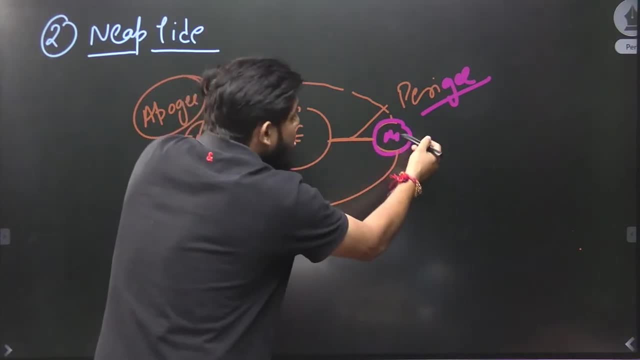 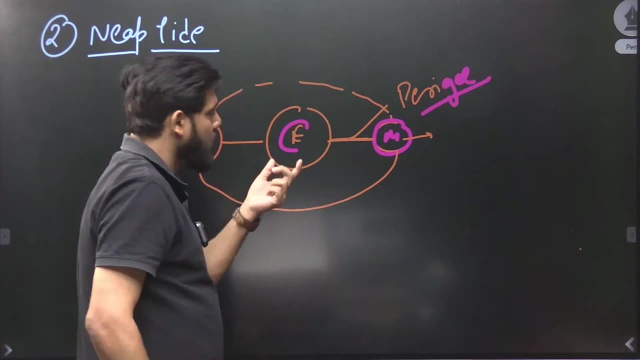 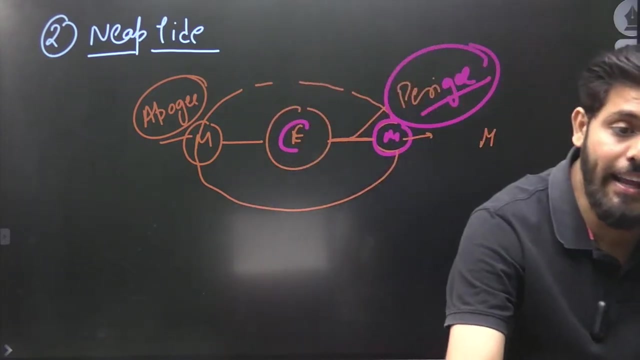 The distance between the Earth and the Moon is minimum, The least distance between the Earth and the Moon. That means The gravitational pull is strongest Where, In this condition, At the time of Parsi, Because of the maximum gravitational pull, The height of the tide Will be very high. 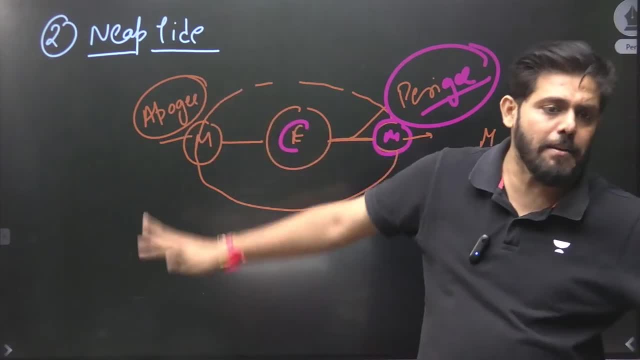 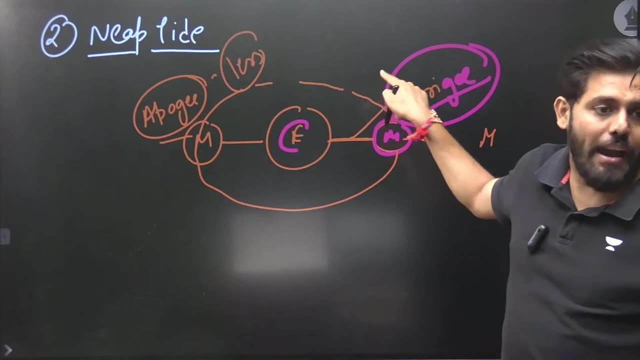 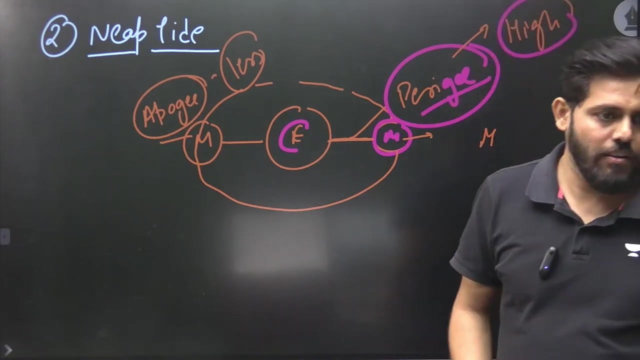 So always remember At the time of Aposi. It is farthest from the Earth, So the average height Will be less And because the average height is closest, Usually The height of the high tides Will be very high. Okay, Clear. So what does it mean? 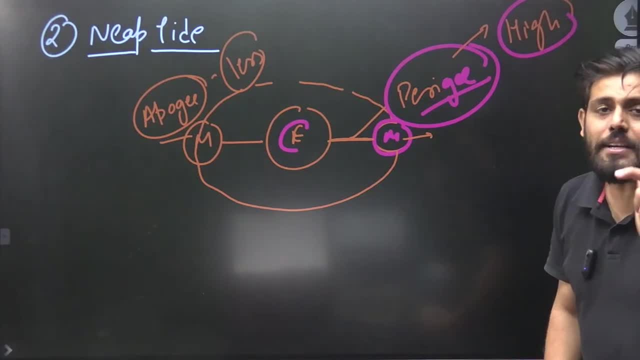 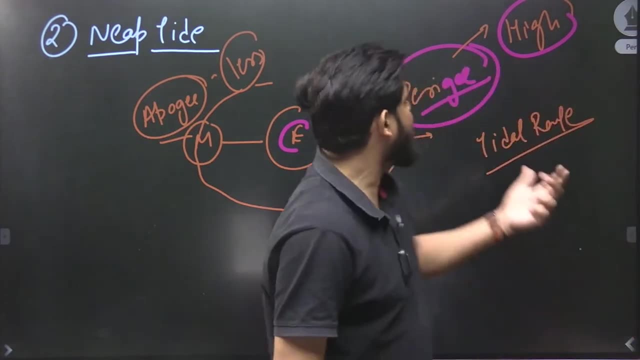 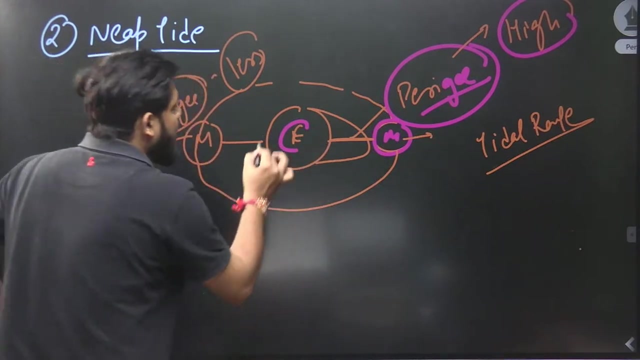 When the Parsi condition is. If you are asked That the tidal range, If you are asked That the tidal range, When will its value be highest, Then you have to tell At the time of Parsi, Because at the time of Parsi The high tide will be more high. 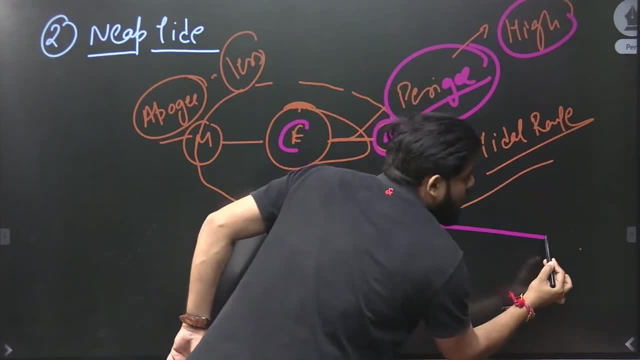 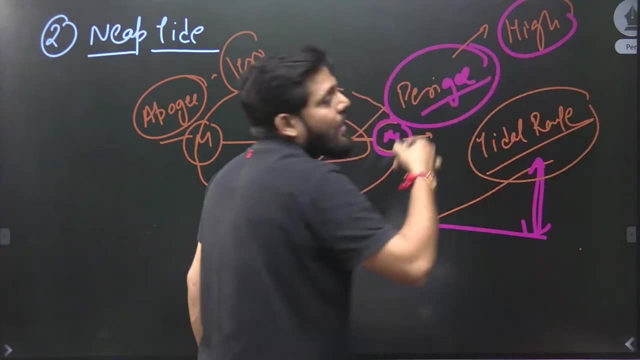 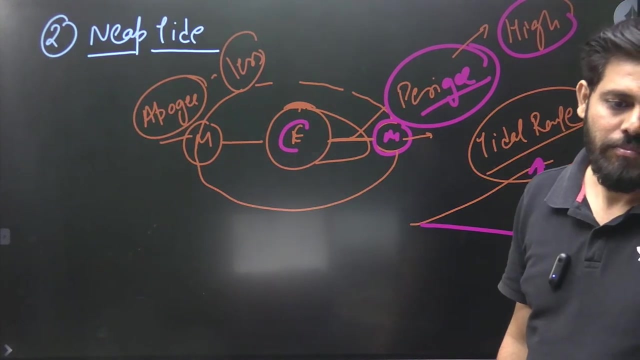 And when the high tide will be more high, Then the low tide will be even lower. So that means The height of the high tide and the low tide Is called the tidal range, And here the tidal range Will be strong. Does anyone have any problem In any way? 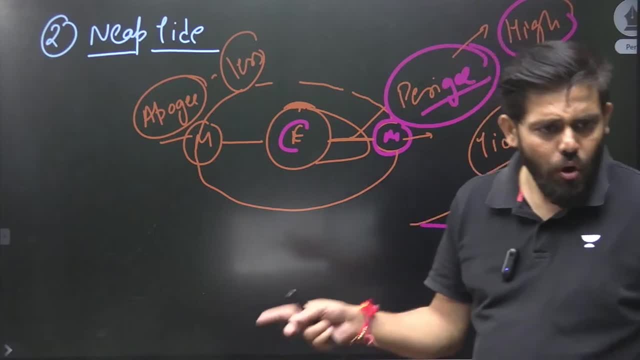 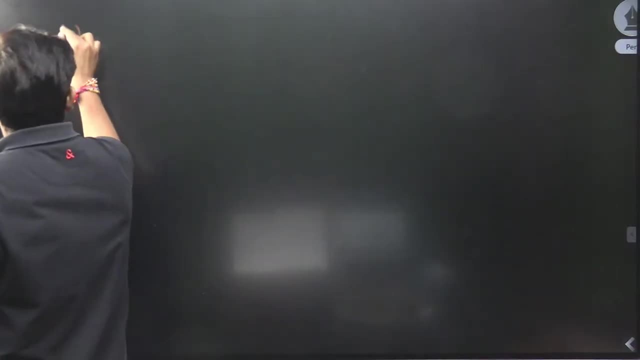 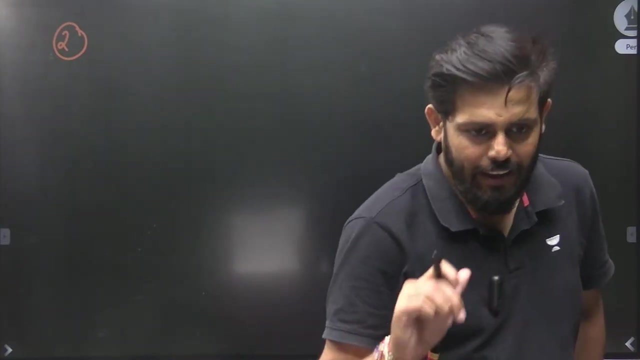 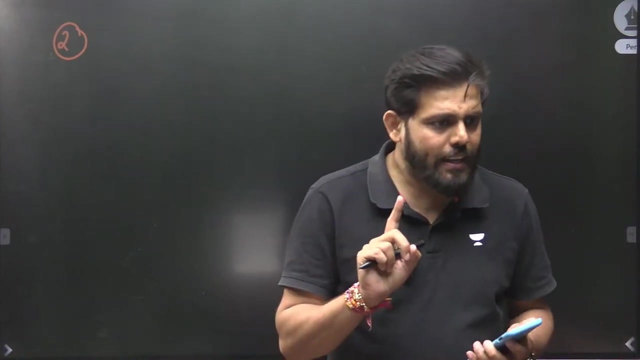 Okay, Is it clear? Now I will ask you One more concept. Now tell me One more concept, One more way The magnitude of high tide and low tide Can be changed. Is it clear? Okay, Now I will ask you One more condition: Got it? Does anyone have any problem? 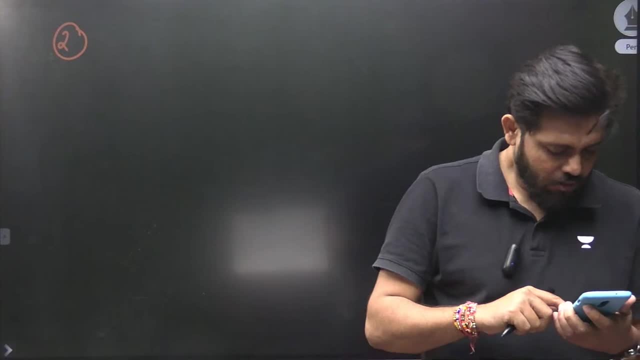 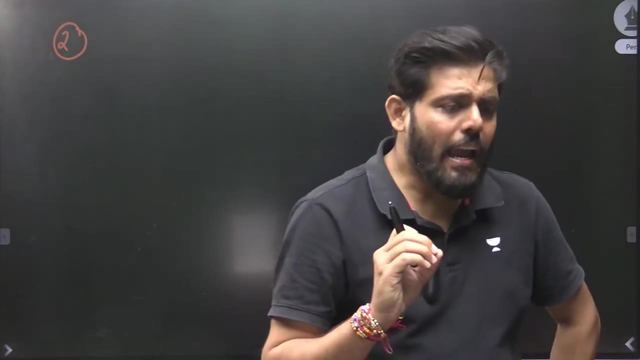 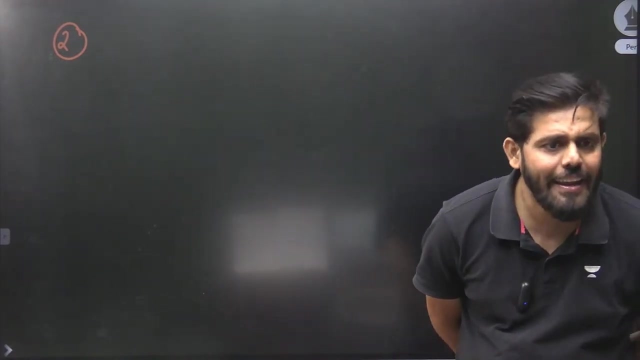 No, Like and share. Now I will ask one more question. Now tell me one more thing. Very good, Very good point And very good question. Now tell me one thing: What is the condition of Perihelion and epihelion? Tell me quickly, What is the condition of? 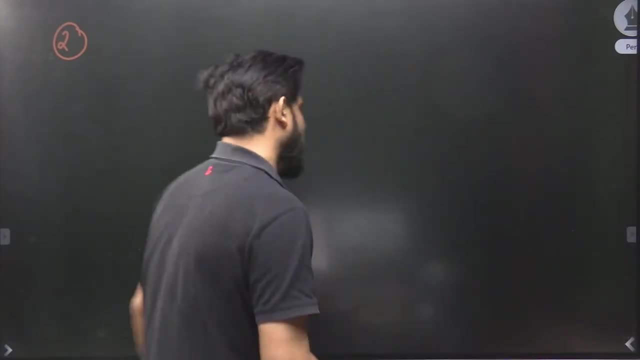 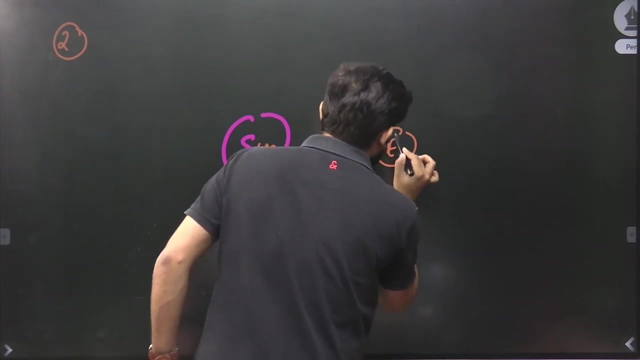 Perihelion and epihelion. What is the condition of perihelion and epihelion? Let's assume Here we have the sun And here we have the earth, And the earth is revolving around the sun In the elliptical orbit. 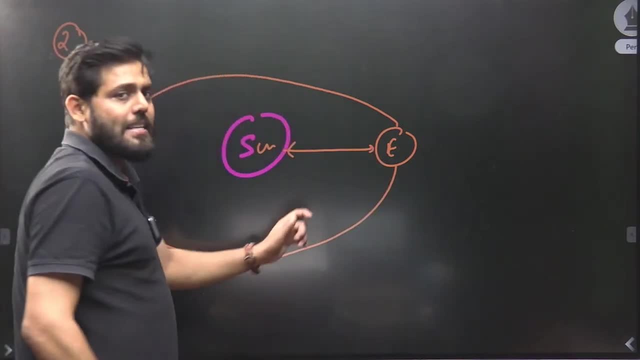 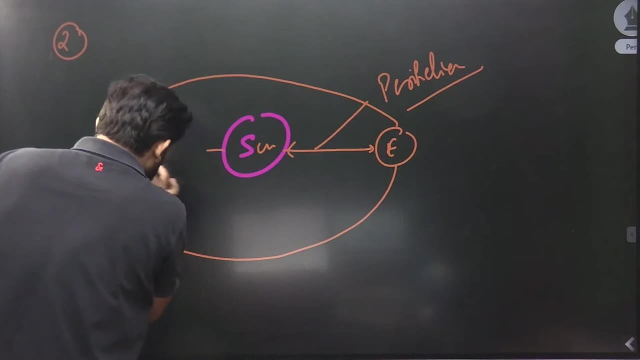 And when the distance Between sun and earth Will be the lowest, That is called perihelion, And when the distance Will be the highest, That is called epihelion. E, p, i, h e l i o n. Remember this. What is perihelion? And epihelion. What will we call perihelion? What will we call perihelion And what will we call Epihelion? This is epihelion. In epihelion, The highest distance is Between earth and sun, And perihelion has the lowest distance between Earth and Sun. 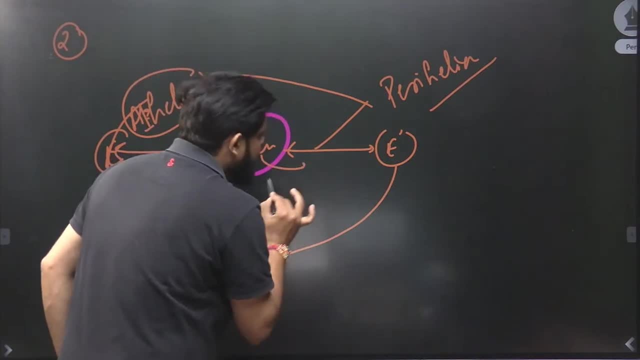 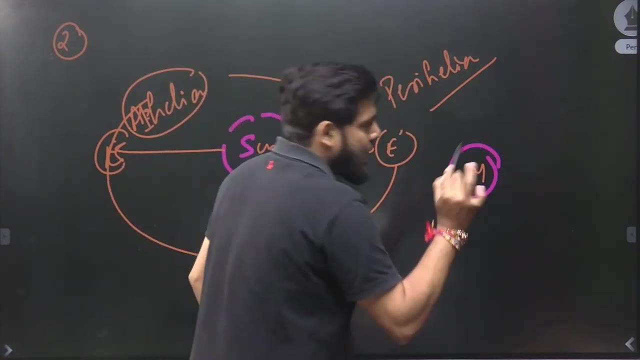 So when the distance is less, the gravitational force of the Sun will be more on Earth, Because the gravitational force of the Moon is strong, But the gravitational force of the Sun also seems to be some unit, So this passing will make it stronger. 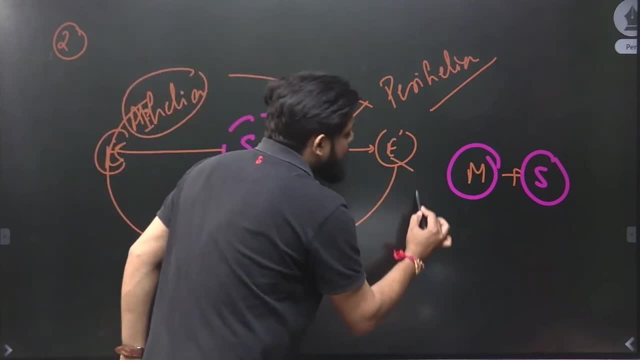 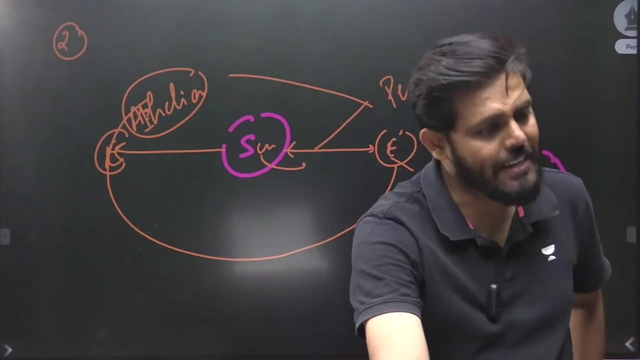 So at the time of perihelion the tides will be generally high and the average height will be generally high. So I have told you everything about when, how and what will be the condition. Tell me quickly How many students have understood everything. 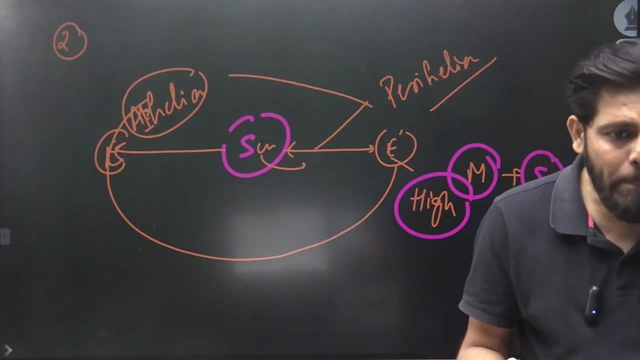 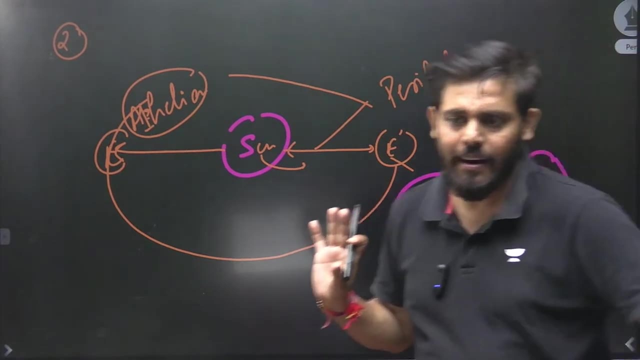 This is the point I told you. So you understood the concept of perihelion and epihelion. You also understood the condition of perzy and eposy. So you understood all these conditions. Is it clear? Is it clear? 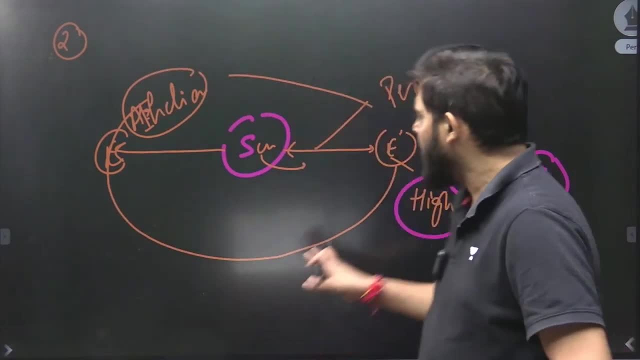 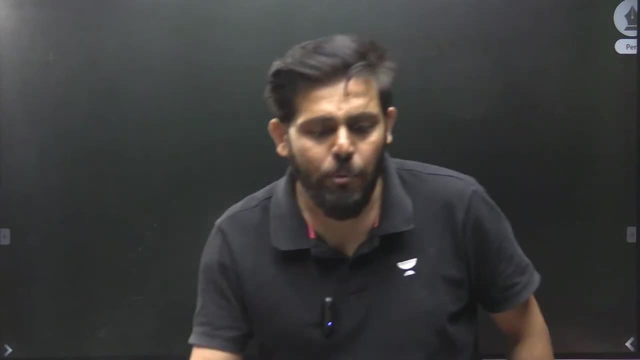 Does anyone have any problem? Each and everything is clear. Now I will tell you. I will bring one or two more points in front of you. Now I will bring a concept in front of you: Tidal bore. Who has heard about tidal bore? 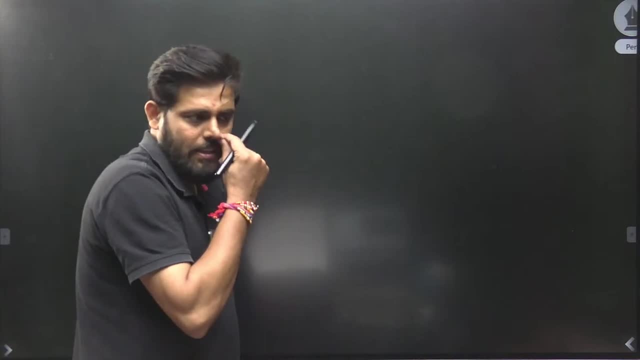 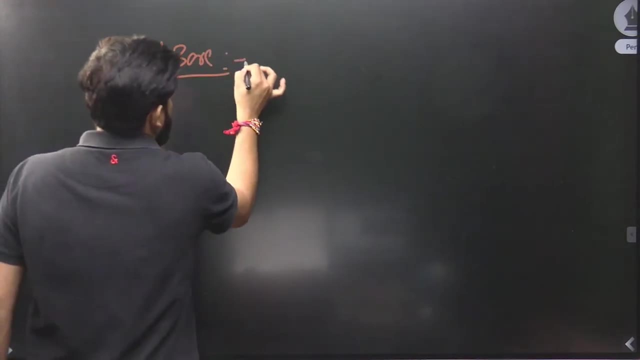 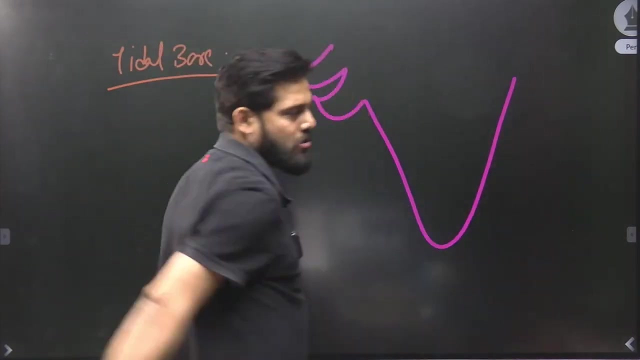 About tidal bore. Tell me quickly: What is tidal bore? Has anyone heard the concept of tidal bore Guys? what happens generally? Let's assume this is our coastal area. This is a coastal area. There is a river here. This river is coming. 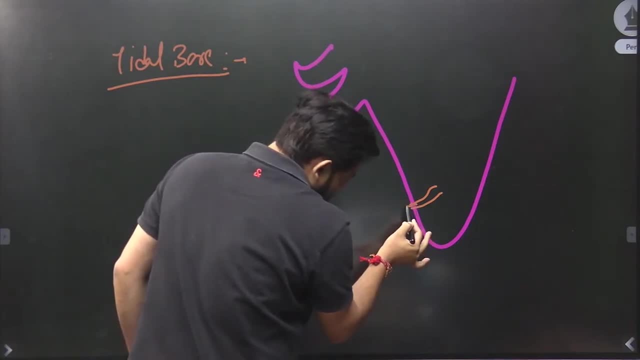 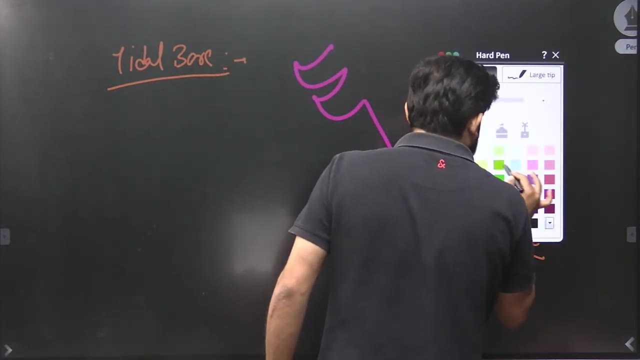 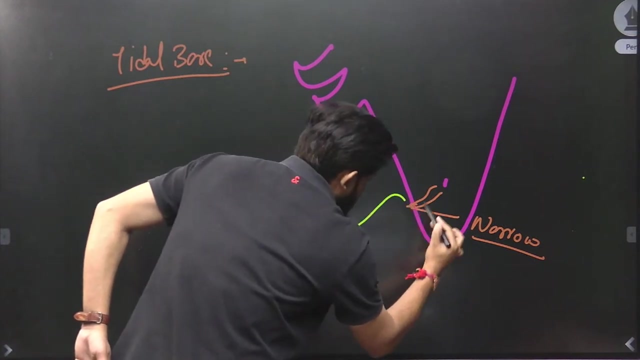 The inlet of this river is narrow. How is the outlet? It is narrow, Is it clear? So what happens When the outlet is narrow and this river is coming to the ocean and draining And suppose there is a high tide here? There is a high tide here. 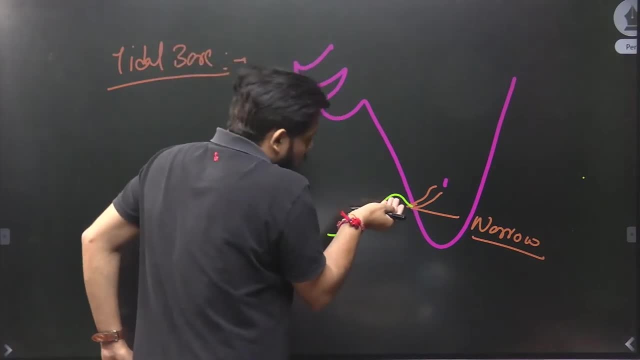 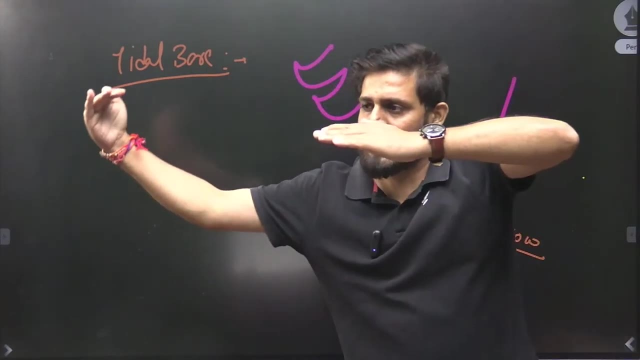 So what will this high tide do? Through this narrow inlet, the water will go back. This is the mouth of the river. The river is going to the ocean. The extra water of the high tide will go from the mouth of the river, from this outlet, to the inside of the river. 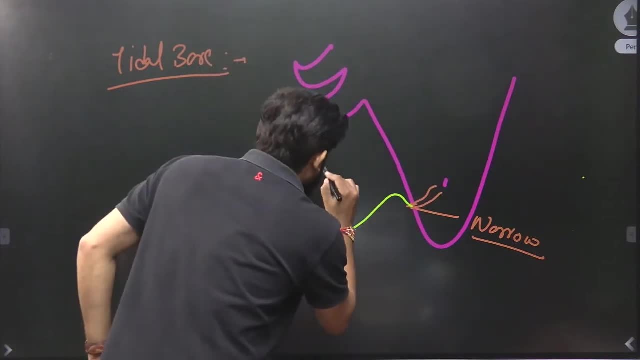 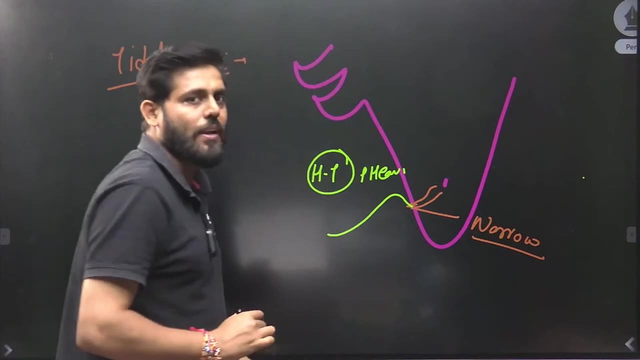 It will go to the inside of the river. Suppose our high tide has come here Now. along with the high tide, heavy rainfall is also happening. There is a high tide and heavy rainfall is happening, So what will the water of the high tide do? 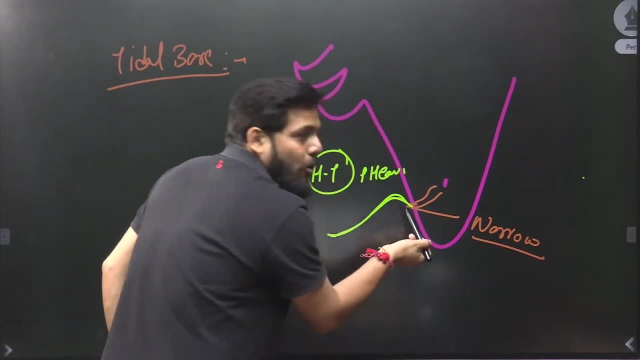 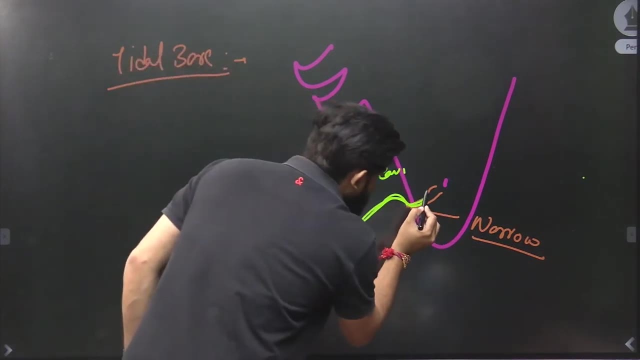 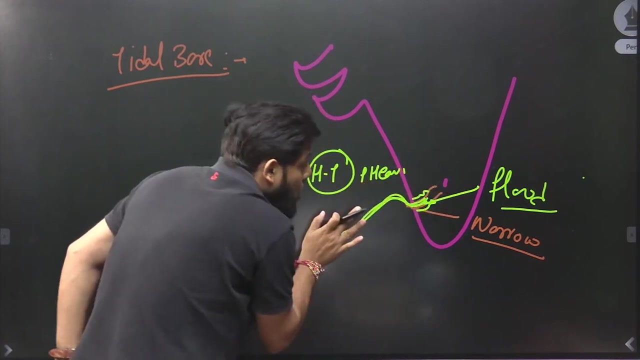 Through this outlet, through this narrow outlet, it will enter inside this river, And when it enters inside, then the surrounding area will be flooded. Why? Because the water level has increased due to the heavy rainfall and due to the high tide, And this condition is called tidal boom. 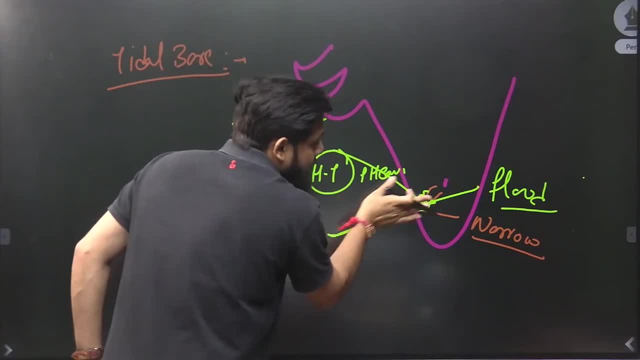 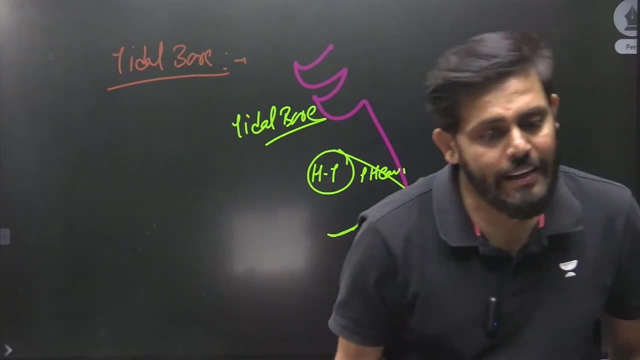 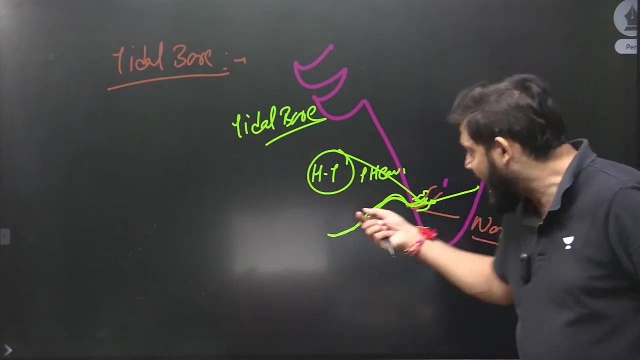 When the tide enters from the outlet to the inside, where the rivers are, and it floods the surrounding area. that condition is called tidal boom. Okay, A strong tide that pushes the river current River current Against. This is absolutely correct And this is the tidal bore. 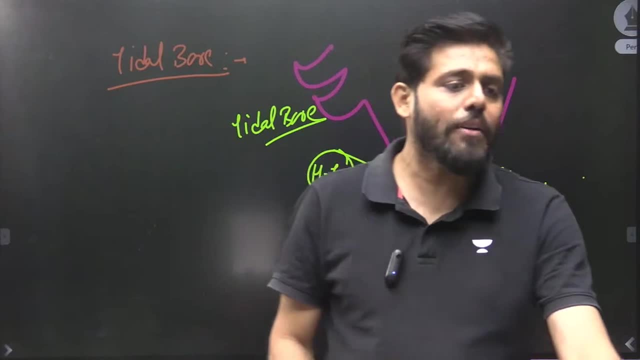 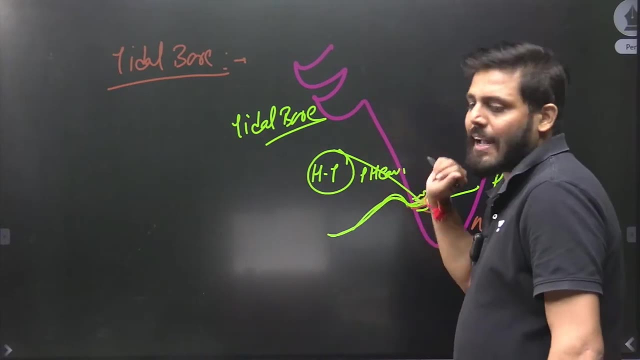 Did you understand? Anyone of you have any doubt regarding tidal bore Or in any concept, Anyone In any way? Fine, Now let's talk about the importance of these tides. We got to know about the high tide, semi-diurenal. 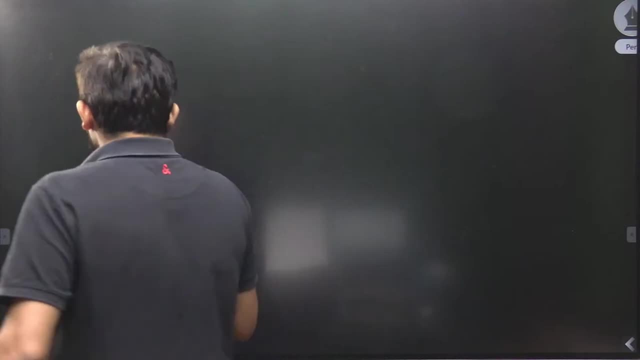 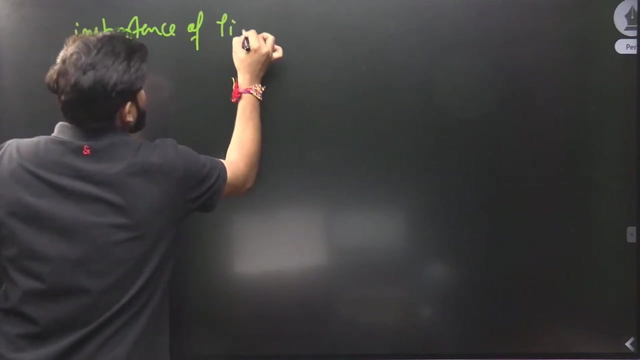 Everything happened very clearly in front of you. Now let's talk about the importance of tides. What is the importance of these tides? This is also very important. The most important thing is their fishing. It is very important for fishing. Why is it important? 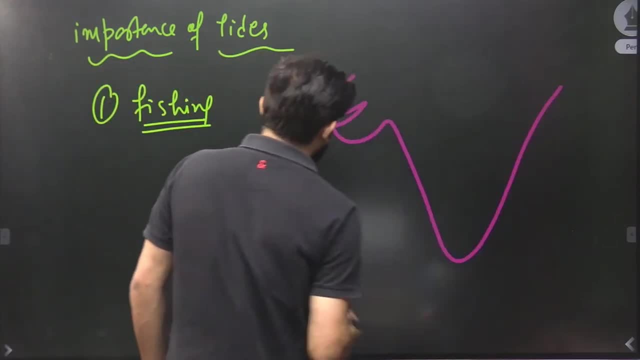 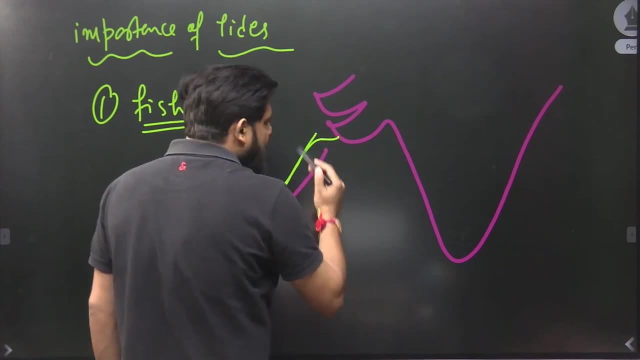 Let's assume that I have this coastal area here. Now, this coastal area, this high tide will come here. When this high tide comes here, then what will the tides bring with them? They will bring the fishes too, And where will the fishes come? 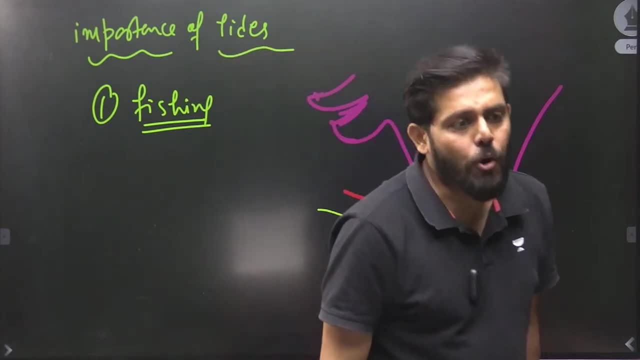 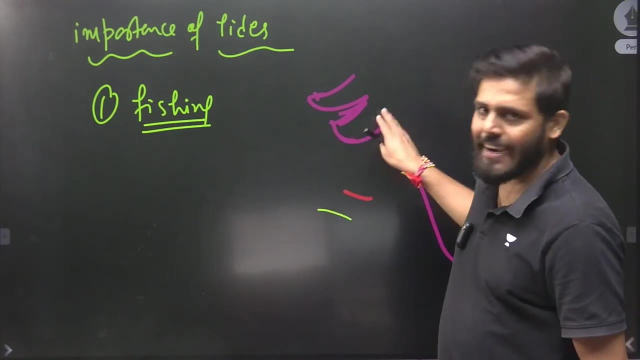 They will come to the coastal area, They will come to the continental shelf, And when they come to the continental shelf then our fishing industries will also be good here During the high tide. when the high tide comes, always remember they will go back to the low tide. 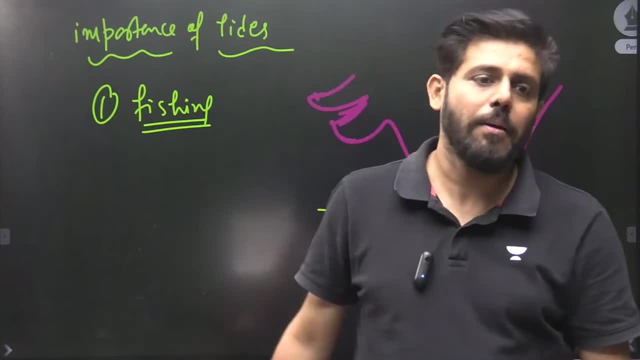 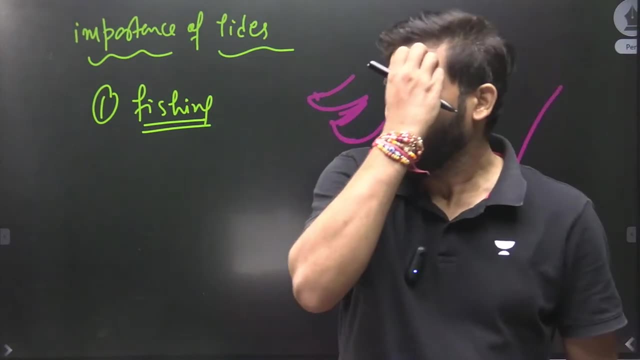 Always. another very important, very good concept. Tell me one thing: if you are standing in a coastal area, if you are standing in a coastal area of the sea, on the beach, then which tide is more dangerous for you? Which tide is more dangerous for you? 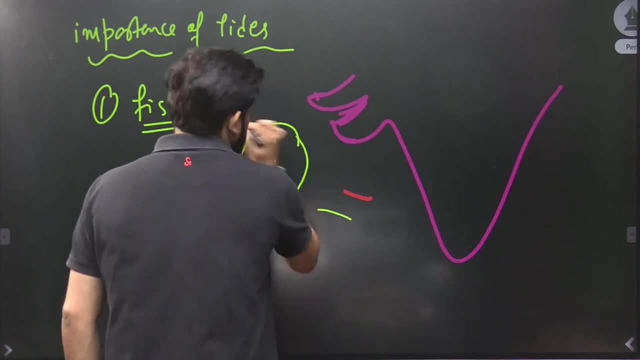 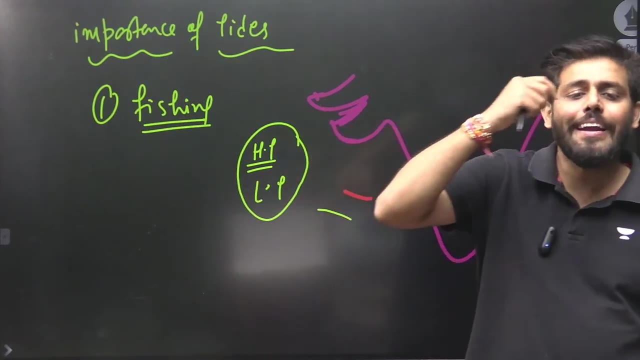 High tide or low tide? Tell me quickly If you are standing in a coastal area, if you are standing in a beach area, then for you high tide is more dangerous, for you or low tide? Tell me quickly Which one is more dangerous. 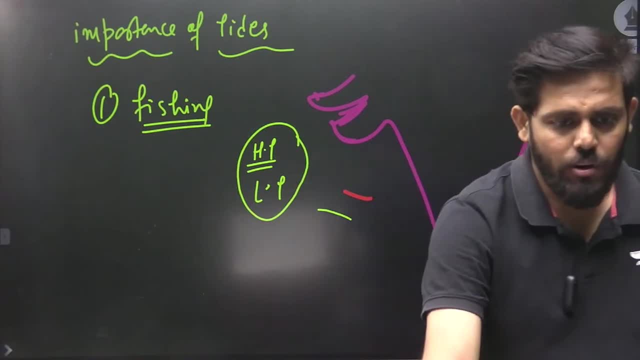 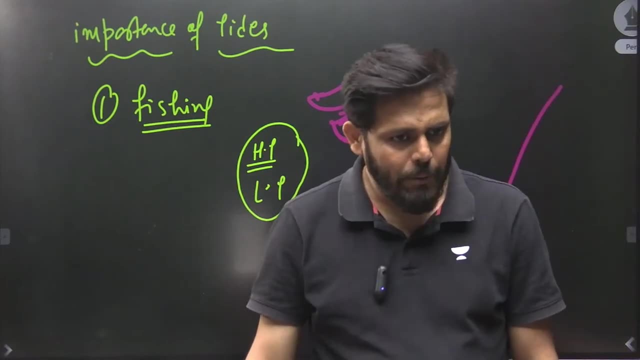 One student is saying: high tide, low tide, high tide, low tide. Tell me quickly which one is more dangerous for you. Some students are saying Parveen, high tide. Mauno, low tide. Avinash is point low. 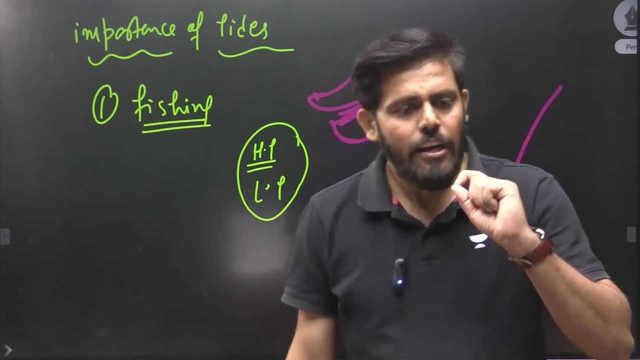 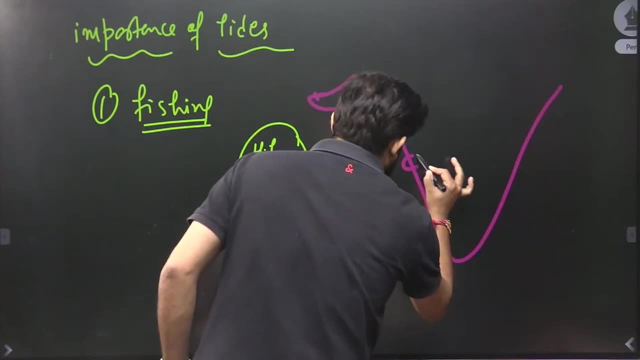 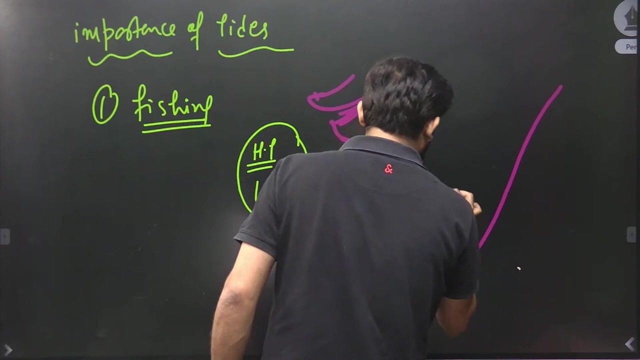 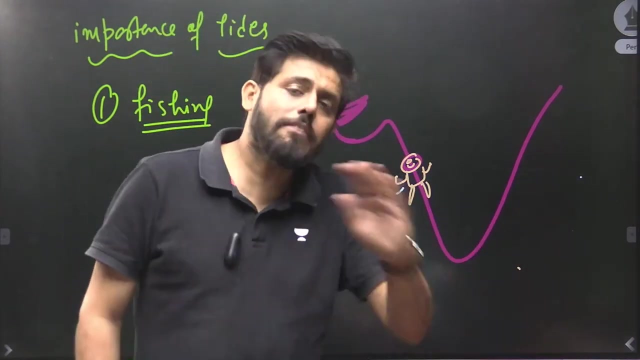 Avinash, low Abhishek is also low tide See, some high, some low See. Suppose you are standing here on this coastal area. try to understand: this is you. you are standing here perfectly, showing your body that nothing will happen to me. you are standing here suddenly. what happened? your high tide came here. what will this high tide do? this high tide will take you back, it will wash you away, but where? it will throw you out? towards the land, towards the inside. 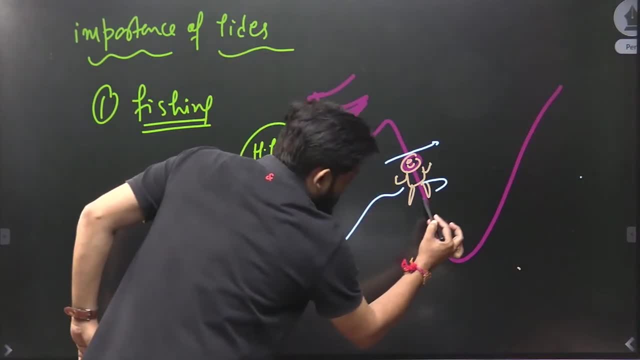 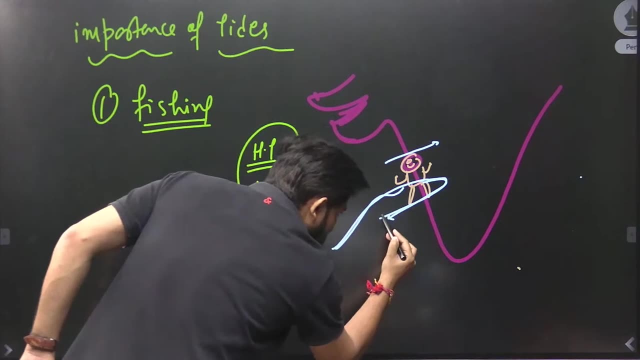 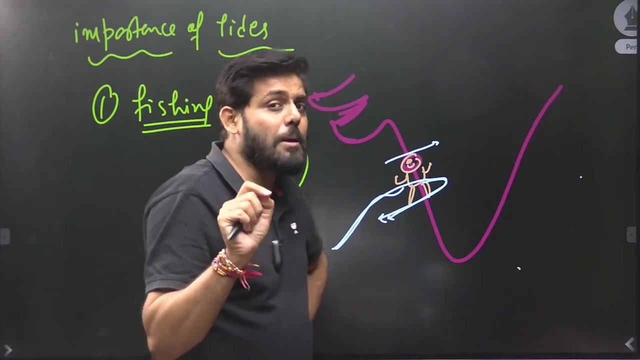 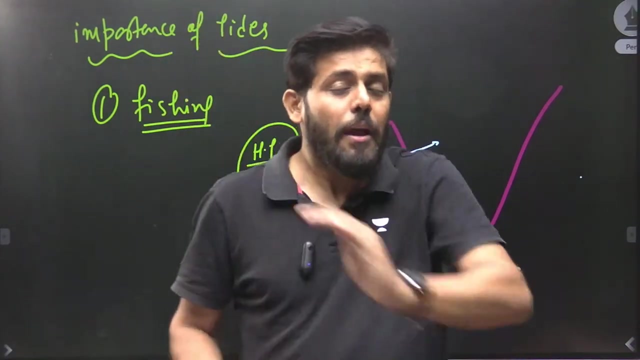 but the low tide goes back in this way. what does low tide do? it goes back. so when this high tide comes, then what does this low tide do? it takes you back into the ocean. so all the people who live in the coastal area, they always know that when there is a high tide it will throw you out towards the ocean, it will push you out towards the land, but when there is a low tide it goes back towards the ocean. 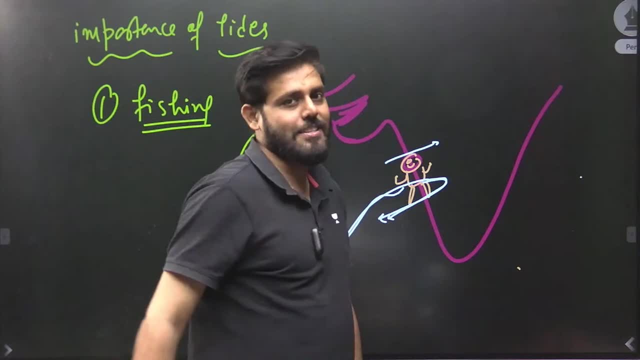 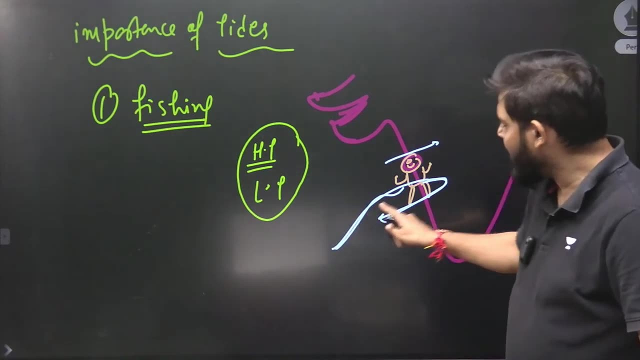 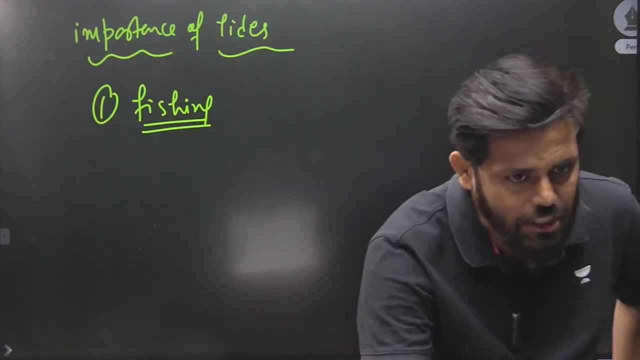 so it takes you with it to the ocean. so low tide is more dangerous. remember this thing, okay, it is clear. so always remember that low tide has more impact. so what did we talk about that? for our fishing, high tide is very good and tides are very beneficial for us. 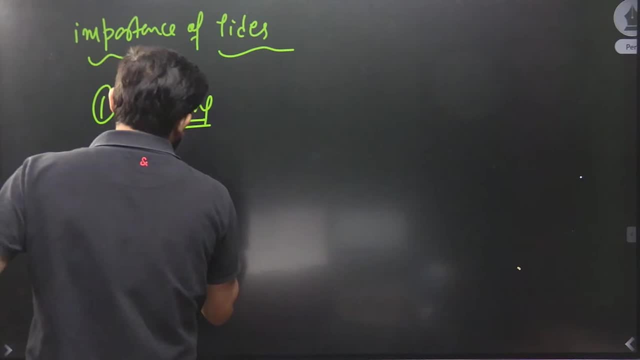 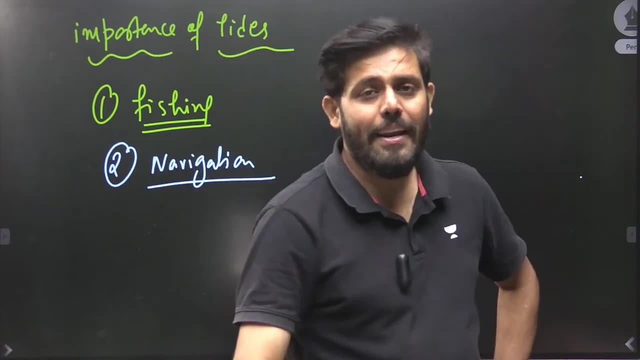 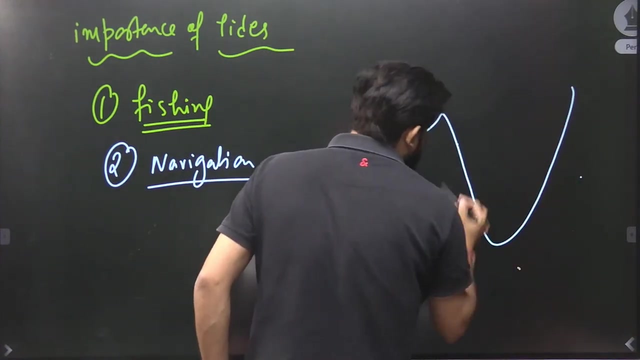 second is navigation. it is very important for navigation, especially if I talk about the shipping, which is very good for our boats, which is very good for our ships. so our first point to discuss is about the ports, and these are the ports. so what is there on these ports? how did our ship reach the ports? 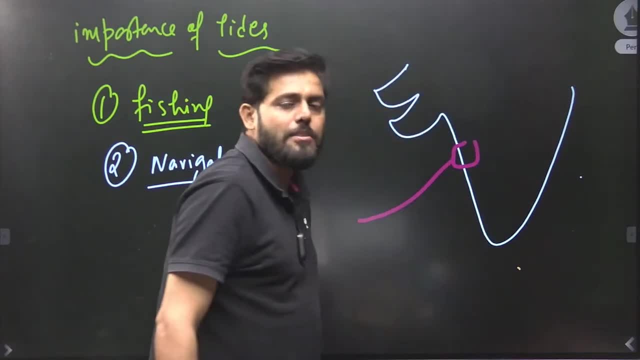 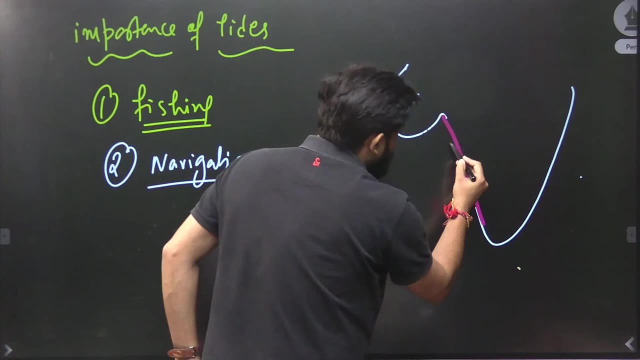 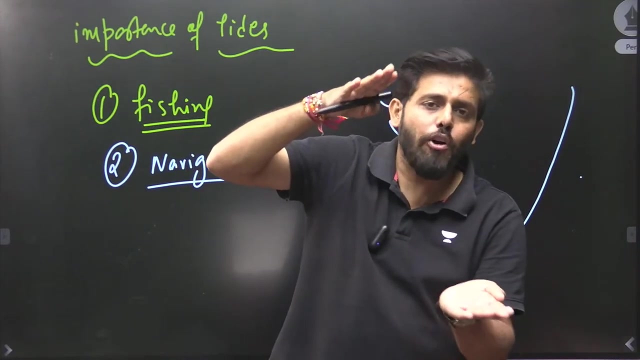 so what are we going to do? these high tides bring it with them, know that the harbors and the ships take it away from the ports. suppose there is a continental shelf at this point? at this point the continental shelf is very big, it is very wide, so the water level there will be shallow and the water level will be low. 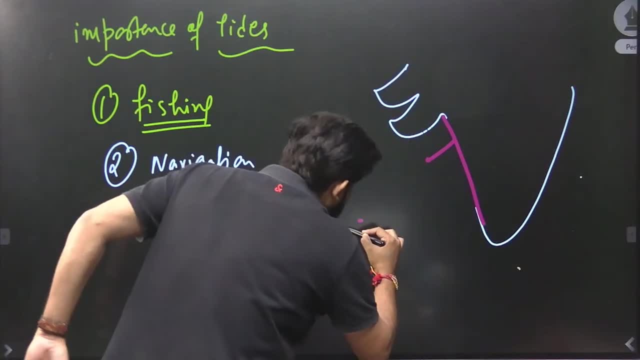 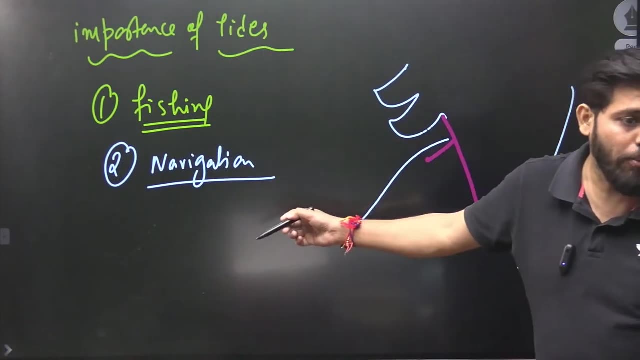 How will the ships come to the harbor? But what does this high tide do? It brings the water level due to which the ships go to the harbor, goes to the coastal area, goes to the port. So that means it is also very important for navigation. 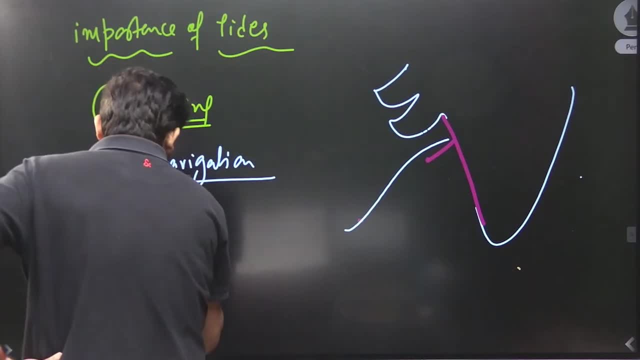 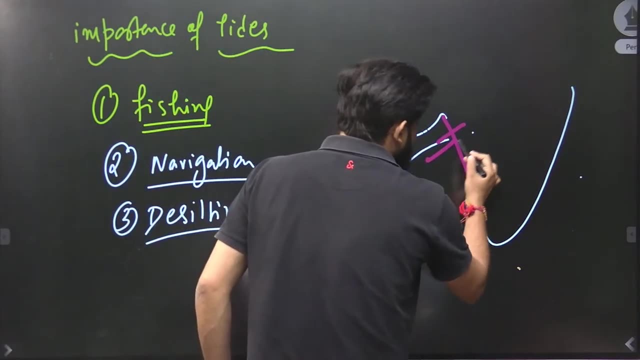 Along with that, desilting. desilting means the siltation that has happened here, at the ports, at the mouth of the rivers, near the rivers. sediments have happened here, so these high tides will come when the sediments go back with them. 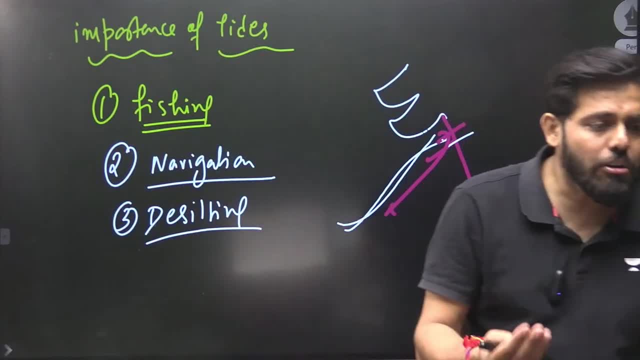 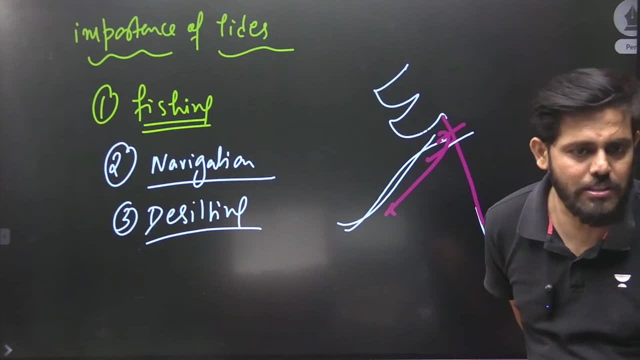 they will be washed away and taken away. So all the silt that has happened, all the sediments, the pollution here will be taken away. so these tides are also responsible for you And this is important to remember. So desilting plays a role in navigation. 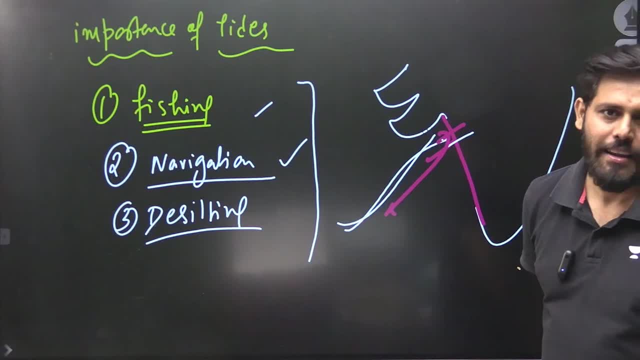 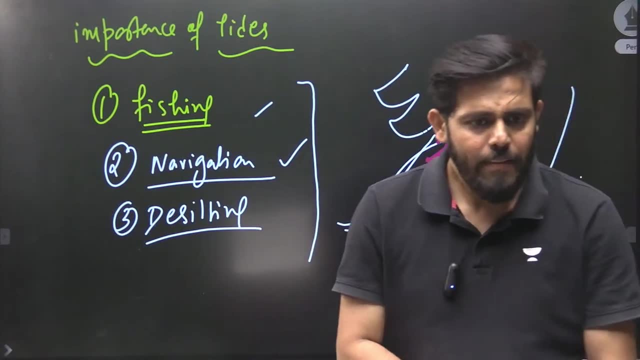 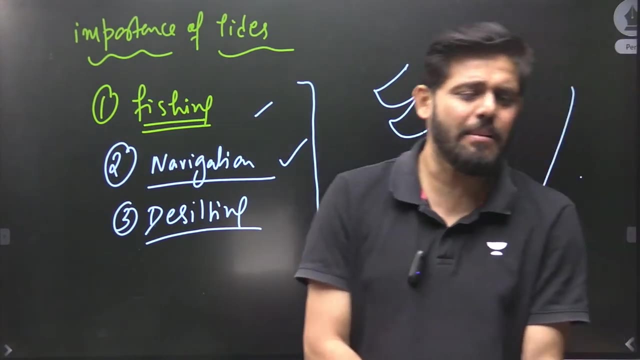 Our tides are very important for the fishing industries. So this is all about the tides. We covered the tides very well. We tried to understand. the title bore: Okay, Krishna, please be quiet, Don't make unnecessary disturbances, Okay. 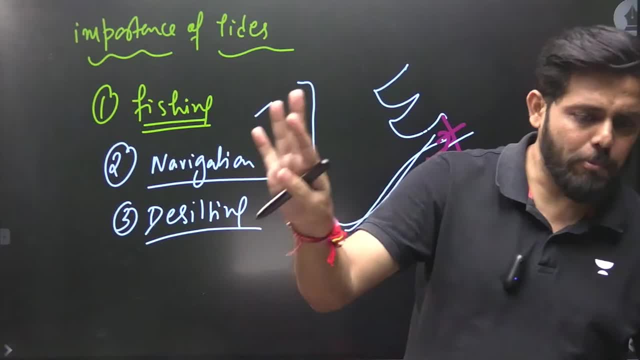 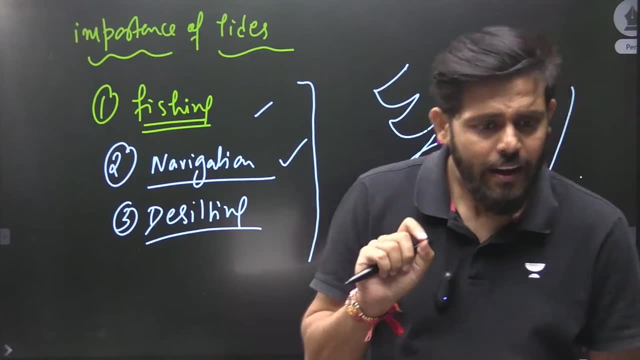 Then you will get blocked. You can ask whatever you want later. Don't do it now. Let the students who have doubts come. Okay, So now tell me any student up to here: hydroelectric power station is absolutely right. Our title is very important for the title: energy. 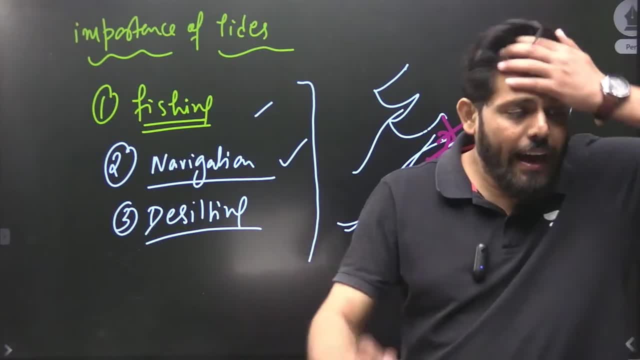 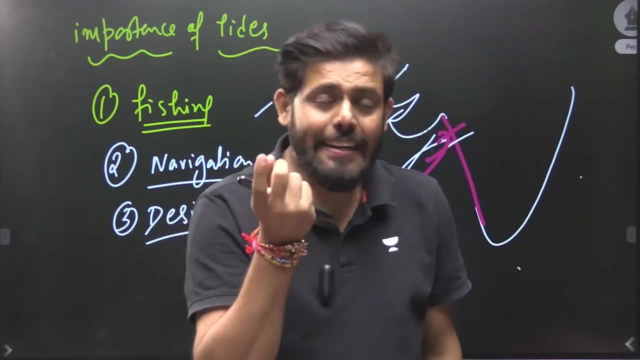 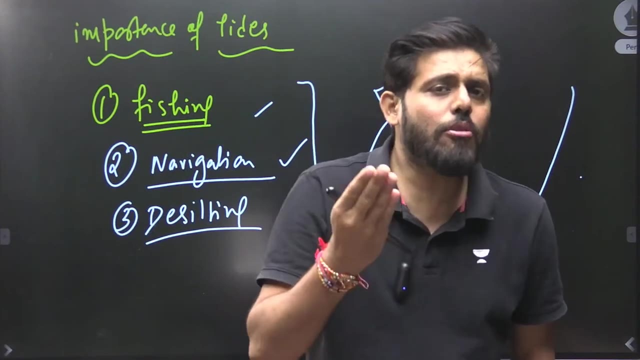 Is it clear? Any student up to here has any problem in any way For the mangroves. See. tides are not important for the mangroves, But the erosion caused by the tides, the coastal erosion, the mangroves protect from it. 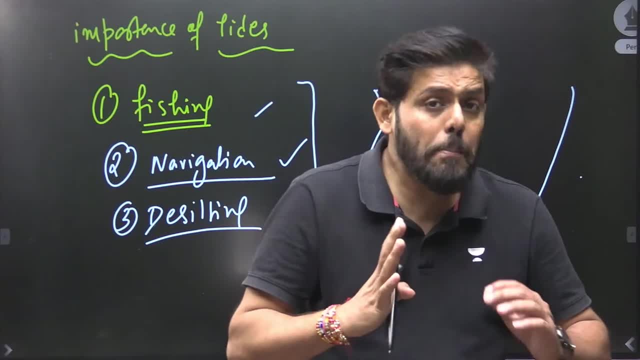 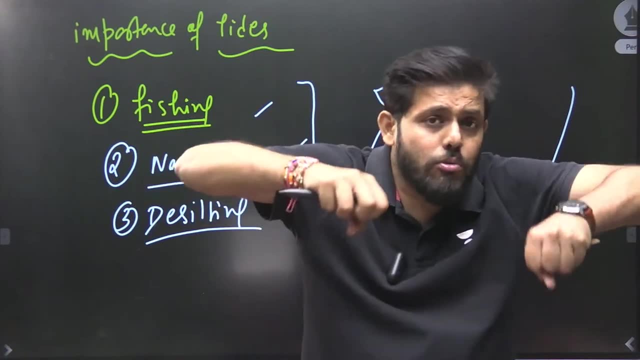 The mangroves, the destruction they protect, Because the roots of the mangroves are very big And they come out of the water too. And those roots which are on the coastal area, the sediments and sand on the coastal area. 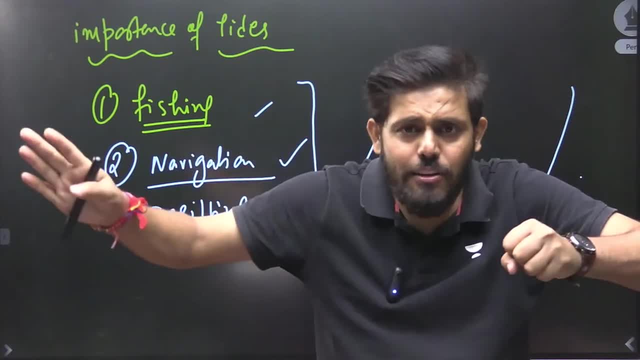 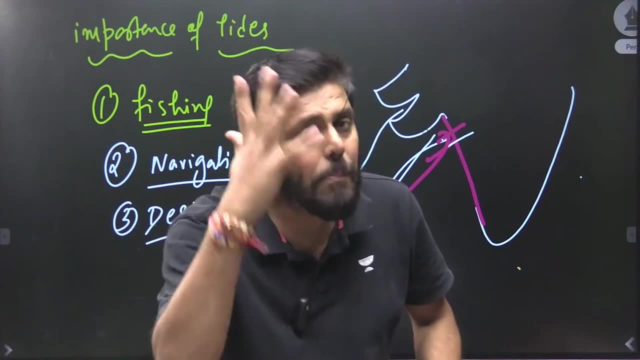 they bind them with each other, Due to which the tides which erode them. when tides and waves come, they erode them, So the impact of that that mangrove reduces. Tomorrow I will teach you the waves. Don't miss tomorrow's session. 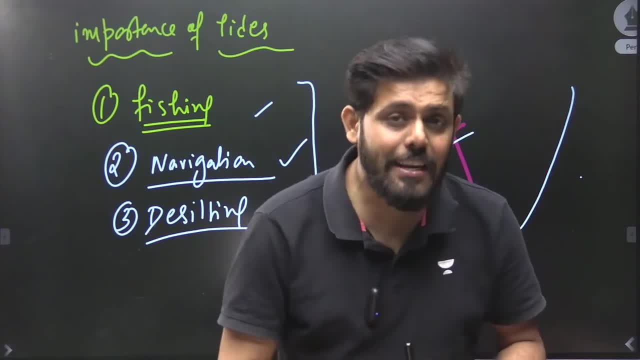 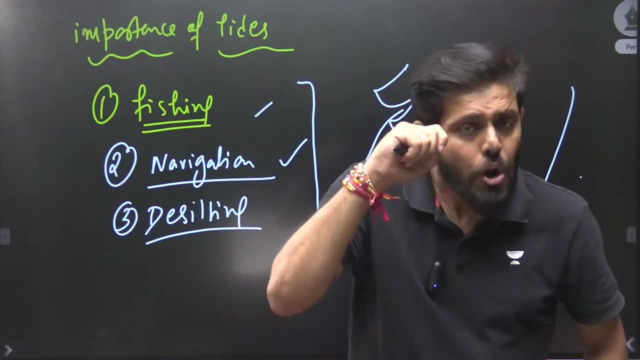 How does the tsunami come tomorrow? What is the reason? What is the wavelength in it? How does it oscillate? We will cover all these things in tomorrow's class In the ocean wave, Which is very important. Okay, Is it clear? 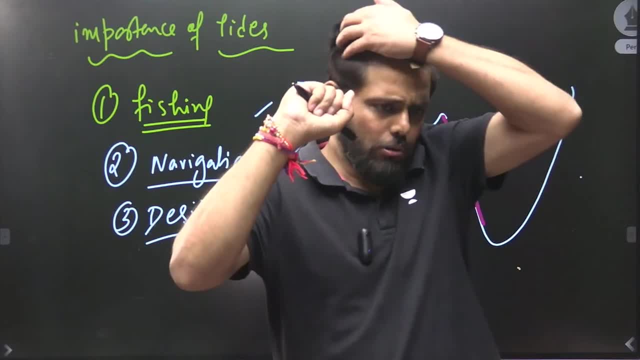 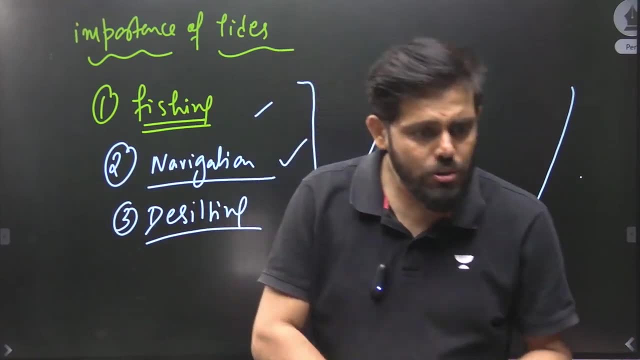 We will study it tomorrow. Okay, Ocean waves. So all the students do like and share it once. Follow Here. I have told the things very tightly. I will talk more about oceans and waves. What are all the things? How are they? 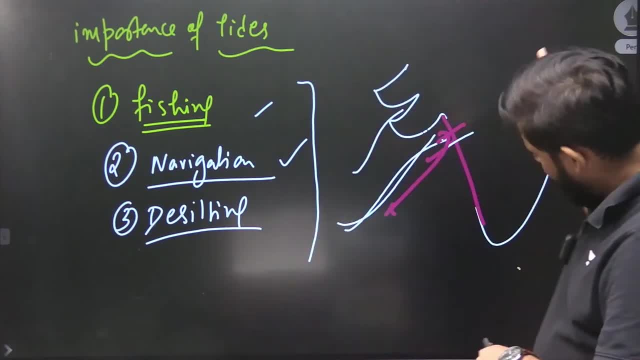 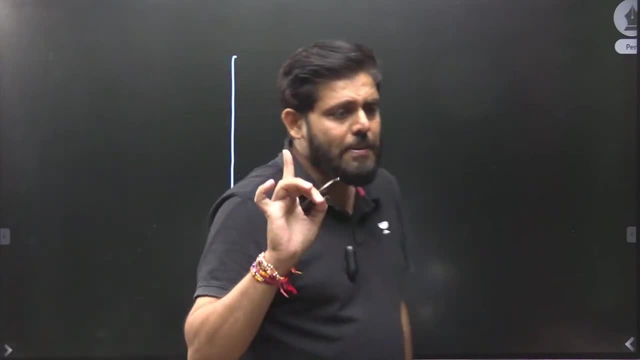 I will cover all those things for you. I will give all the updates: Which book to read, How to read. We will discuss all the things Quickly. first of all, all the students. my telegram channel is unacademy- underscore- andrudmalik. 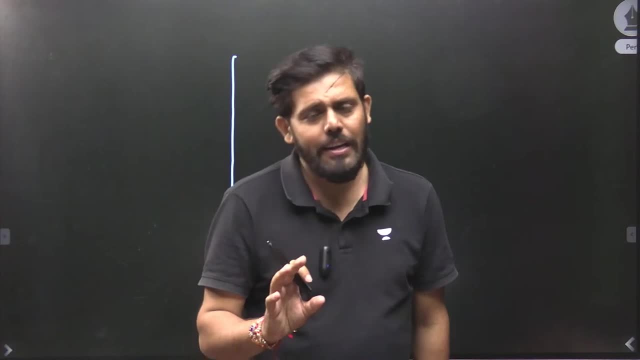 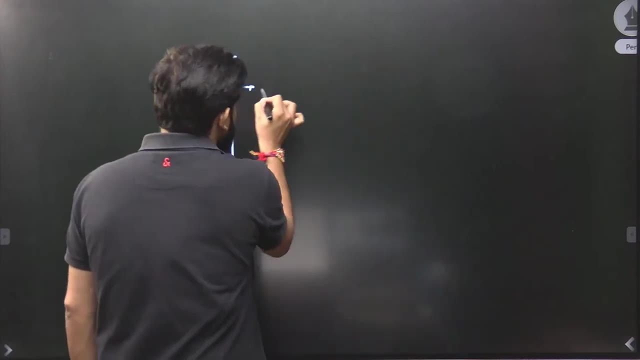 unacademy. underscore: andrudmalik: Do follow it, Do join it. All the notifications, all the updates you will get there, Along with that guys, very soon. next month I am starting NCRT, And with a lot of quality. 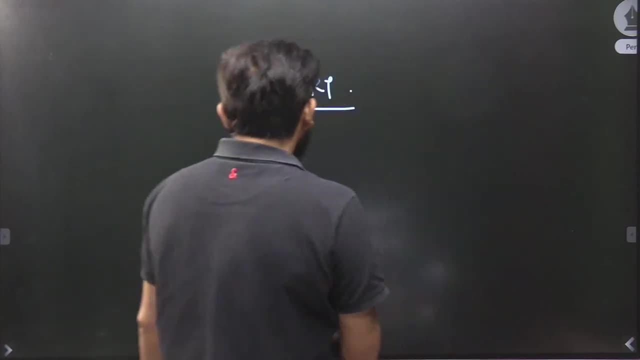 I am going to cover this NCRT Along with that. most importantly, I will start environment Environment And I will cover it in a lot of detail: Environment And this environment. I will cover it for you from next month. The classes of environment. 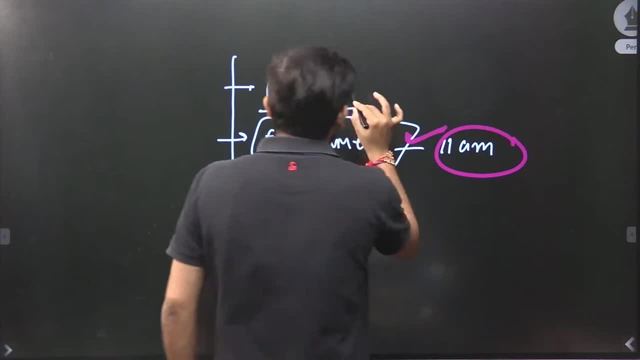 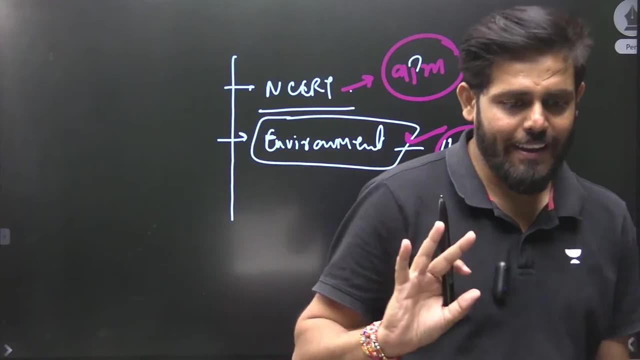 will be from 11 am in the morning And there NCRT will be from 9 pm in October. October month for you Means it is a seed for you, Is it clear? Very nice, Is it clear? Along with that, 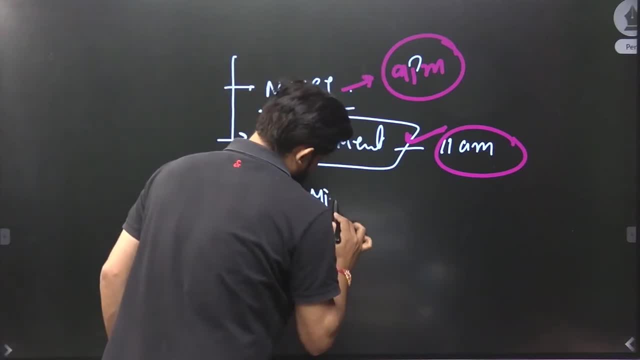 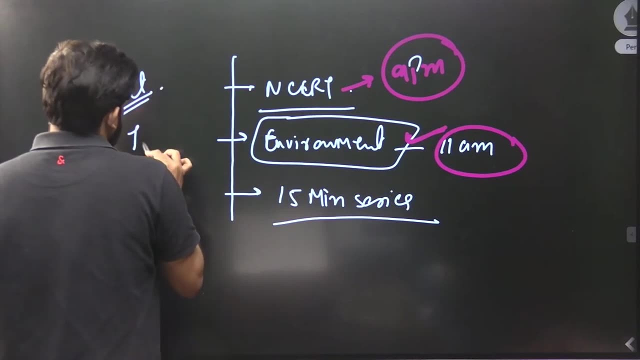 I will bring you a 15-minute series. I will bring a 15-minute series, And in October I am getting a new batch of Indian geography, So you can join that too, And it is a fresh batch With quality content.